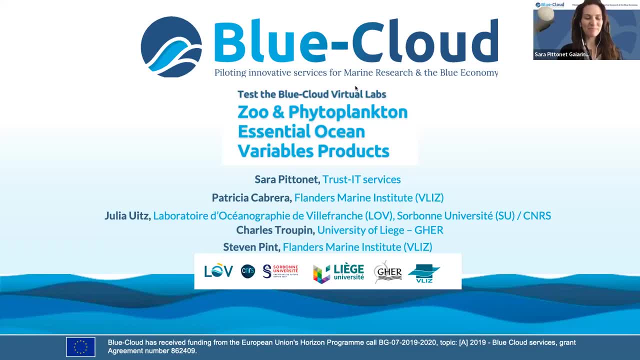 Welcome again to this webinar. We will have a question and answer session at the end, but feel free to use the question and answer box, the feature on Zoom, to ask any questions while our experts are presenting. So again, welcome everybody. I know we have some renowned members of the Blue Cloud community, but I also see some newcomers to this webinar. 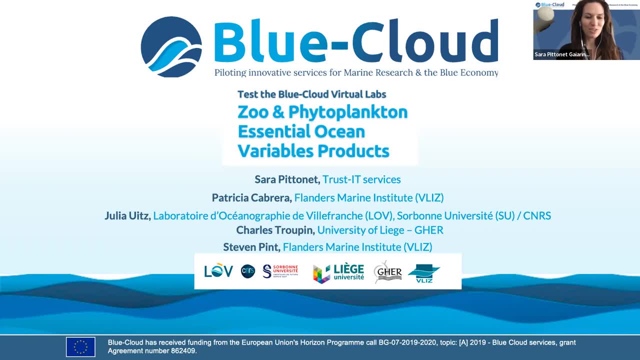 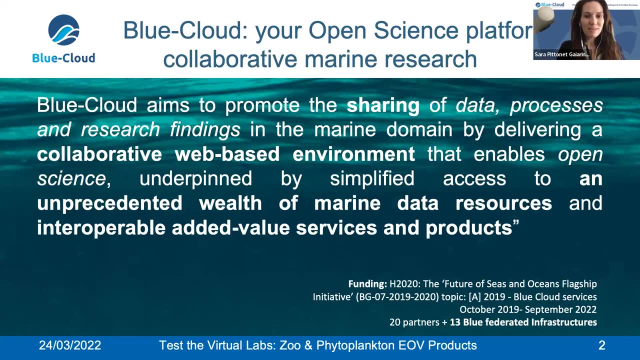 And so I'm very pleased, as Blue Cloud coordinator, to just give you a brief introduction again about Blue Cloud that we like to call your open science platform for collaborative marine research. So Blue Cloud is the Future of the Seas and Oceans flagship initiative. 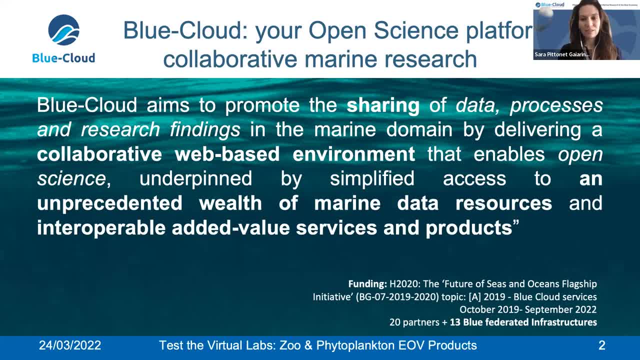 It's a part of the European Union Horizon 2020 program and it's the thematic open science cloud for the marine domain. It aims to promote the sharing of data processes and research findings by delivering a collaborative web-based environment that allows you to access an unprecedented amount of marine data resources, as well as interoperable 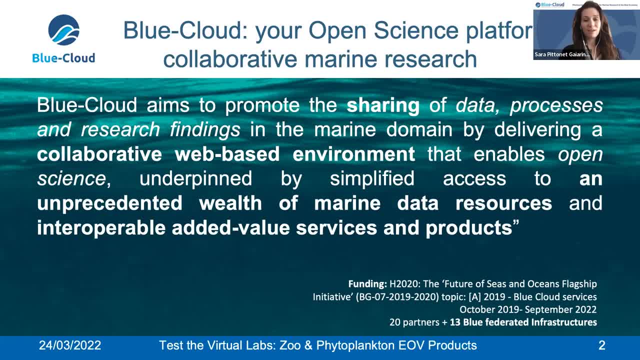 buildings, services and products that will allow you and other researchers to perform research, we hope, in a better way. The project started in 2019 and features 20 partners across Europe, but what's the strategic in the Blue Cloud framework is that Blue Cloud is federating European Horizontal Infrastructures, such as viruses. 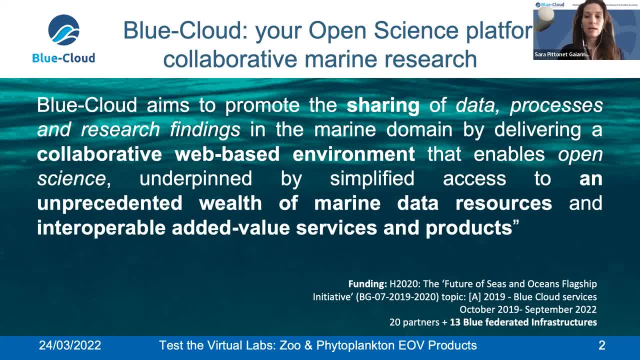 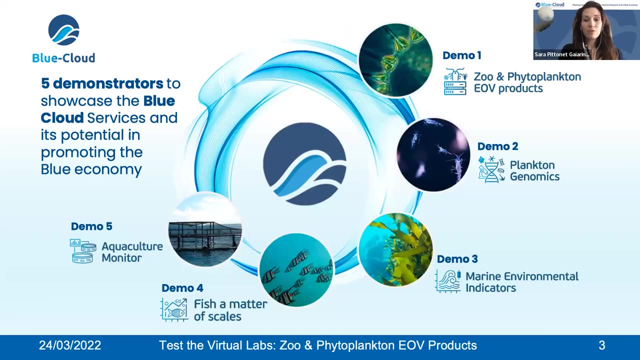 such as with 13 blue data infrastructures, and together they create this virtual space where you can access all together data, tools and services to perform your research in a more efficient way. Five virtual labs are developed as real life demonstrators, making use of the data and the 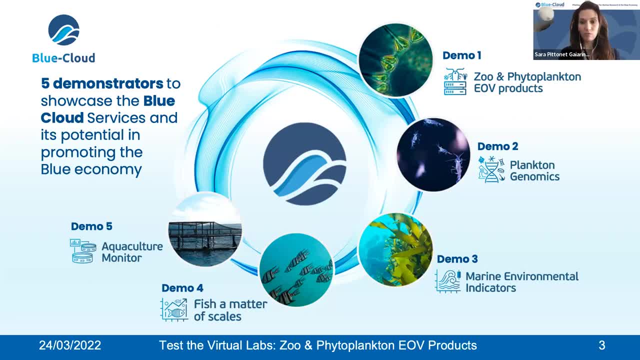 services available in the blue cloud virtual research environment and they address specific challenges in biodiversity, genomics, environment, fisheries and aquaculture domains. and today we'll be very happy to hear the novelties of the virtual lab dedicated to zoa and phytoplankton, essential. 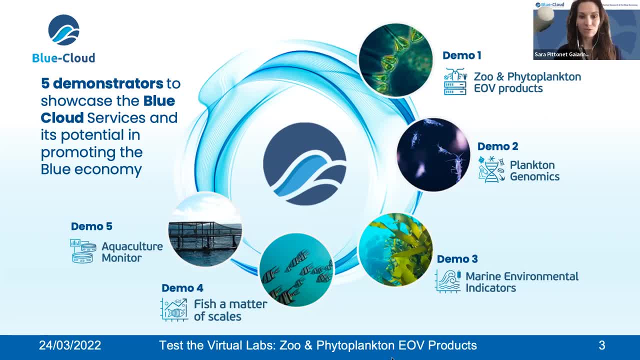 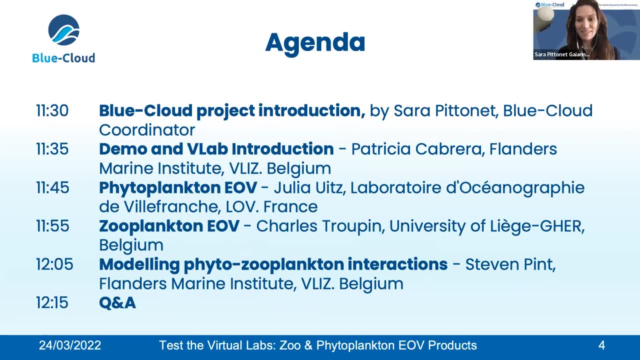 ocean variable products, which we call demonstrator number one. So what will you learn today? First of all, you'll learn why plankton is important in the function involved coastal and open oceans ecosystems, and why understanding the changes in across time and geography of plankton is important to understand the health of our ecosystems and, in general, the responses. 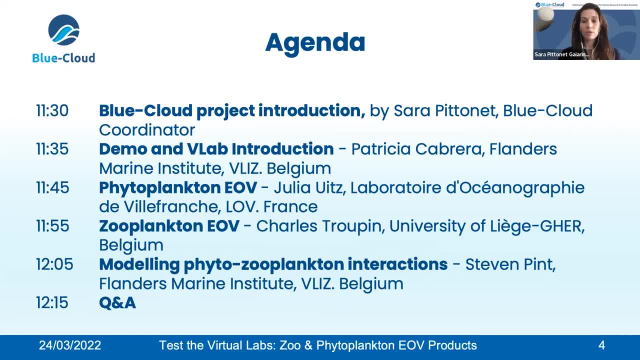 to climate change. Then you'll learn more about the zoa and phytoplankton essential ocean variable products demonstrator, where you can find three different products that will allow researchers to generate 3D vertical distribution of chlorophyll concentrations, to generate zooplankton distribution maps over a period of time and spatial areas, and also to run. 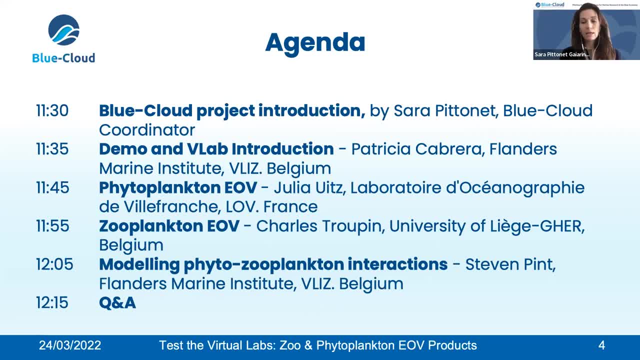 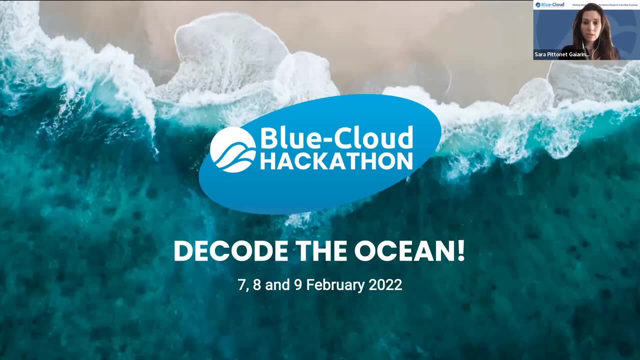 a modeling service that helps understand how photon zooplankton production changes across time and space in the ocean. So last month, so between the 7th and 9th of February 2022, Blue Cloud run its first hackathon. It was open to marine researchers, data scientists, ICT experts. 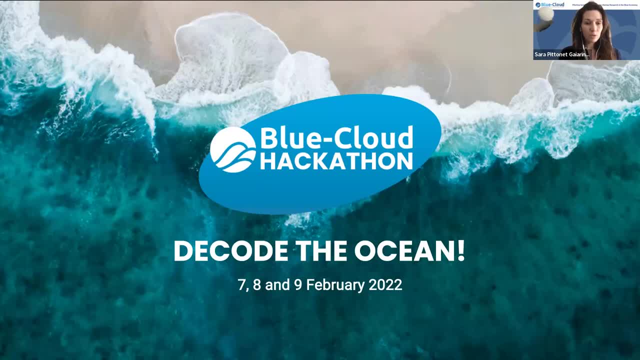 innovators and students to test the Blue Cloud virtual research environments and virtual labs and the services and products that are available there. So we had almost 150 participants, the first of which were from 39 countries, of which 20 European countries. We were very proud. 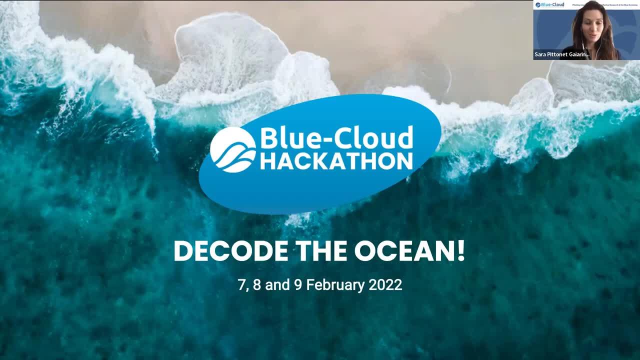 of the feedback received by these end users, and now I like to say that it's your turn. so we hope that this webinar will entice your curiosity and your interest in the virtual labs and will help you ask us questions and have your try within Blue Cloud's environment. 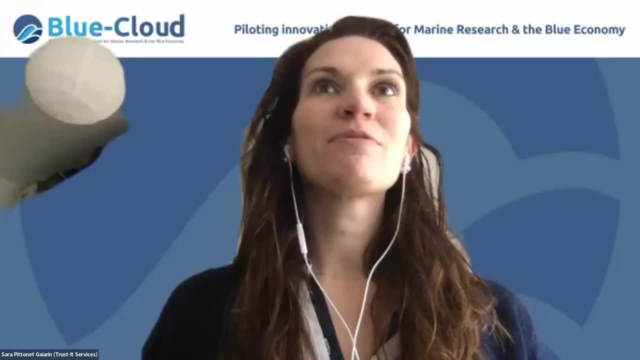 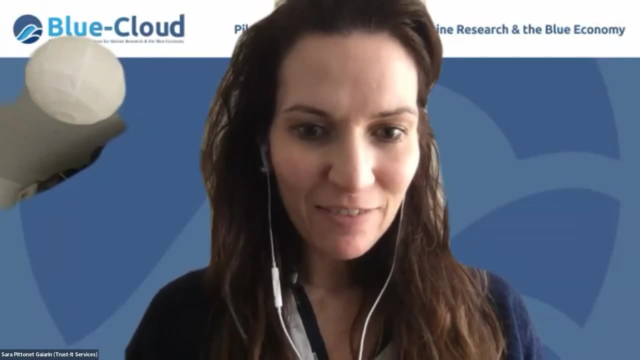 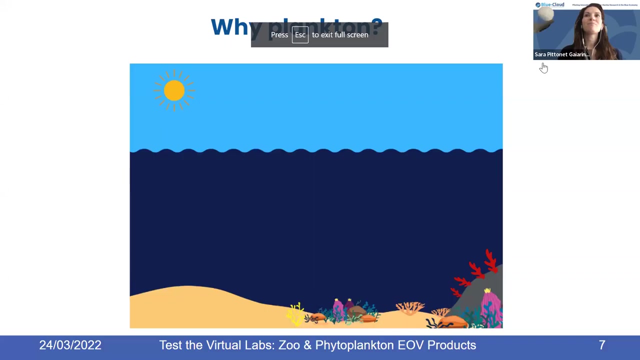 With that now I'm happy to leave the floor to back to Patricia. So yeah, I think you can share this screen. So Patricia is from the Flanders Research Marine Institute in Belgium, Leeds, and she's one of the leading partners of the zooplankton demonstrator. 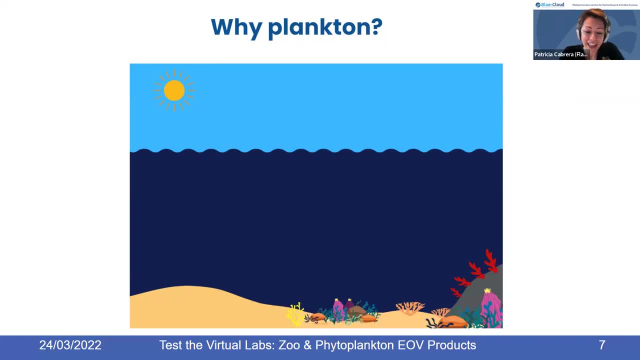 Thank you. Thank you, Sarah. So yeah, I was leading a team of researchers that develop this work. So before they explain us in detail how they develop the methods and the results, I will just quickly explain why we are studying plankton and also some basic information about. 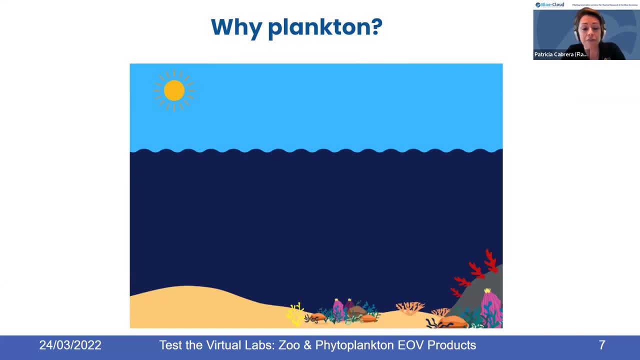 how to enter in the vLab and where is everything in the virtual lab. So, as you all may know, they are very little, tiny creatures that are in the ocean and they are very important because they are the foundation of many of the marine traffic webs in the ocean. 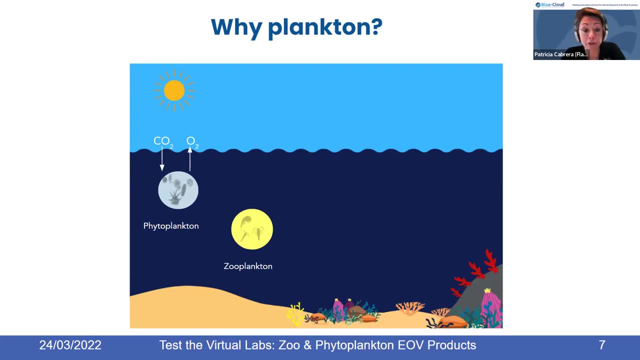 So they have also a great contribution in biogeochemical cycles in the ocean, like, for instance: phytoplankton do contribute for approximately 50 percent of the global earth photosynthesis by capturing CO2 from the atmosphere and releasing oxygen, and as well a phytoplankton and zooplankton do contribute to the biological carbon pump. 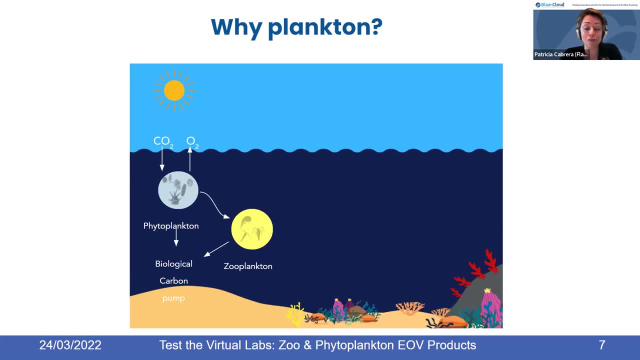 so zooplankton feeds on phytoplankton, and both serve as the basis of the higher species in the trophic webs, like sea turtles, jellyfish, fishes and up to the human. as that, we depend on the ecosystem services that the ocean is providing to us. 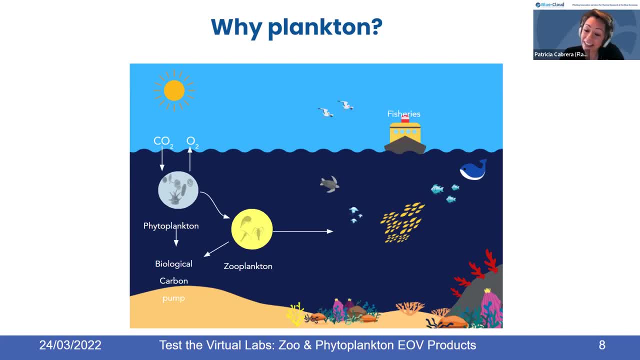 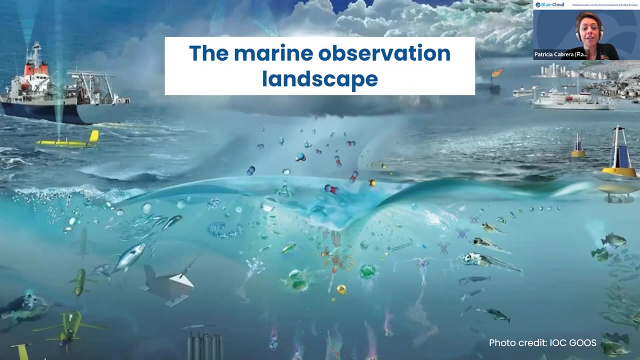 but what can happen if these little creatures disappear in the ocean? so the whole ecosystem can collapse, and therefore that's why we need to study them and understand how are the changes will affect in the future to the ecosystem, and so for this, there is a lot of ways to to study plankton and, in general, the the whole ecosystem. 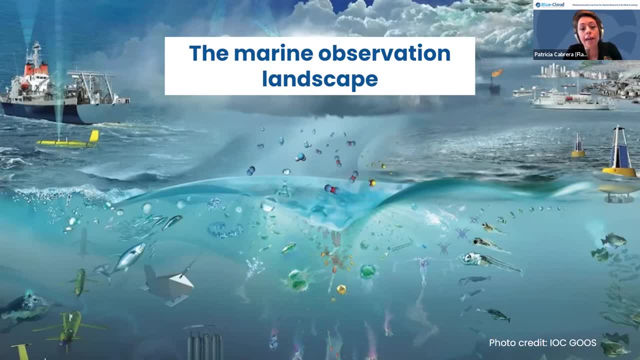 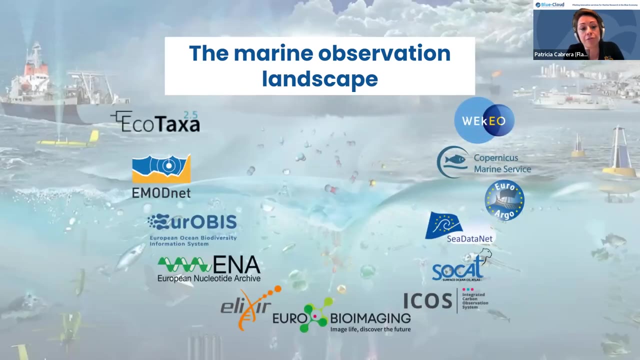 and as we are advancing in technologies, there is a much more, a different way how we are taking these observations. it is faster and we're taking much more data. and all this data it is scattered through a lot of different data infrastructures which you, you, the is the reason why blue cloud comes, comes into into play to really federate all these data. 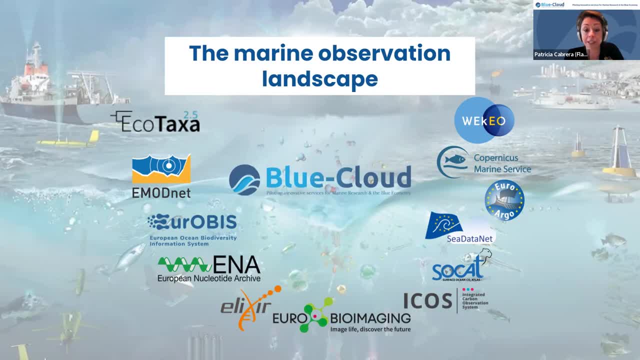 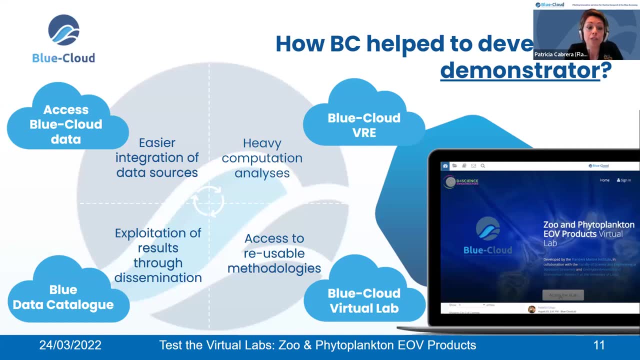 infrastructures, but as well to provide many other services that have helped us to develop this, this demonstrator, and how this happened. so, uh, through the access, data access and service to all these data infrastructures i just showed, uh we were able to have, uh, there is, uh is a lot of data, and 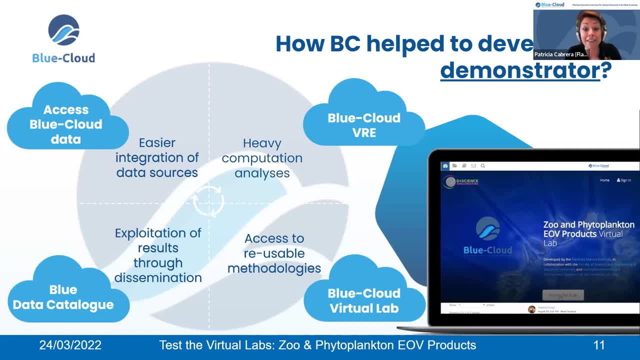 and we have been releasing data for the last, though ccc modern conjures for this project, undoubtedly the latest limits. payoff is very small, like i said, and in this project, uh, we ourselves remember well that this- uh, there is soon to be some very low compute processes. so my 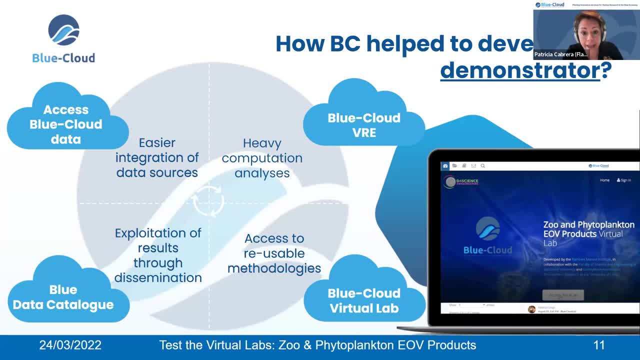 experience has telling us that the working environment, which Philipp some of the products that are i just mentioned, for instance, as vitamin fuel, as i said, had to have some happen And there we are able to have to work collaboratively between everyone, with all this different data and using all the services. 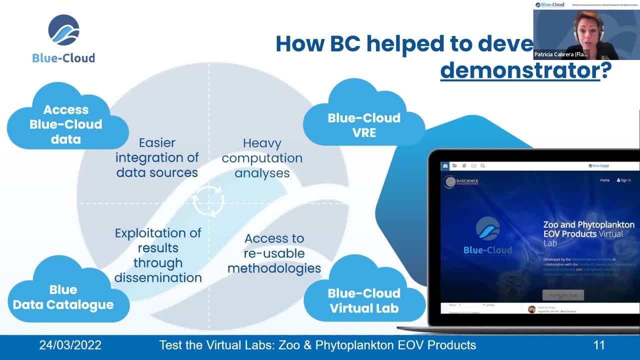 And finally, we can also exploit these results. such it was done in the hackathon, Or we're hoping that with these webinars people get to know more this demonstrator and can jump in and use it, as well as publishing this through the Blue Data Catalog. 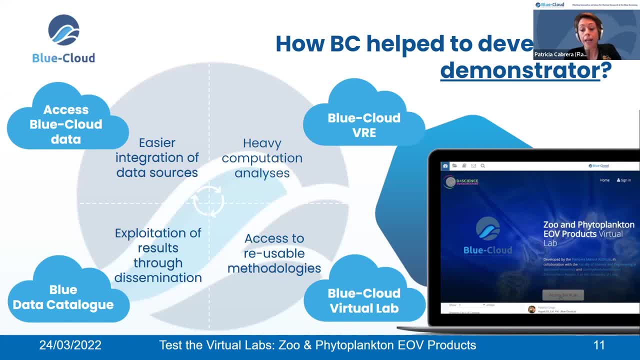 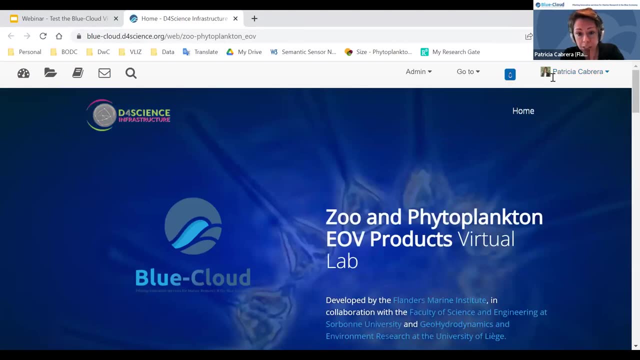 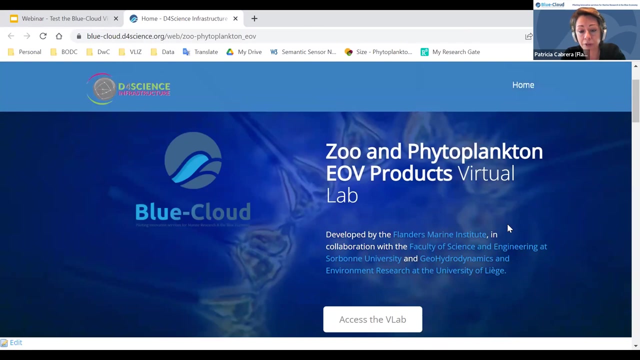 And also Zenodo and EOSC catalog. So those are more or less in a nutshell. what are the services in Blue Cloud? and I will just quickly jump into the homepage. And so, as you can see here in the bluecloudorg web page is where you can find the access to the VLAB, for example, and there normally. 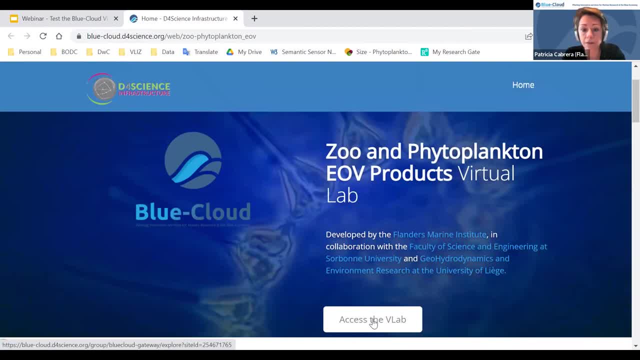 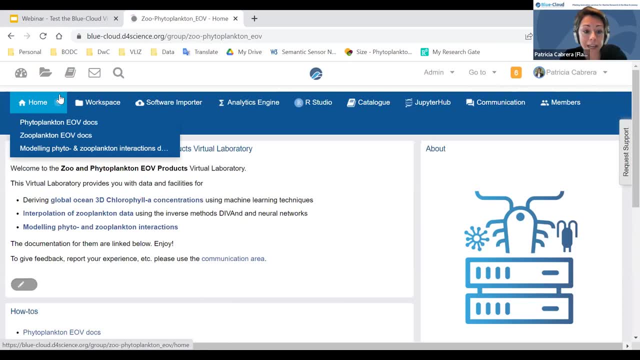 if you click here, you will need to register for me because I am already registered. it's just going to jump straight into the VLAB. So this is the landing page of the VLAB and, as you can see, here we have the documentation. 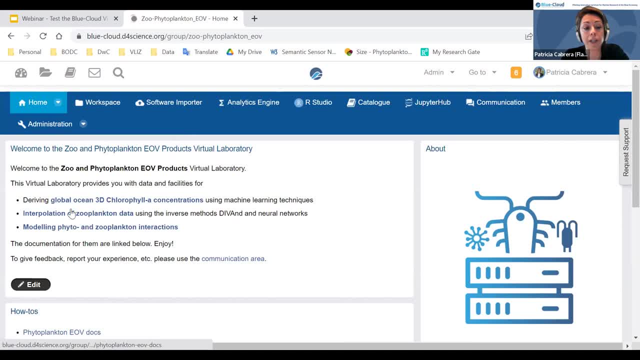 So if you click in each of these, it will give you all the steps, guidelines and a step by step on how to run the three different products that are going to be presented just right after Me. showing you this, and just something that is interesting to clarify is the workspace here. 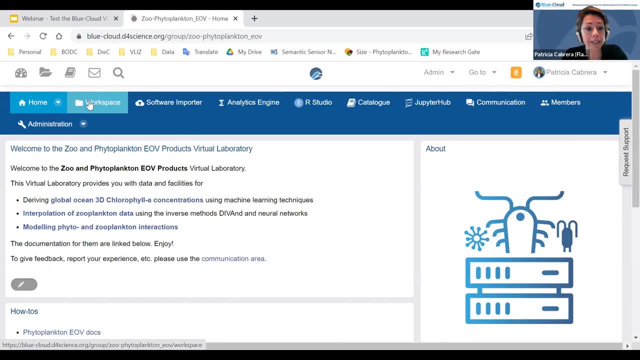 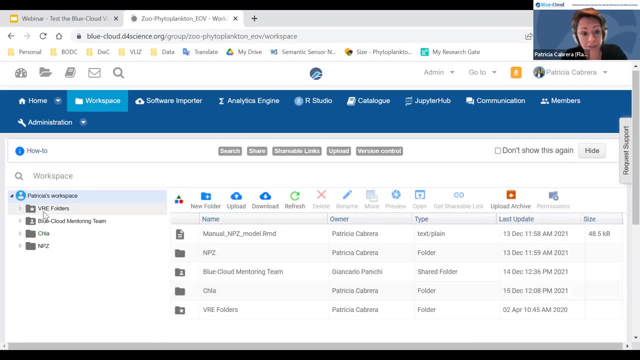 So everything to navigate is these tabs in the workspace. you land there where all the folders- your own workspace or the shared workspace, which is the VRE folders- is where everything is placed: Input, data, scripts, Jupyter, notebooks, R markdowns, outputs, results, etc. 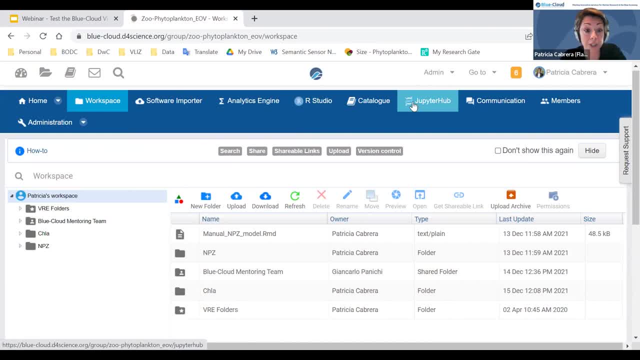 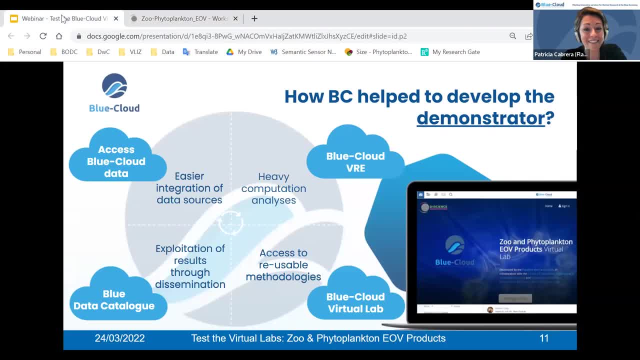 So, yeah, that's more or less in a nutshell, And now I can let Julia, who is the researcher behind the phytoplankton EOVLAB from the Laboratoire Océanographique-sur-Mer from France, that will explain you how they did this work. 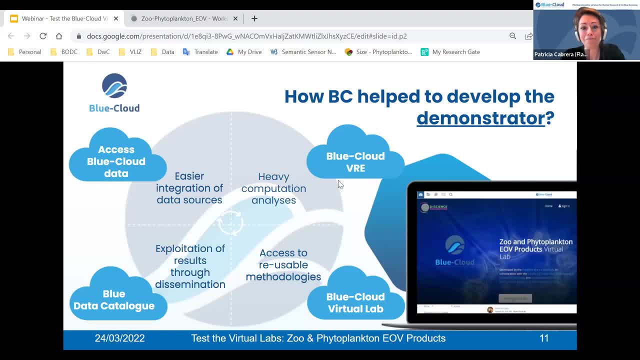 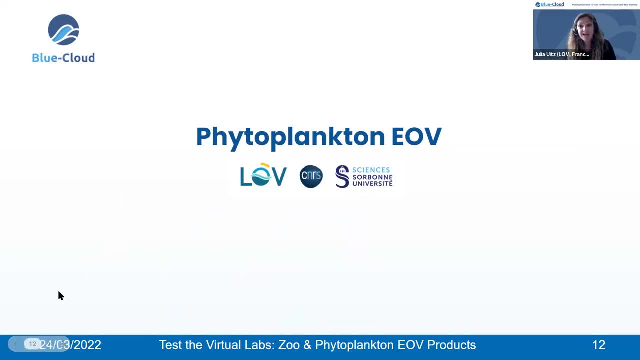 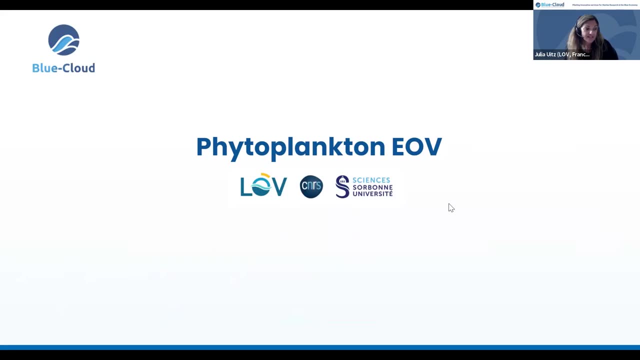 Yeah, Julia. Thank you, Patricia. So good morning everyone. I am going to present the phytoplankton EOV product that has been developed in Villefranche with my colleagues Renaud Jepelin, Poulard Gregman, who did a postdoc within the context of BlueCloud, Raphael Souset and Hervé Gloucester. 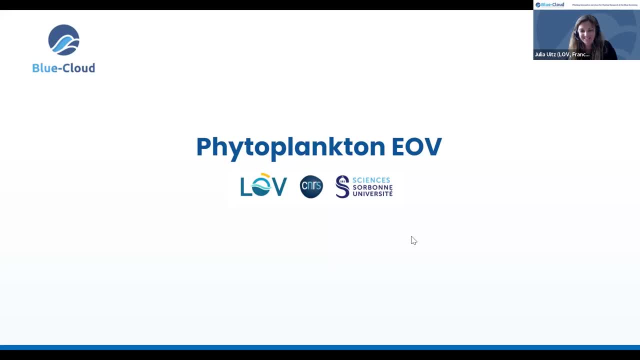 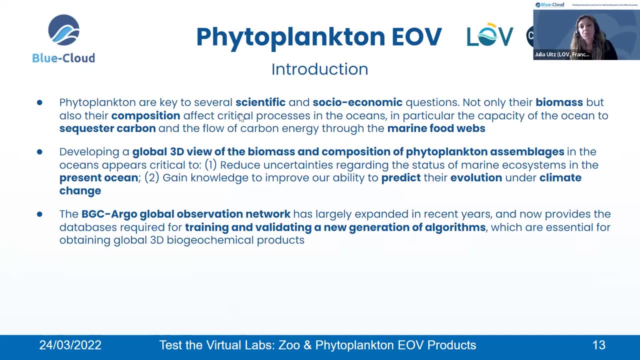 Next, please, Next, please. Thank you. So, as Patricia said earlier, phytoprotein are key to several questions relevant to fundamental research or to socio-economic issues. Not only their biomass, but also their composition critically affect processes in the oceans, in particular, the capacity of the ocean to sequester carbon from the atmosphere and also the flow of carbon through the marine food webs. 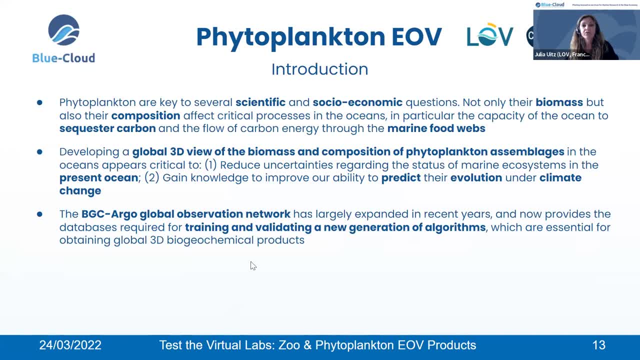 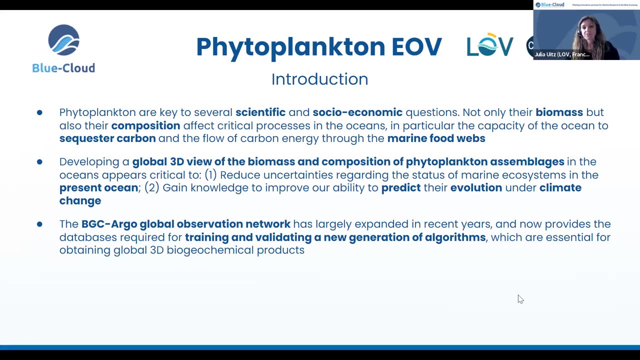 Hence, developing capability for obtaining a global 3D view of the biomass and the composition of phytoprotein communities in the oceans is critical, in particular, to reduce the uncertainties regarding the status of marine ecosystems in the present ocean, and also to gain knowledge and improve our ability to predict their evolution under a changing climate, with feedback to the entire climate system. 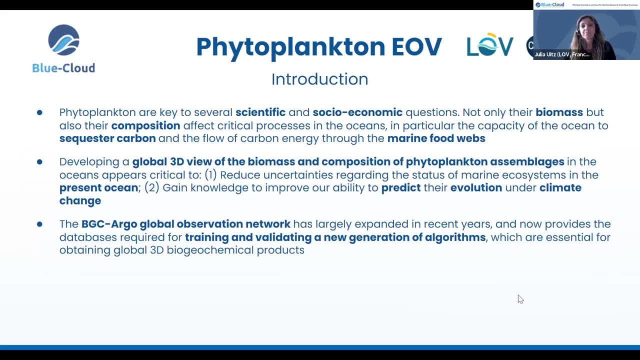 In. In recent years, the BGC, the Biogeochemical Argo Global Observation Network, has largely expanded and now provides the institute data required to train and validate a new generation of algorithms that are based on machine learning and that represent a powerful tool to develop such a global 3D view of biogeochemistry in the oceans. 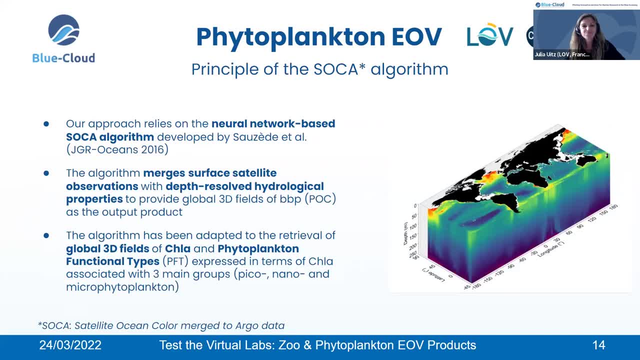 Next slide, please, Next slide, please, Next slide, please. Thank you. So, in the context of Blue Cloud, the approach that we have used is based on a neural network-based algorithm, the SUCA algorithm- that has been developed in our group by Raphael Suzette. 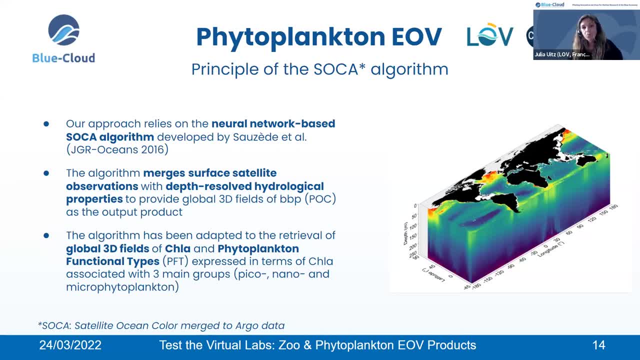 So this algorithm permits to merge surface satellite observations with depth-resolved hydrological properties of the ocean. So this algorithm permits to merge surface satellite observations with depth-resolved hydrological properties of the ocean to develop a global 3D product of the particulate backscattering coefficient. 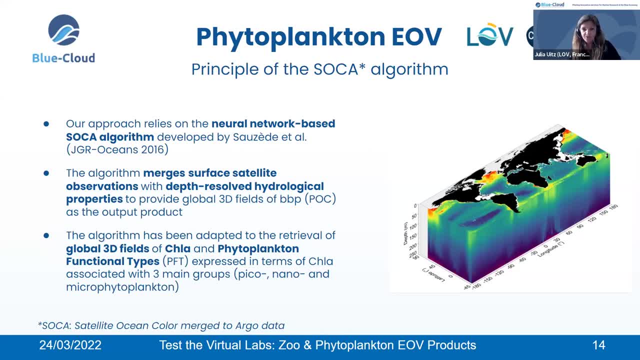 which can easily be converted into the stock of particulate organic carbon, which is a key biogeochemical product. So, for the purpose of Blue Cloud, this algorithm has been adapted in order to produce global three-dimensional fields of chlorophyll air concentration. 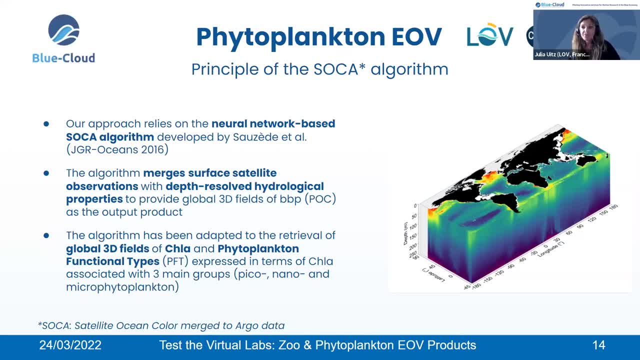 which is a proxy- a wide-use proxy- for the phytoplankton biomass and global 3D fields of phytoplankton functional types, so-called PFTs, which are an expression of the biodiversity of phytoplankton communities in the ocean. 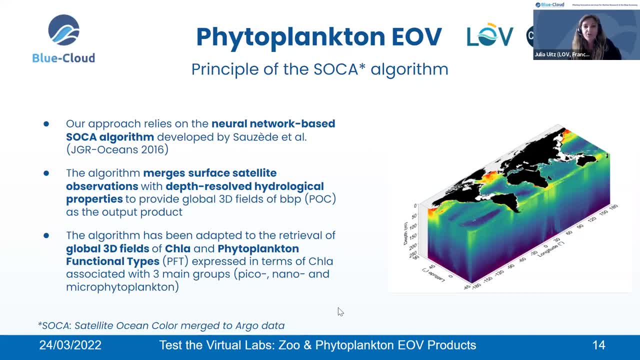 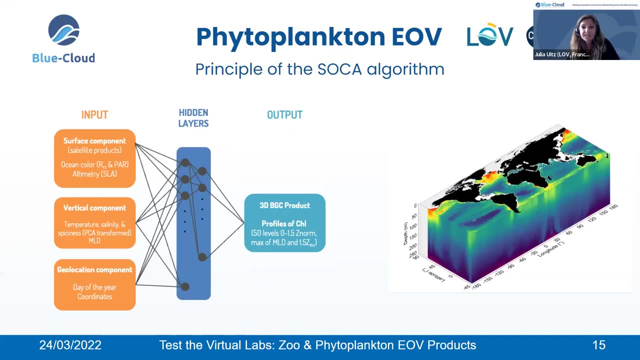 and that, in the context of our approach, are given in terms of chlorophyll concentrations associated with three main phytoplankton groups: picotin and microplankton. and chlorophyll plankton. Next one, please. So this slide shows the general architecture of the SOCA algorithm. 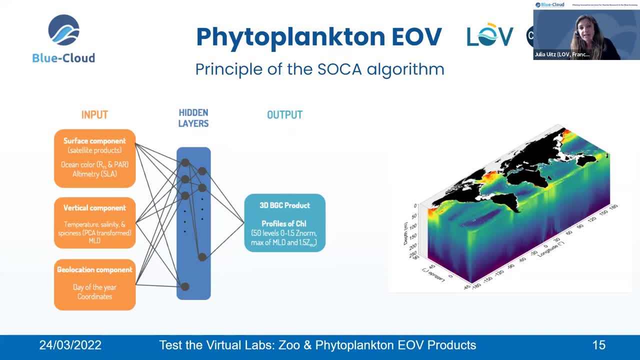 with an input layer, an output layer and several hidden layers in between. So what's important to notice here is that the input layer is composed of three main components: the surface components. that includes surface observations of the ocean, ocean color observations And this is the surface water surface observations. 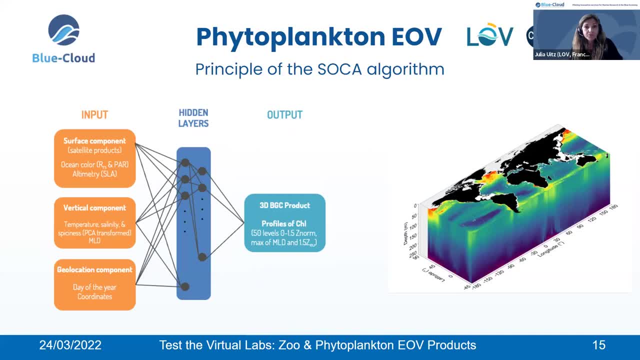 So this slide shows both surface water surface observations and the surfaceасьimetry observations. Second, it has a vertical component with depth resolved information on the temperature and salinity in particular, and a geolocation component with the day of the year and the geography coordinates. 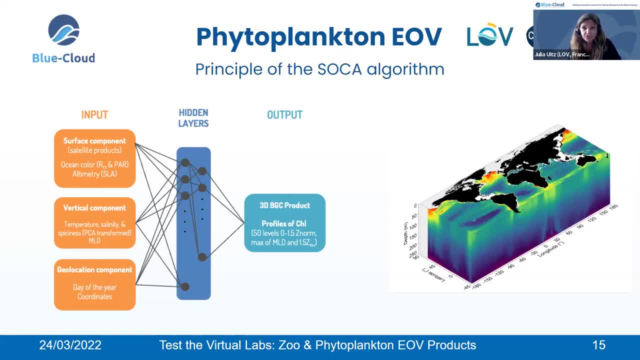 And the output product of this algorithm is going to be vertical profiles of the chlorophyll concentrations, whether associated with the entire phytoplankton biomass or, same meaning to say, with the other. So here I'm just showing the graph of the surface water, surface albums. 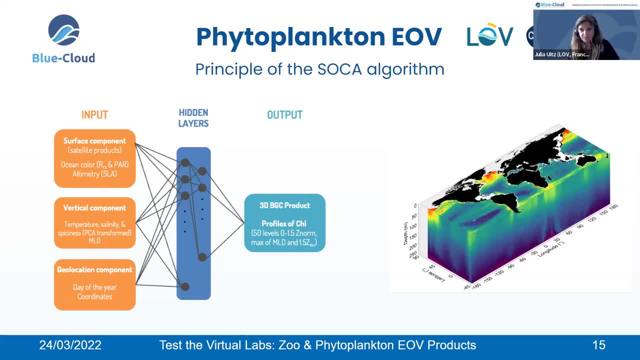 So this is a slide showing the surface water surface albums And this is a slide showing the surface water surface albums with the three phytoplankton groups- I was just referring to picotinine and microfiltroplankton- And these chlorosol concentrations are distributed. 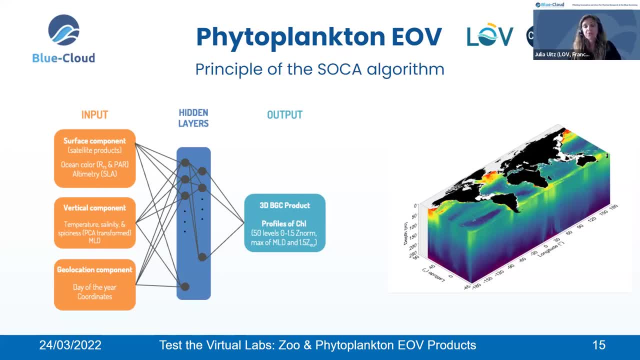 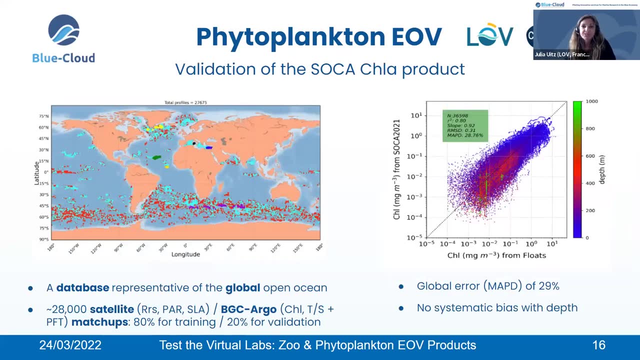 within the entire water column through 50 different depth levels. Next, please Thank you. So the SOCA algorithm has been developed using an extensive database that's representative, as much as possible at least, of the global open ocean. This database comprises satellite observation of the surface oceans. 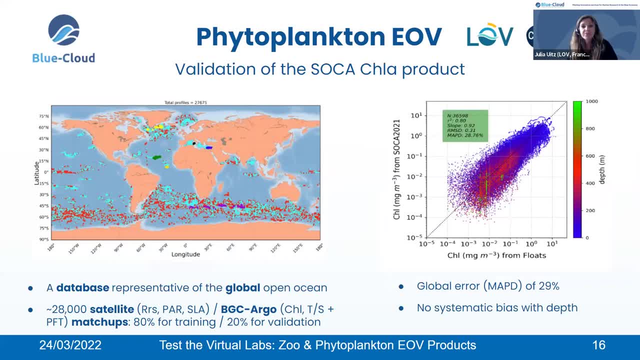 that were matched up with vertical profiles of several variables derived from in situ BGC, Argo, flood measurements. So 80% of these data were used for the training of the algorithm and the remaining 20%, that were, of course, extracted randomly, were used for its validation. 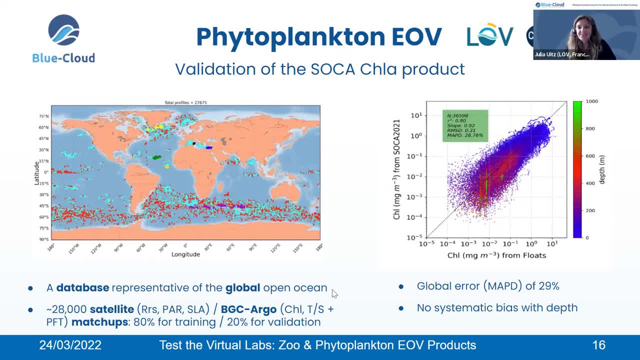 So on the right-hand side of the slide you may see that the chlorosol concentration derived from the algorithm on the y-axis compares quite well with the chlorosol concentration measured in situ, with error square value of 0.8, a slope that's close to 1,. 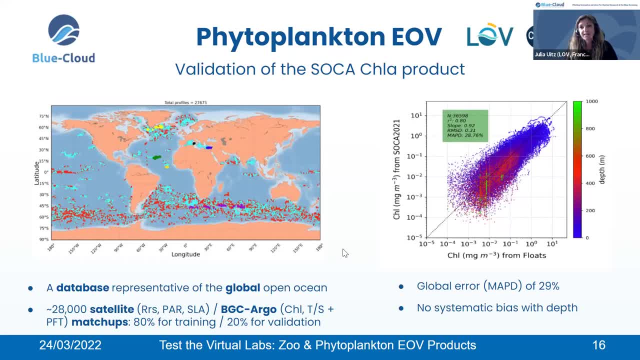 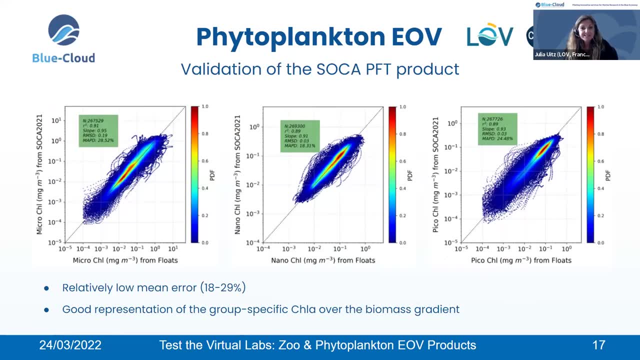 and a relatively low mean. relative error of less than 30%. Next slide, please This slide. on this slide, you can see the scatter plots for the validation of the chlorosol concentration associated with a micro on the left, nano in the middle and pico on the right side of the slide. 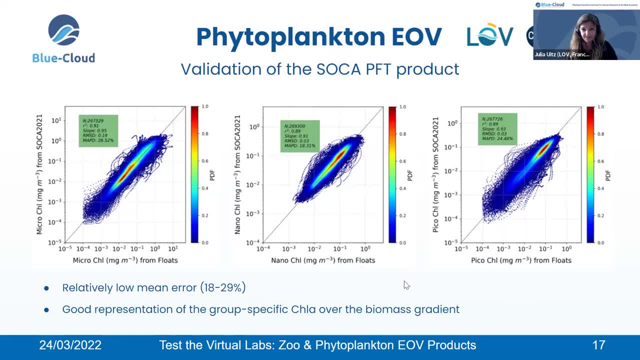 So these scatter plots tell us that the algorithm performed relatively well for each of the three phytoplatin groups, with relatively low mean error of less than 30% per second. Next slide, please, So you can see that the algorithm performed relatively well for each of the three phytoplankton groups, with relatively low mean error of less than 30%. 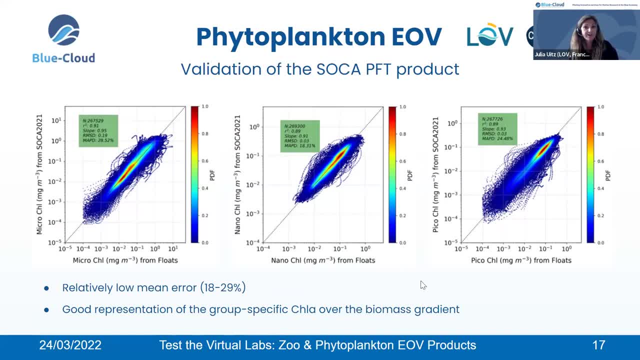 even less than close to 80% for the nano-microphyte plankton. And what's also interesting to notice is that the algorithm is able to reproduce quite well the dynamic of chlorosol concentration for each group, even for the pico phytoplankton, which is on the right-hand side. 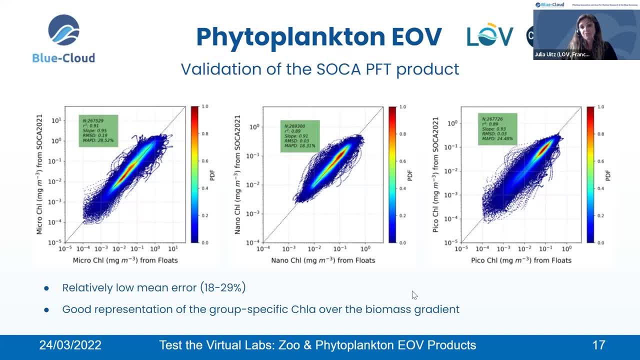 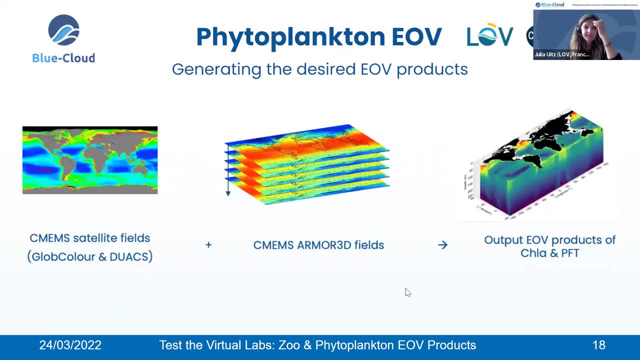 which is usually more difficult to predict because it varies in the very narrow gradient of chlorosol concentration. Next slide, please. So one possibility for applying this algorithm and generating the desired phytoplankton EOV product is to use as input to the algorithm. 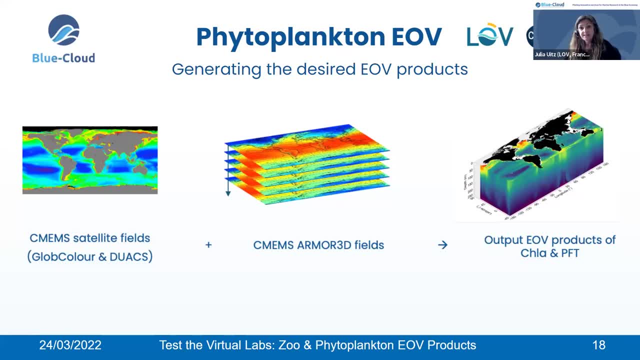 surface satellite fields and depth-resolved hydrological property fields derived from the well taken from the Copernicus CMMs catalog. So this is what we've done here. I'm going to show you an example of the output product. If you can move to the next one, please. 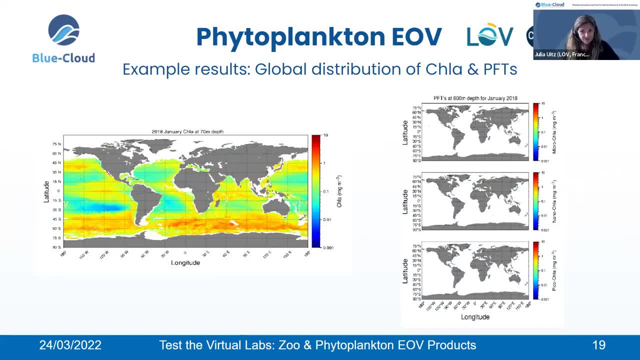 Yes, So that's the global distribution obtained from this application of the algorithm. Chlorophyll A, associated with the entire phytoplankton biomass on the left and the three different groups of phytoplankton on the right. That's an example of application for the month of January 2018.. 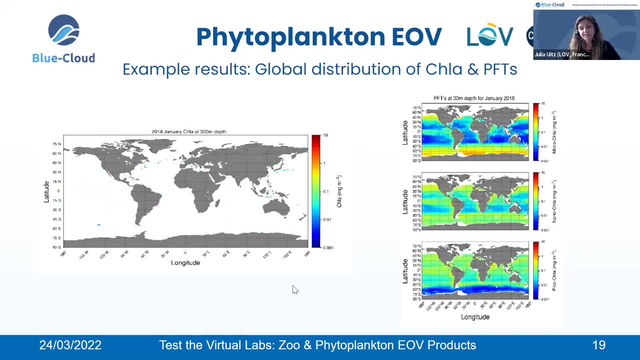 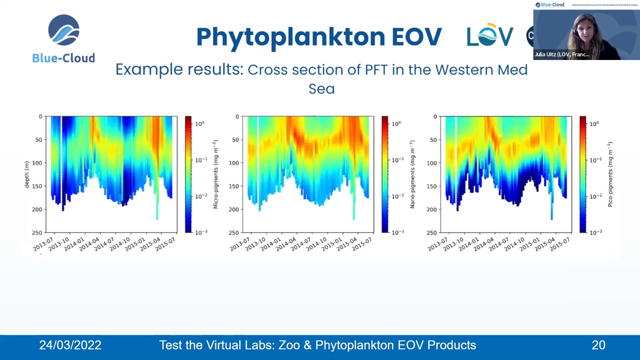 And the animation shows The concentration changing with depth from the surface down to 100, 1000 meter. But that's not super easy to visualize, So let me show you, on the next one, a cross section that has been extracted for the Western Mediterranean Sea, which is a very dynamic region. that's been extracted from the global product. 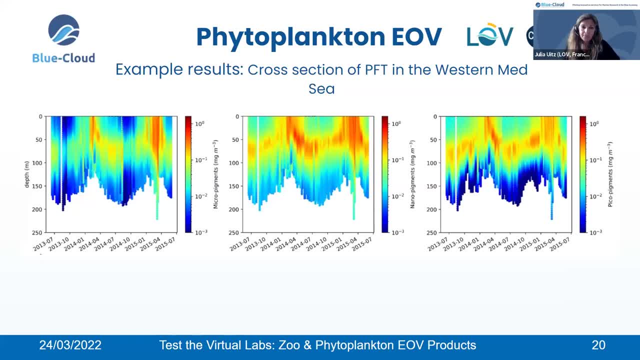 And that permits, that allows us To visualize the seasonal and the vertical variability of the biomass and composition of the assemblage. So that's for this, that's in the Ligurian Sea, the Northwestern Mediterranean Sea. So, as you can see, we observe each year an increase of biomass in the surface layer of the ocean and that coincides with the recurrent spring bloom that occurs each year in the Mediterranean Sea. 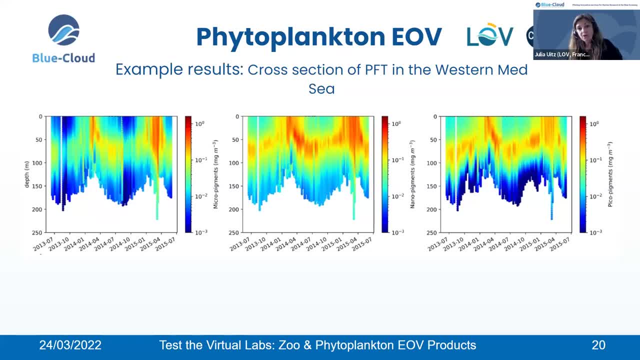 In the in its western basin, and that's followed in summer by a deepening of the biomass and an increased contribution of small phytoplankton, and that's that's that's coincided with them. this pattern coincides with the summer oligotrophic period. 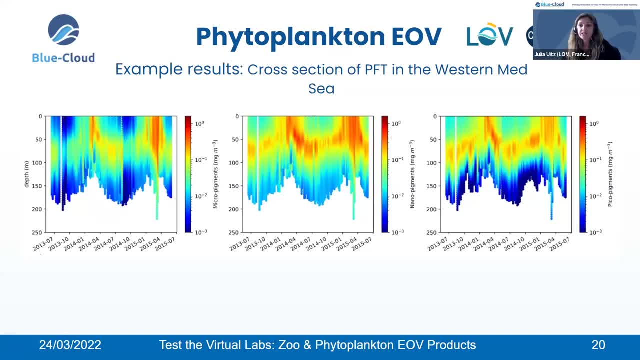 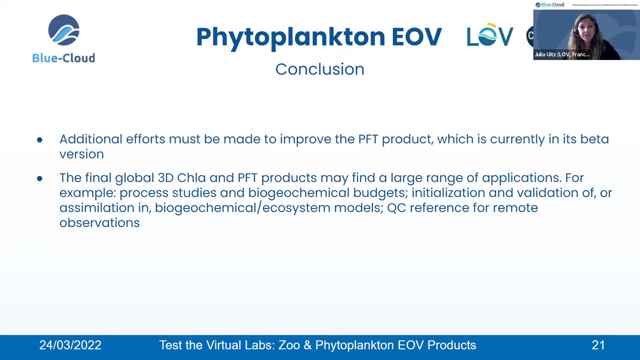 So that's very consistent with expectation: knowledge of the distribution of the biomass in the global ocean. And I guess that we are moving to my final slide. Thank you, slide please, Thank you. So to conclude on the methodological note, I have to say that additional efforts will. 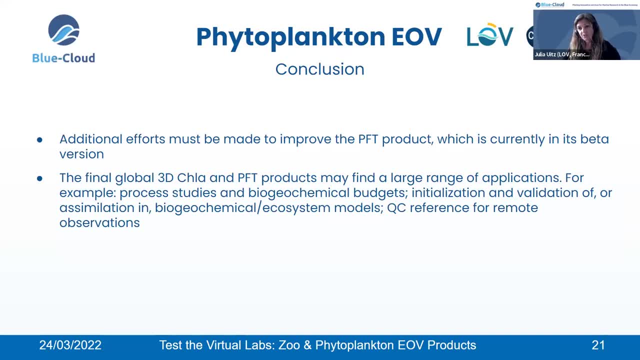 need to be made in the near future to improve the PFT product because currently it's the very, it's a very better version, Although it provides already satisfactory results. And, this being said, the fight. we expect that these final, the final global 3d product of crossland PFT will find a large 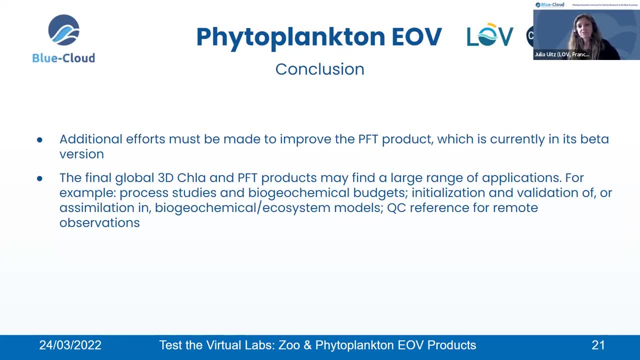 range of applications. for example, but not only, they could be used for fundamental research purposes studies or to draw large scale biology chemical budgets. This could also be used for the initialization or validation of the new generation of biology chemical models that are currently explicitly integrate different fight present groups. 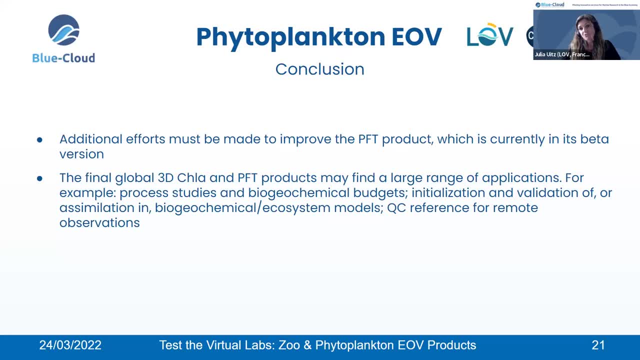 or, for instance, from a more operational perspective, it could also be used If we derive climatological product. it could be used as a reference to qualify near real time data from global remote observation network. And I'm done, Thank you. 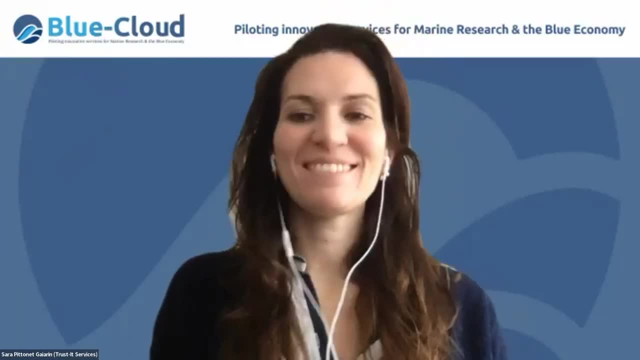 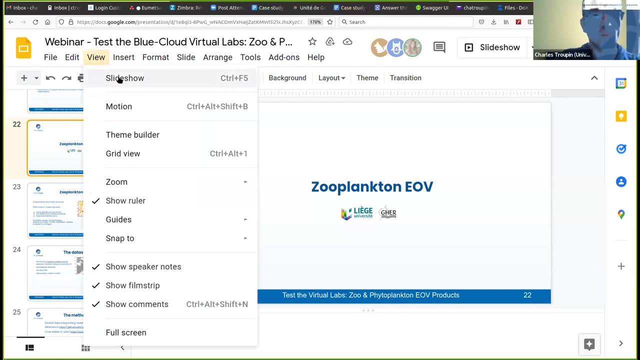 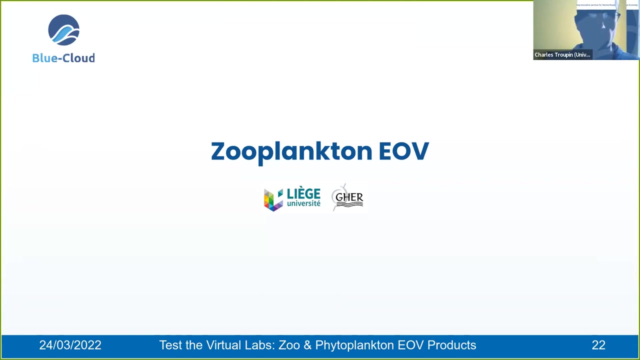 Many thanks, Julia, And now it's the turn of Charles Charles Rupin. Okay, thank you. So I will talk about now the zooplankton EOV developed at the University of Liège, essentially by my colleague Alexander Brat. because of agenda conflict, could not make it. 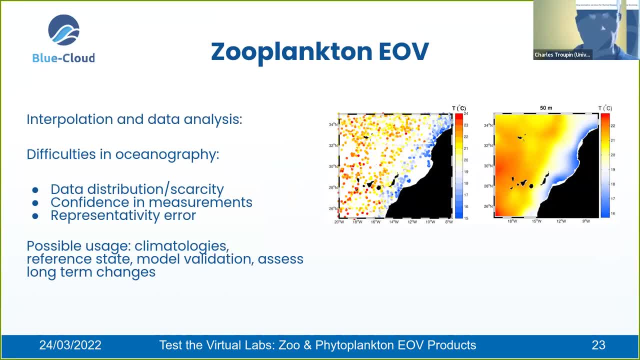 today. So what we're doing in Liège most of the time we're trying to interpolate data. That's what we show in this figure. So you see all these dots that are typical distribution of measurement, in this case temperature for a given month at 50 MHz. 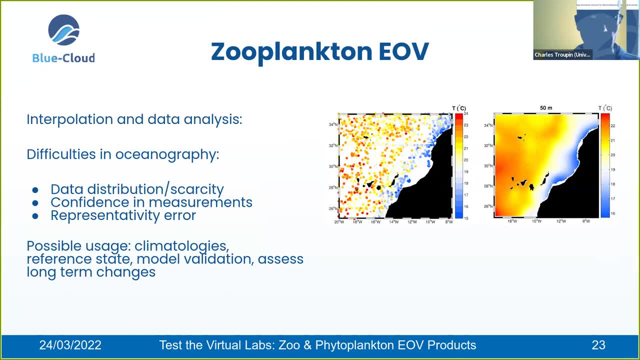 And what we want to obtain is something that we see on the right, which is a gridded field, an interpolated field, And it's a typical task in oceanography, but it's not easy because of the data distribution. you have a lot of gaps, But, at the same, 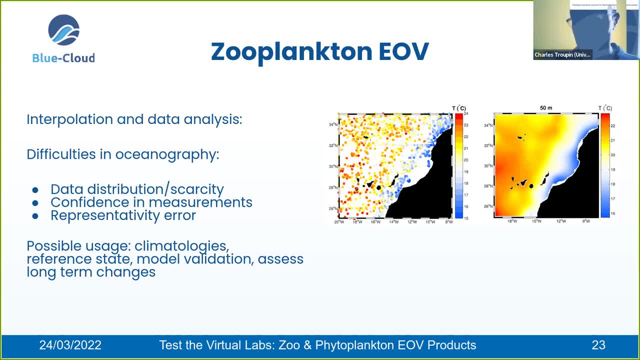 time you have a lot of data. then you have the different confidence in the measurement. some measurements you trust them a lot because you know them. some of them are larger error And finally the present representativity error, which means we try to create a gridded field which is a representative. 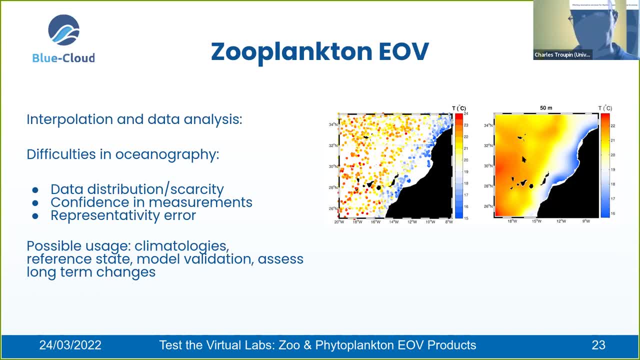 of the long term condition using data collected at given times. So it's, it's difficult. So why you use that we use this? climatologist is gridded field for model validation, for example, or to assess the long term change. So there are many. 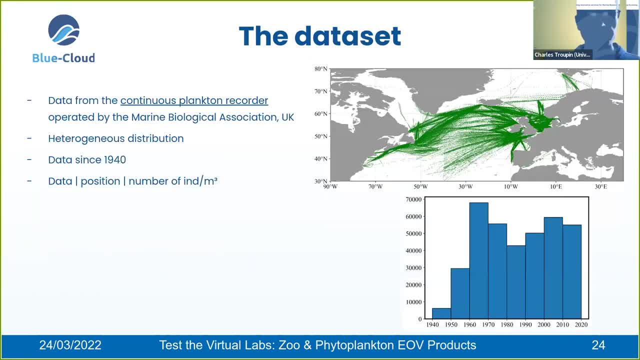 usage or just the visualization of the data. In this project we've worked with the CPR data continuous plankton recorder. they are provided by the MBA, the marine biology and the geological Association in the UK And you can see the typical. 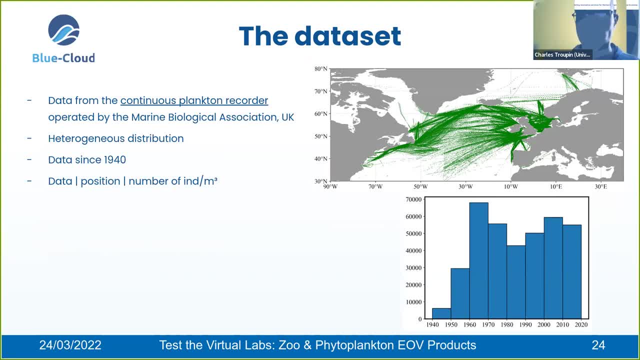 coverage on the map on the top right side. So these types of data, what they consist of in fact, with a position, and then the concentration, a number of individual per cubic meter, And with this data we want to create a gridded maps as the 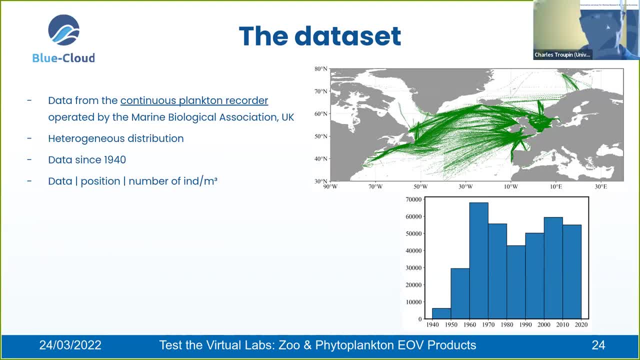 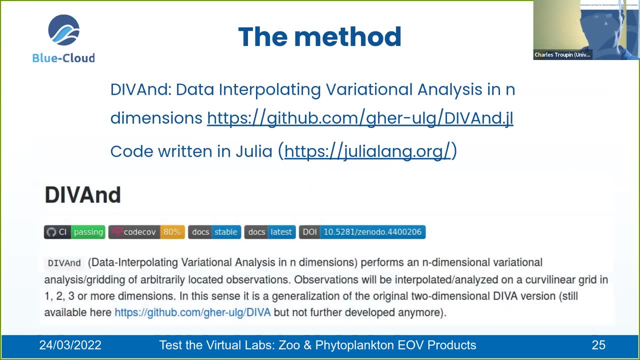 previous slide, So the data distribution is rather good. So we have data since the year 40s And we have even data up to today, Almost. So the method that we use it's called diva, nd, So develop or read you heard of. diva means data interpolating. 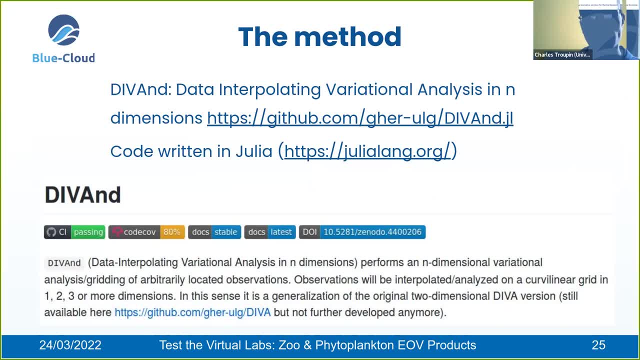 variation on analysis And the nd means we are doing that in n dimension, So the dimension can be longitude, latitude and depth, and time and other dimension if we have. So the code is available on GitHub. It's called diva ndjl. jl means 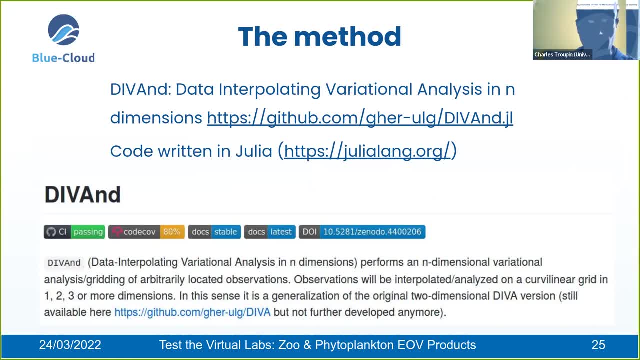 it in Julia. So the Julia is a very powerful language that we have used. We've been used for the last years and it's very quick, very fast. So it's a good thing for us when we have to deal with a lot of data. So 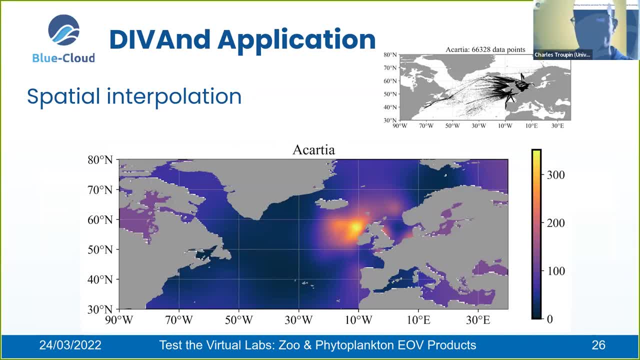 the application here. on the top side you see a map of typical distribution, which is called a cartier, one of the species that we study with 66,000 data points, And the big map in the center is, in fact, the map that we obtain with the interpolation. 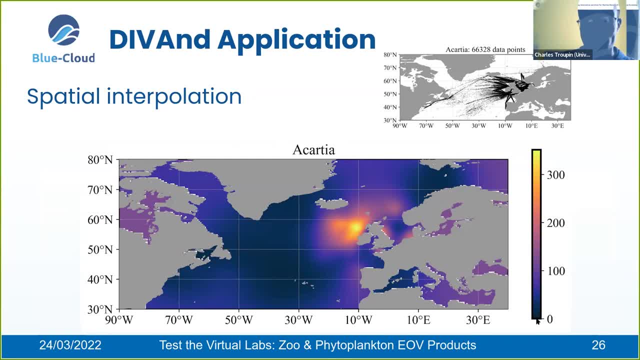 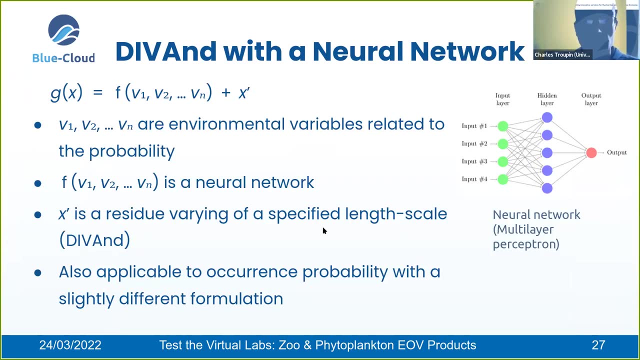 So we see the distribution, really concentration ranging from zero to something more than 300. And it allows us to show which area are more propitious to get to observe more of these species. But we did not only do these techniques, we also develop neural network technique. 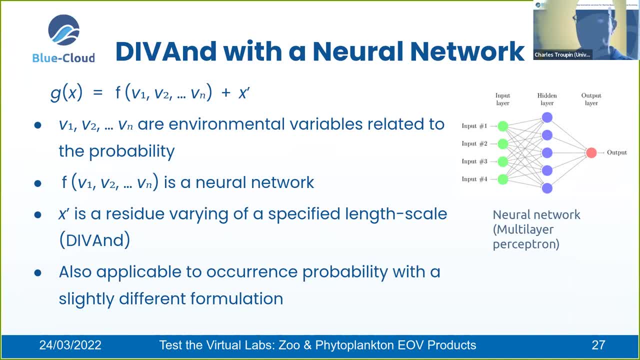 I will explain you how it works. So the idea behind that is that a given species is driven by different factors, different environmental variables- In this case can be temperature, for example. we know that temperature will influence them, So we will put all these what we. 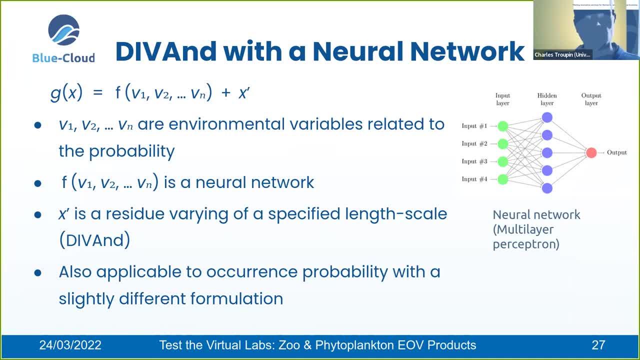 call them the core variables inside the neural network to derive the concentration or the probability of occurrence of a given species. So here we have v1, v2, vn. the core variables, f is the neural network and x, prime is a residual varying for given length, scale within 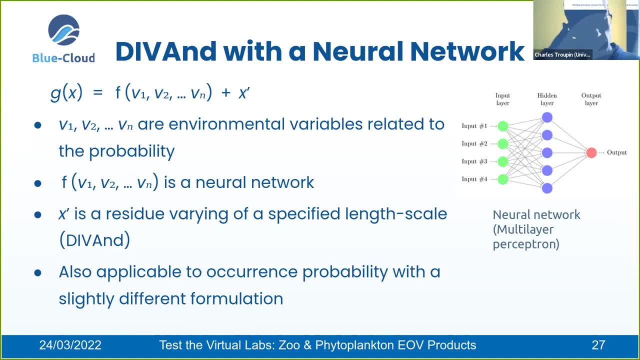 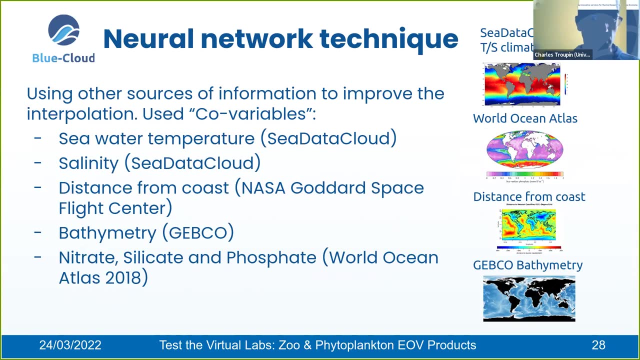 divine deep. So the methodology is rather complex, But the idea is, yes, to use different variables to reproduce the layers of different species. When we talk about core variables, we need typically the seawater temperature, the seawater salinity, and we take them from the sea data. 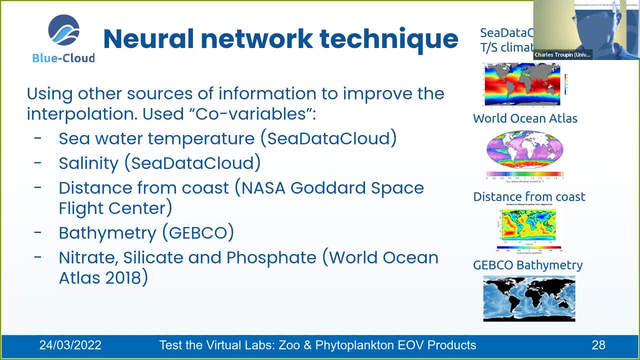 cloud infrastructure. Then we also need the distance from the coast, which is a very relevant variable, the bathymetry from GEBCO And also nitrate and phosphate concentration. we take them from the world ocean atlas, So all these data are available within the VRE, the blue cloud VRE. 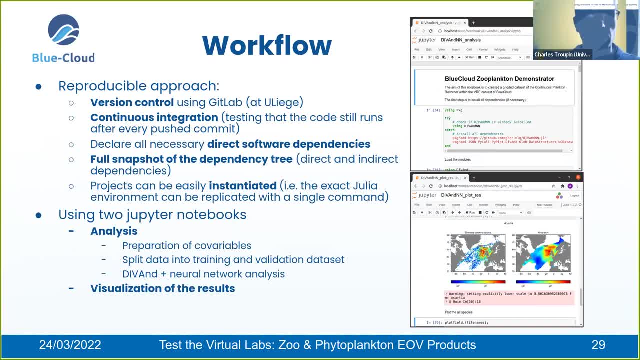 and we just need to process them. How does the workflow work? So we want to have a reproducible approach. This means that anybody should be able to redo the computation with the same environment. So first of all, we use the version control, which means the code that. 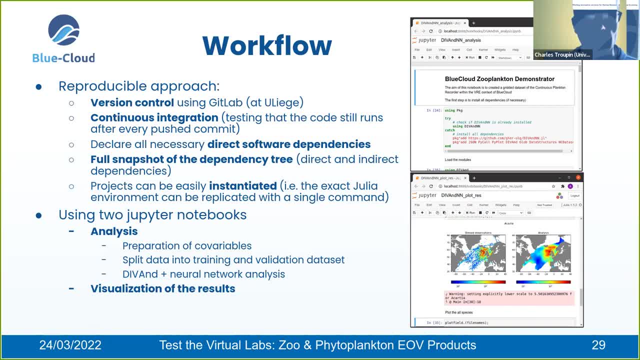 we run is managed using Git In particular, in this case, GitLab instance at the University of Liege. We use a lot the continuous integration. So for those of you who don't know this, continuous integration means every time we modify our 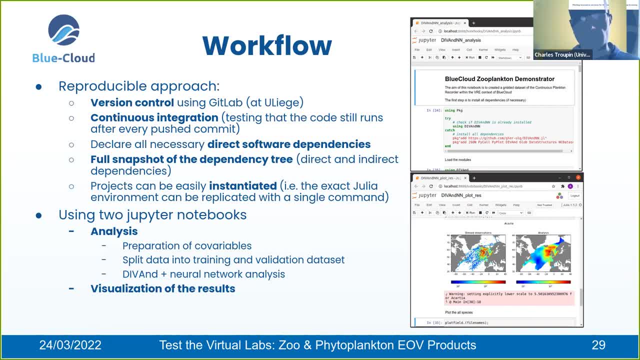 code or change a version of a package. there's a set of tests that are automatically run on the code to check if everything is as expected, that we did not break anything by doing our changes, So it's very important to have this in this kind of tool. 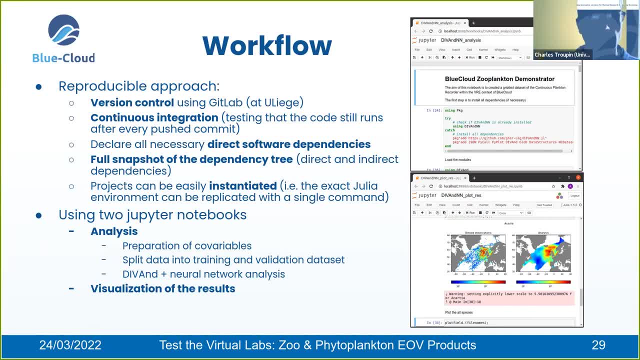 So all the software dependencies are declared inside the project and then you have a full snapshot of the dependency tree. So it means you really can recreate the exact same project to rerun the code. We use two Jupyter notebooks. The first one is for the analysis, So it prepares the 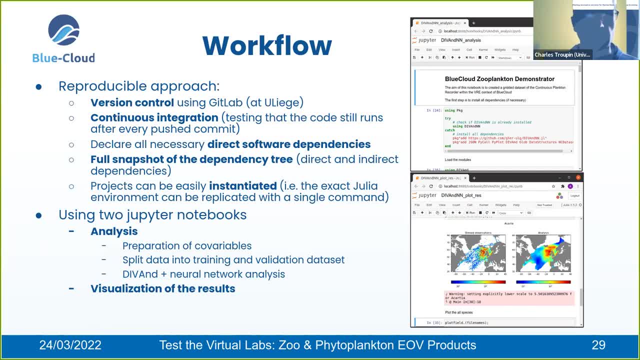 covariables, as we see in the previous slides, split the data into two components, The first one for the training and the other one for the validation. Then it applies div nd plus the neural network approach, And the second notebook is for the visualization of the results. 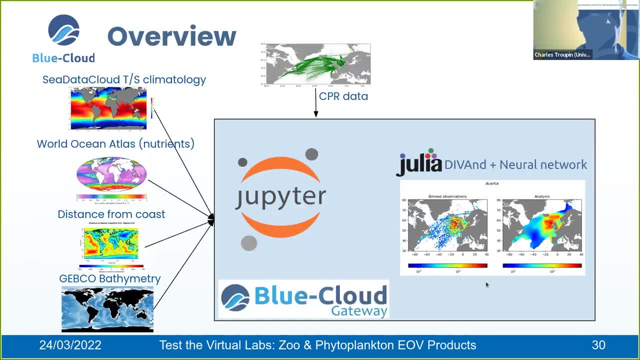 As you can see in this map on the right side On overview, so you have the main input data, the cbar data. Then on the left side you have the core variables going all together inside the blue cloud infrastructure where the JupyterLab instance is run And we can have our tools or notebooks with Julia. 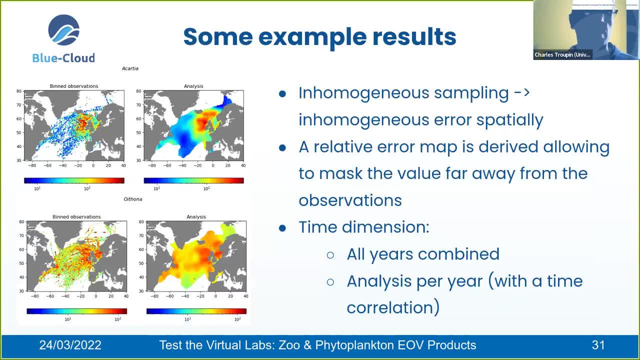 running div nd plus the neural network. Some example of results: we've taken again the Akartia species. On the left we have the observation and on the right the analysis. The same for Oitona: the observation and the analysis. So what you? 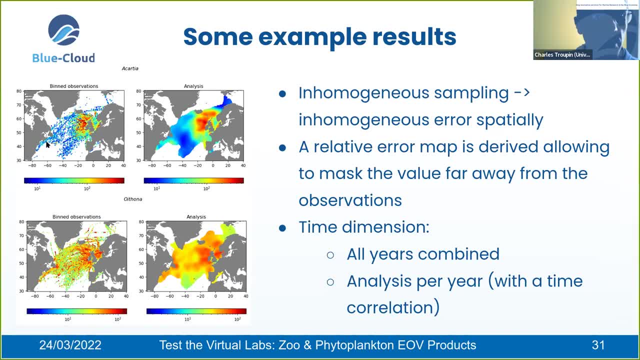 need to note here is that you have a lot of blank areas. So it means in these data, these areas, we don't have data, So it means the expected error is quite high. So with our approach you can create not only an agreed field but also an error field, And if the error is above a given value, 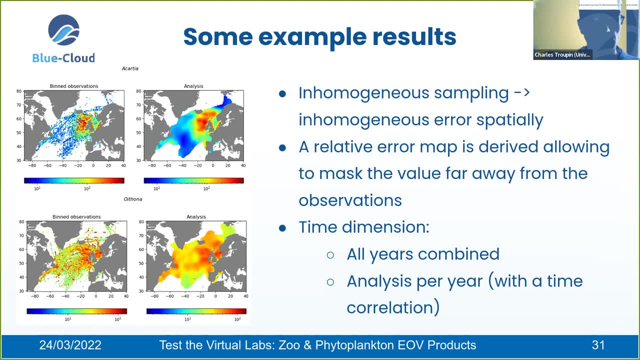 for example, 30%, we say Okay, we don't want to show the analysis because we don't trust and typically means because we don't have measurement. So no measurement means high error. So we don't want to show the analysis when the error is too. 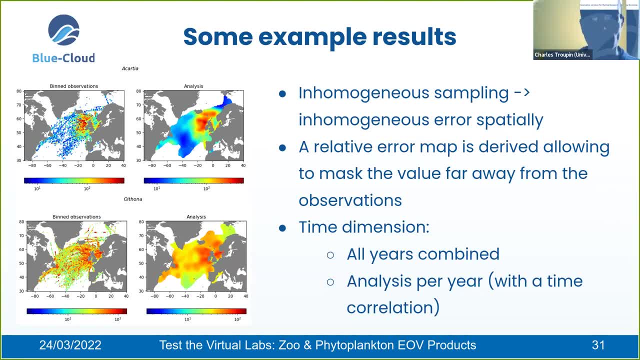 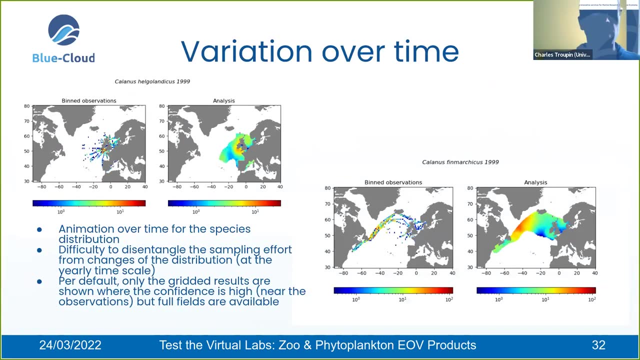 high For the analysis. We have also worked on the time dimensions. we can take all the data all together for the since the 40s until now, so 60 or 70 years of data, or we can analyze year by year. if the data coverage is sufficient, We can also 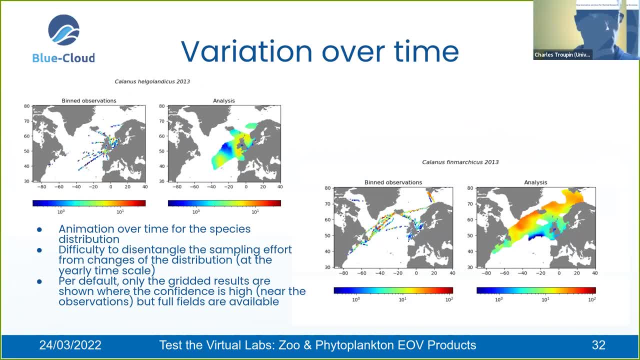 dedicate efforts to study the variation over time, which is a very interesting exercise in some cases- of species. In this case, we have Calanus ergolandicus and Calanus finmarkicus- and what we've done? we have created all the fields year by year and create an animation for the different. 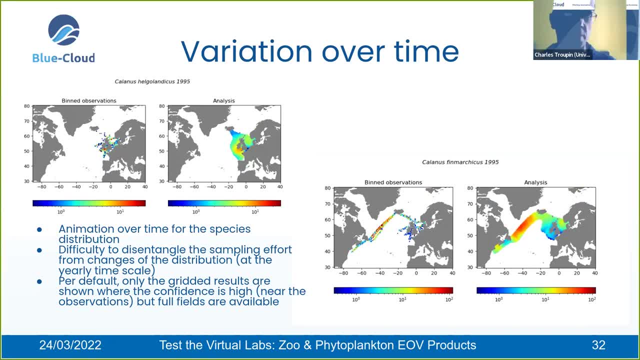 concentrations. So the problem is that it's often difficult to disentangle the sampling effort from the change of distribution. so every year the sampling is not exactly the same, so we can have the impression that the concentration increase or decrease. but it might be an effect. 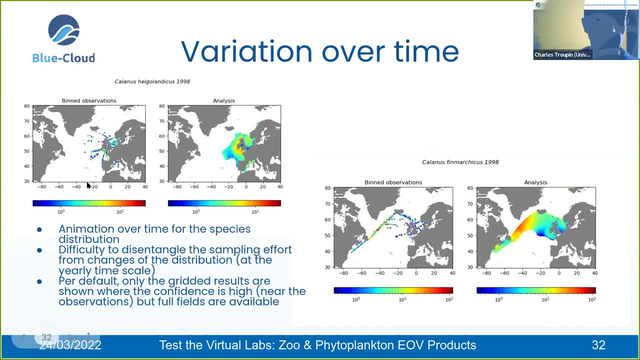 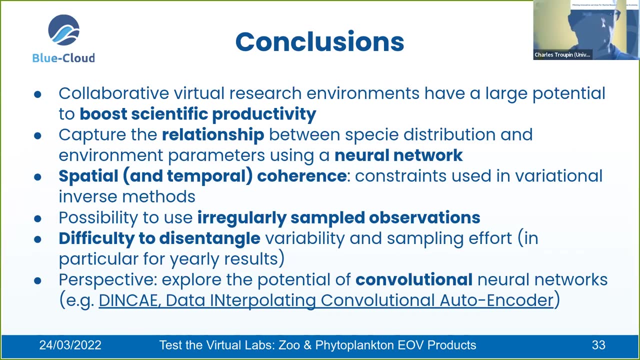 of the distribution. So here we show only the gridded field, taking into account the error, but we also provide for this case the full gridded field and the error field. So a few conclusions of this work. so we really believe that collaborative vitro research. 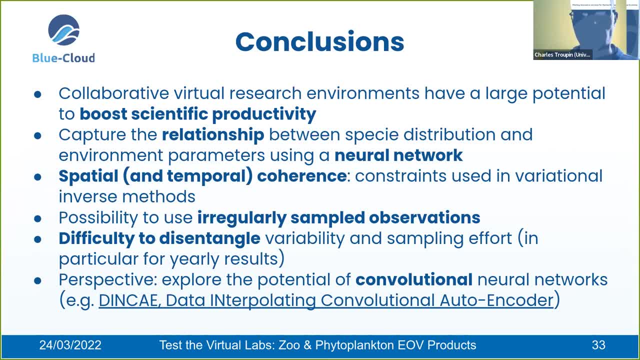 environments such as the one implemented within blue cloud have a very, very big potential to boost the scientific productivity, because it means you don't have to download data, you don't have to install softwares, you don't have to buy a new computer. everything is there for you. 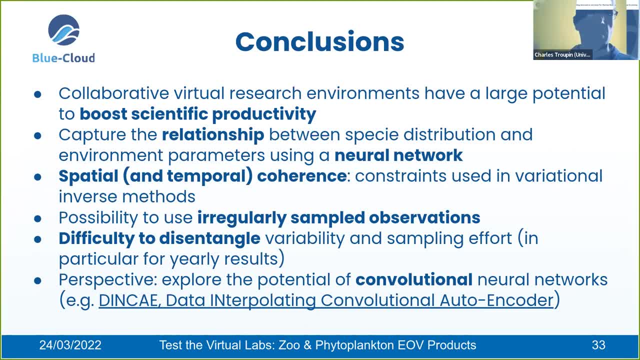 You'll be able to capture the relationship between species distribution and environmental parameters and the neural network. So the spatial and temporal coherence, the constraint used in the method, the particular diva, allows you to really take into account specific constraints such as occurrence, presence of cost, etc. Possibility, of course, to use irregularly sampled observation. 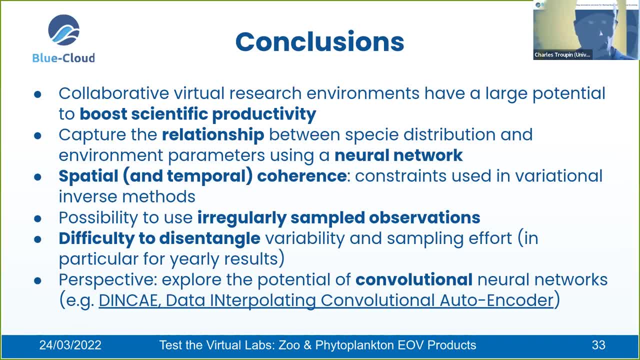 which is the reality in most of the variables in the ocean that are not regularly sampled, and also, as mentioned just before, difficulty to disentangle variability and sampling effort. As a perspective, we think in our case we would like to explore the potential of other techniques, in particular the convolutional neural network, and we have a method which is 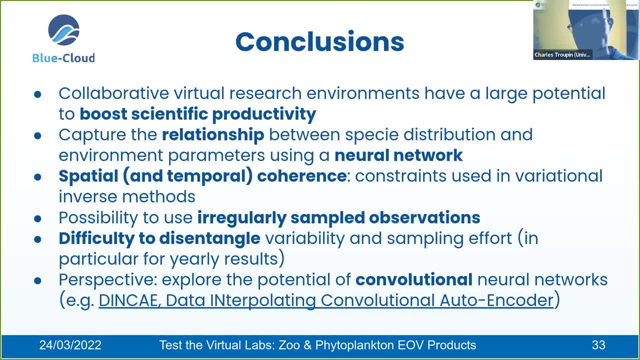 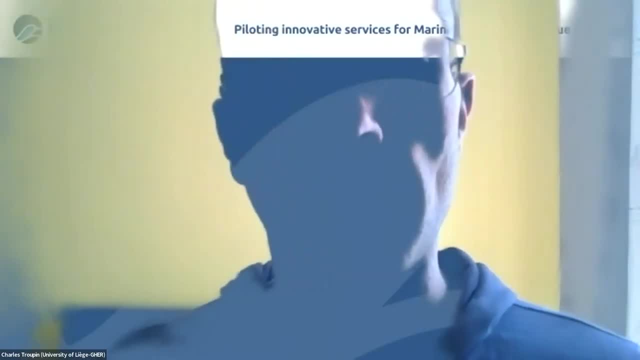 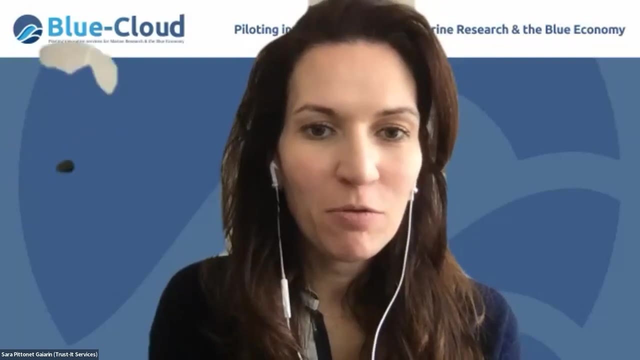 called DINCAE, data interpolating convolutional autoencoder, that we could or will try on a new data set and again make the tool available to communities. That's all for me, thanks. Many thanks, Charles, and while you were presenting, we received a couple of questions. 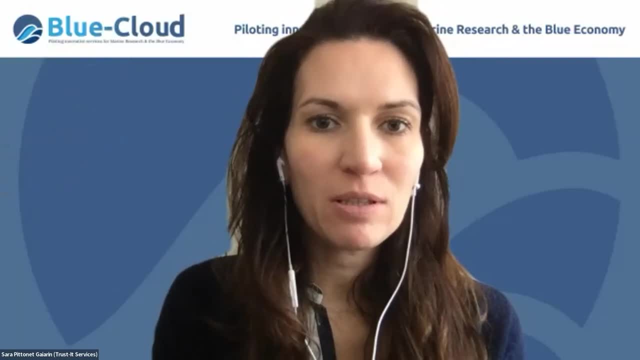 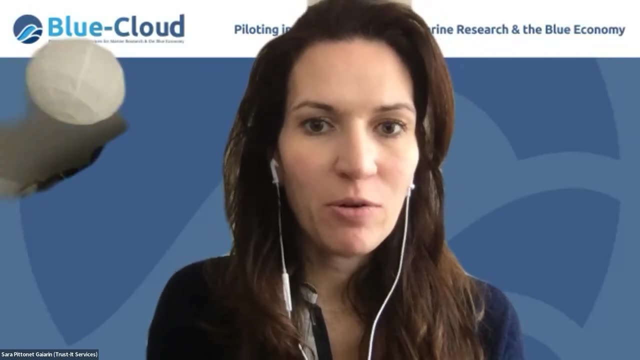 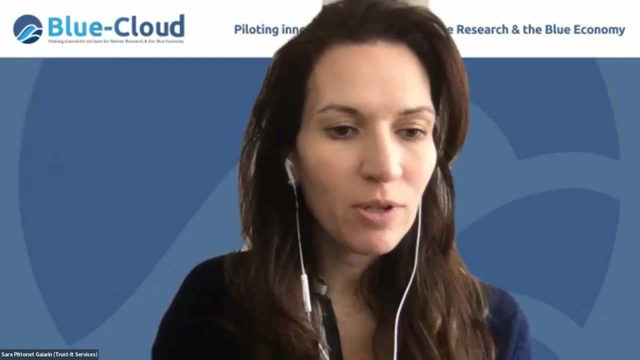 One has been addressed already, was asked by Veronique, and it was about the distribution scale of the phytoplankton biomass. so Julia replied already. I don't know if you want to say something, something more, also for the benefit of the the others. otherwise, 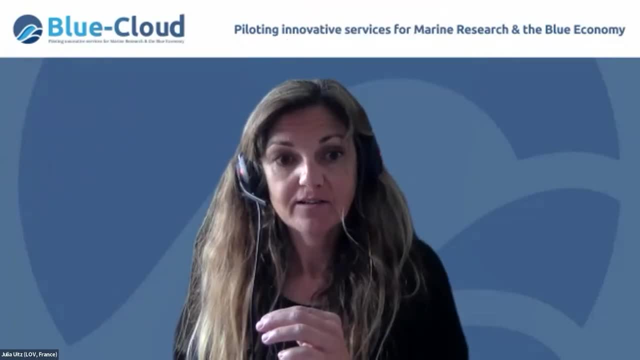 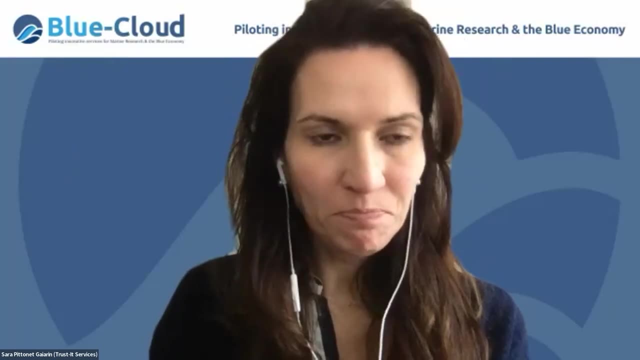 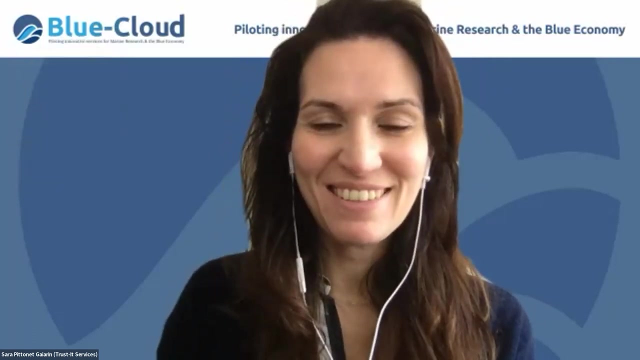 Is it better if I type the answer inside the, the Q&A, or Yes, yes, so we are. we are for our participants. we are typing the answers. I believe everybody can see the answers in the, but I mean, it was just a way to say some additional clarifications to Julia. 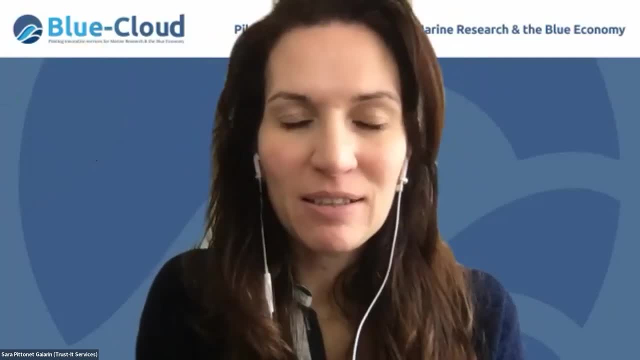 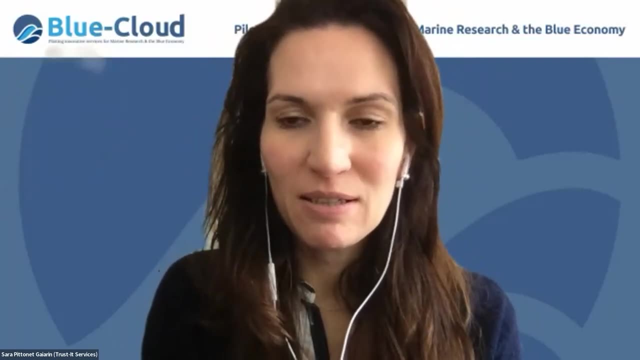 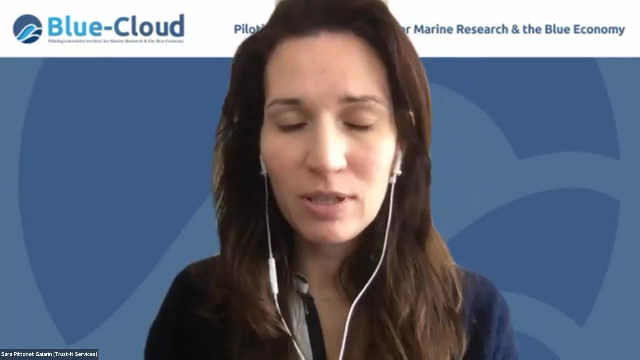 Otherwise, there is another question by Laura. Laura, did you try to use the data from in situ monitoring program for MSFT assessment? I'm not sure who is this question for. is for Charles or Julia? I will try to reply anyway in the Q&A. 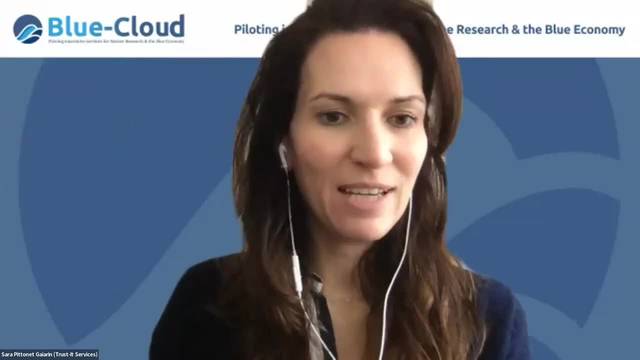 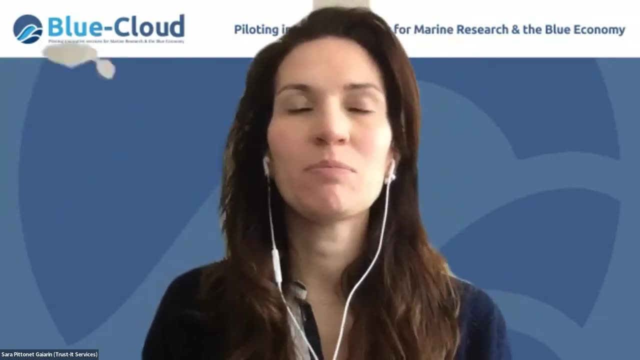 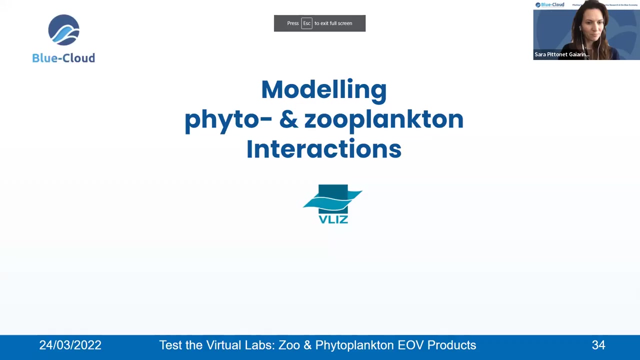 Okay, great, so have a look there, and so in the meantime we can move on. we have a last presentation by Stephen Penn. Yeah, thank you, Sarah, for the introduction. so here at the Flunders Marine Institute we were working on a model where we were incorporating phyto and zooplankton interactions, and so short introduction about that. 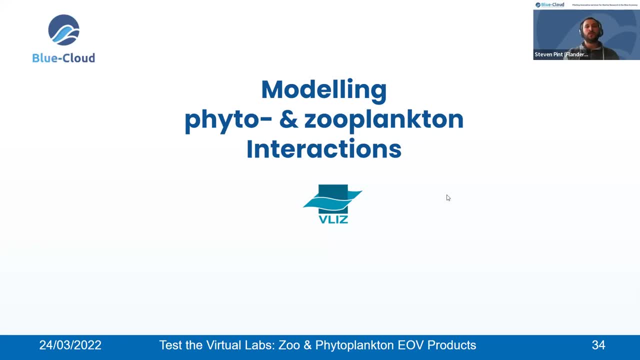 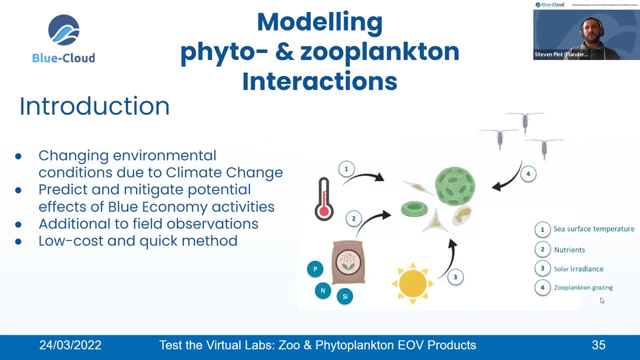 what's important for phytoplankton, what's changes or influences on phyto plantings that we are working on now? and then we had the question that the final picture shows, and then we saw the concept of the plant. So we say what is important for the plant? 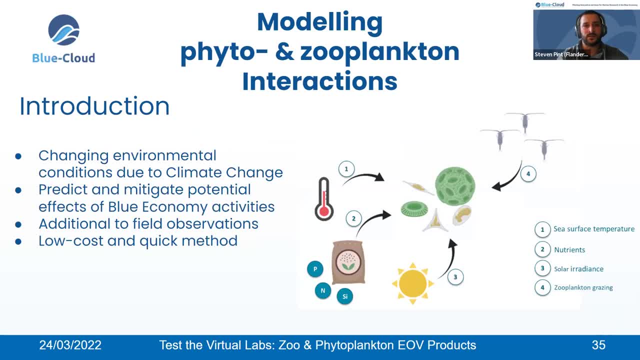 and then the final question that we make is about what is important for the plant is biomass dynamics, it's sea surface temperature, nutrients such as phosphorus, nitrogen, silica. further, we have solar irradiance, and then we also have the interaction with the zooplankton. 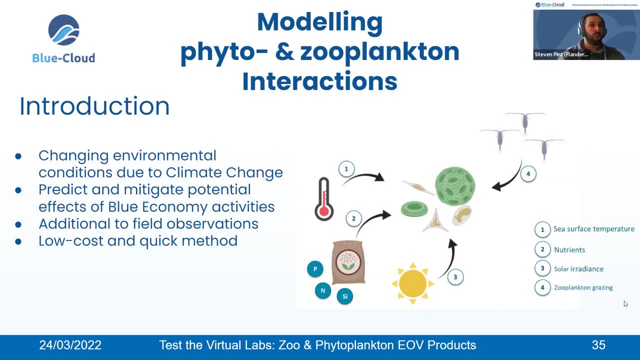 that is grazing on the phytoplankton. why could we use such a model? because the environmental conditions are changing and will continue to change due to climate change. further, it can be used to predict and mitigate potential effects of blue economy activities, and the model can also be useful for monitoring programs to fill in data caps, so it can be. 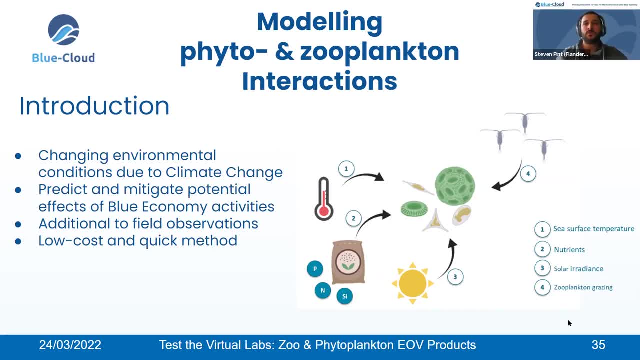 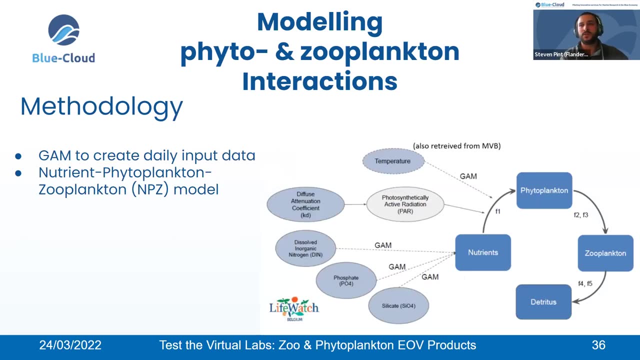 used additionally to field observation. further modeling in general can be relatively low cost and a quick method to explore different scenarios and solutions further. let me talk about the model itself. it's a model that is used to predict and mitigate potential effects of blue economy activities. a nutrient, phytoplankton, zooplankton- model, where the interactions are quantified through 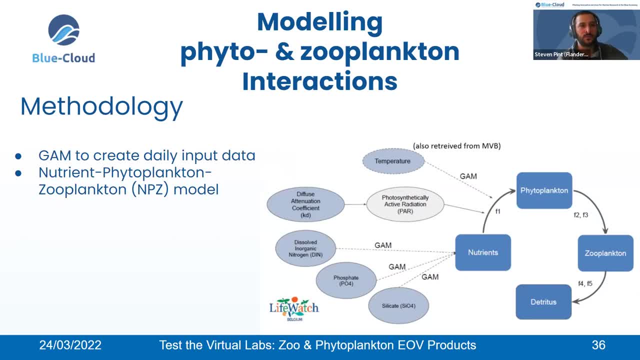 mathematical equations. you also have to try this in there, but we kept the constant. so what do we feed to this model? we feed daily input data from temperature, solar irradiance and nutrient data, and we create this daily input data with generalized additive models in combination with a. 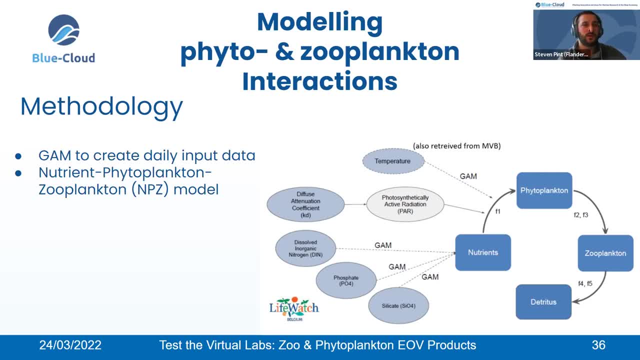 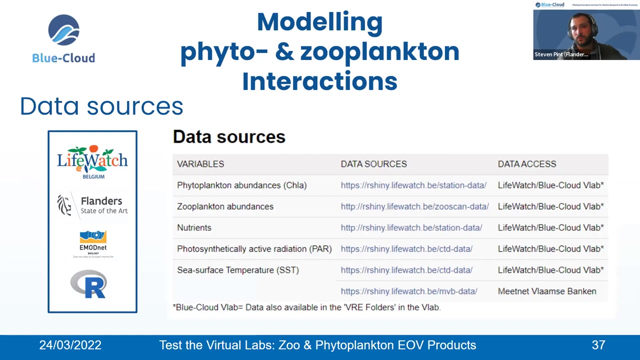 field observation that we collected from lifewatch and the flourishing monitoring network. so we use field observations with some generalized additive model to create input data for our model. the code for the gam models is also available in the blue cloud and our data sources are provided and there is an overview provided in in the vlab where you can have a look at the. 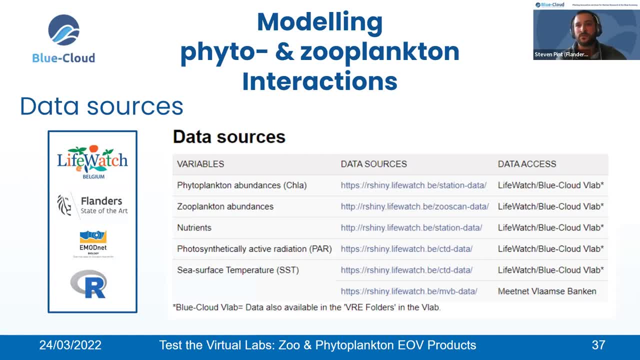 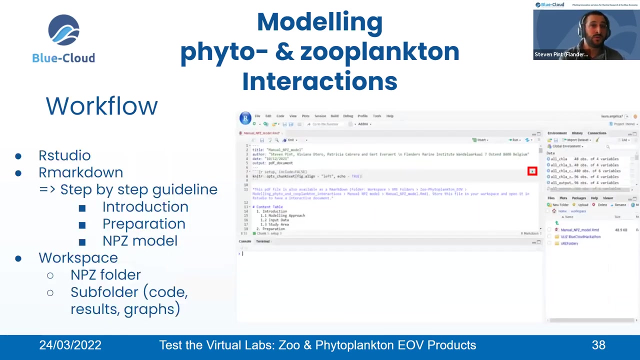 data sources and also you have links that take you to our data sources where you can download data for yourself or explore them, and we used data from lightwatch, flamish monitoring network, emotnet, and a model was built in an open source program, which is r, the workflow for you. how will you be using the model? it will be in our studio in in the vlab, and 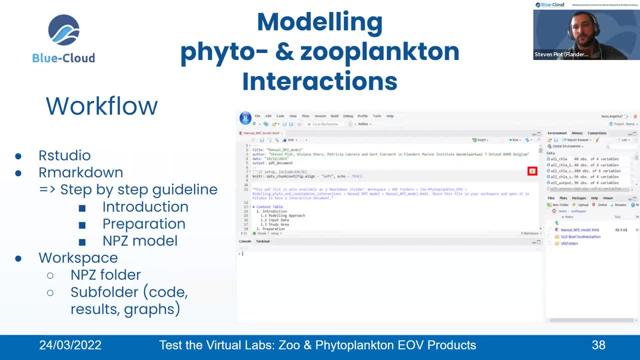 but first you have to do that as well, as you have to come together more frequently or confusingly as you can. and then in the vlab, and but first you have to integrate it into your model. First you have to download an R Markdown document from the VRE folder in the workspace. 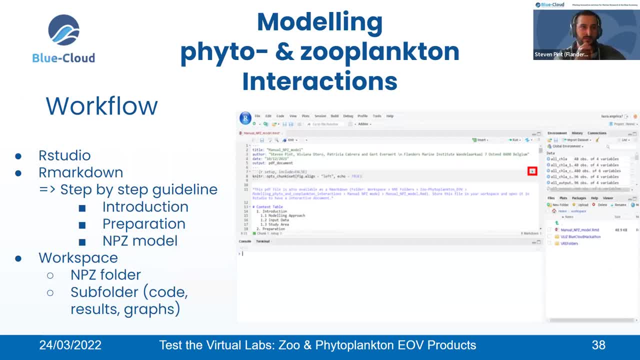 You have to then upload again to your personal workspace And the R Markdown is basically a step-by-step guideline that will guide you through the entire process of using the model. There is an introduction first about modeling approach, about the input data that is used. 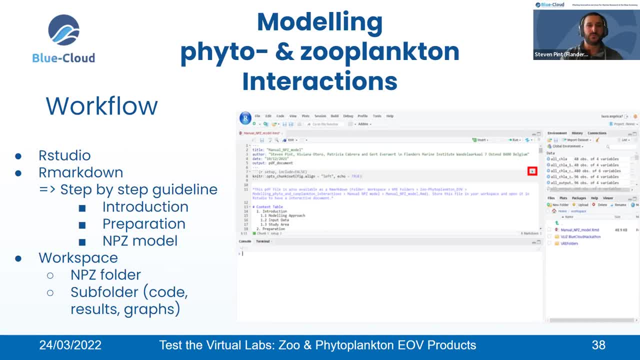 about the study area in the example that's given and also about the NPZ model, the nutrient phytoplankton and zooplankton model, and how you can use it, what you can adapt to it. You can twist and tweak a little bit around. 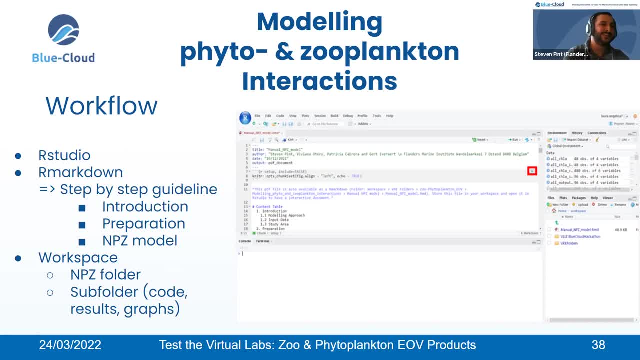 follow the guidelines and it should be working Further. it will also use your personal workspace. Our Markdown document will create a main folder called NPZ folder and some subfolders in there where it will copy and paste the input data, the code that you will be using. 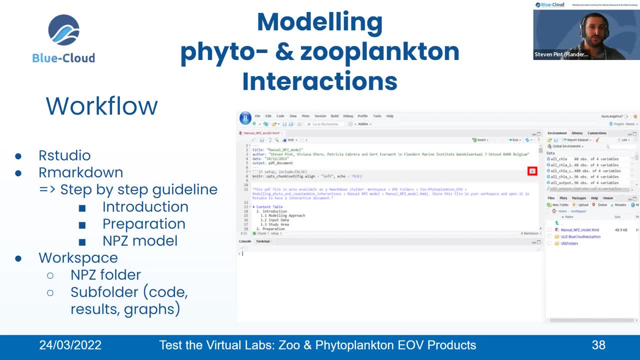 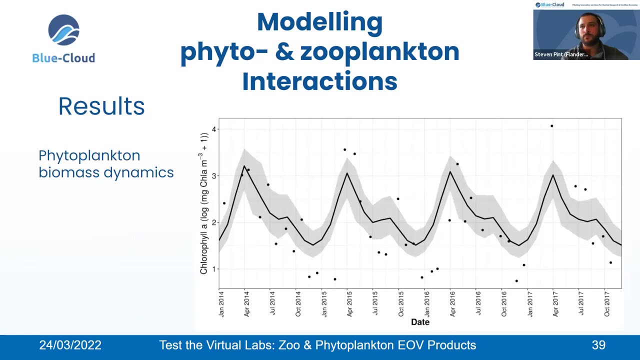 to also store your results in subfolders and also some visualizations in there. We did that so you don't have to change the working direction. so it's a little bit more user-friendly for you to use. Maybe most important for you to know. 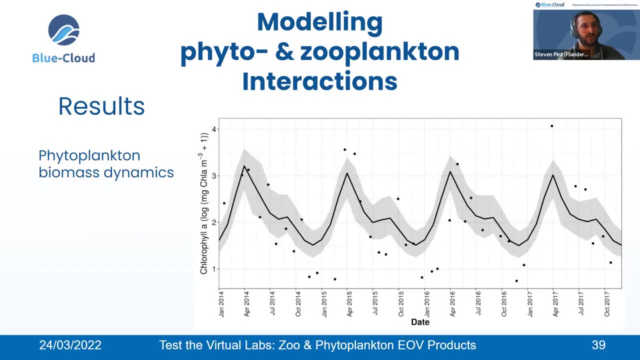 is: what can you get out of the model? so the results that you can get from the model is phytoplankton biomass dynamics, of course. So it's the biomass. It's the biomass that's expressed in chlorophyll A on the Y-axis. 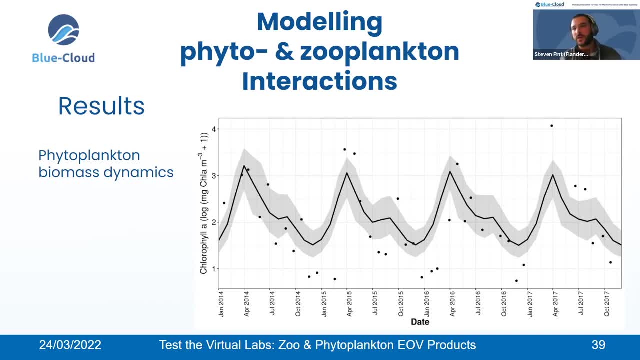 It's in a rock scale. It's important to know over time. So the solid black lines are the mean values that are simulated by the model, surrounded by its shaded area, which is the uncertainty of the model, and the black dots are field observations. 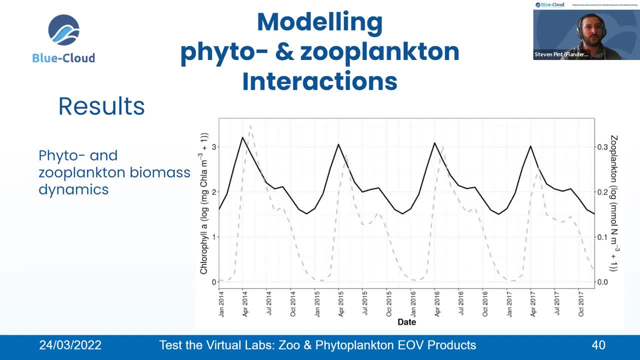 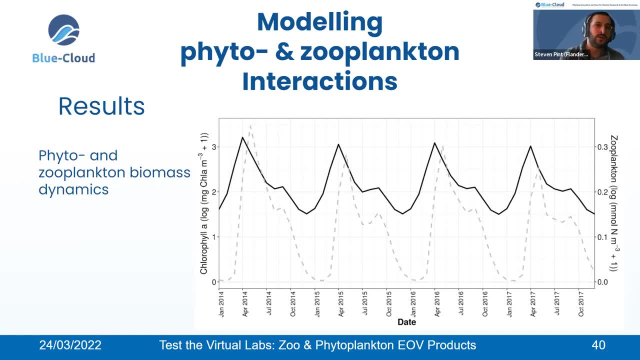 and the dashed line over time and how they interact with each other. And we can clearly see that if there is a peak in the black line, so in phytoplankton, it's followed with some time delay by a peak in the zooplankton, the dashed line. 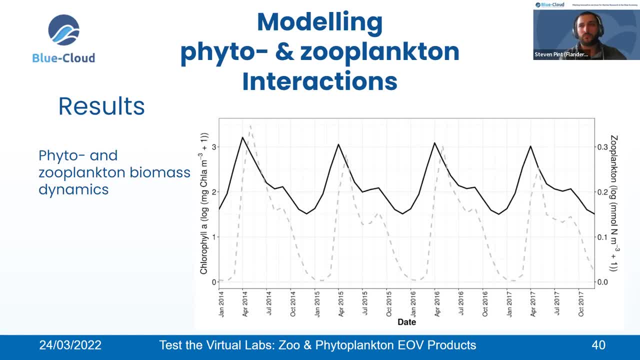 And that is actually a classic and textbook example of a prey-predator interaction, meaning that the zooplankton is actually grazing on the phytoplankton in the model. That's what we wanted, so that's good. Further, the relative contribution. 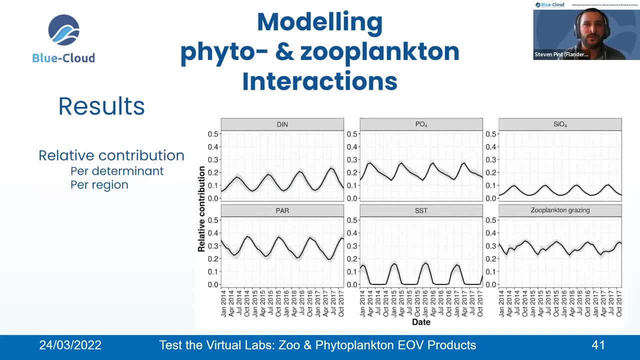 of all these factors that I told you in the introduction that are important for the phytoplankton biomass, In the top row we have the nutrients. So how important are the nutrients We have from left to right, nitrogen, phosphorus and silica? 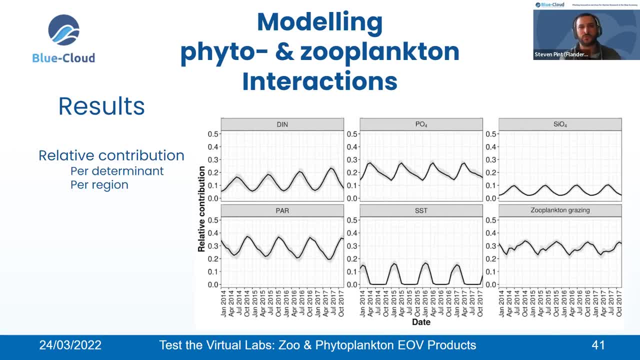 On the bottom row we have, from left to right, solar radiance expressed as photosynthetically active radiation, then sea surface temperature and zooplankton grazing. Here we have the relative contribution, which is the contribution of a factor divided by the contribution. 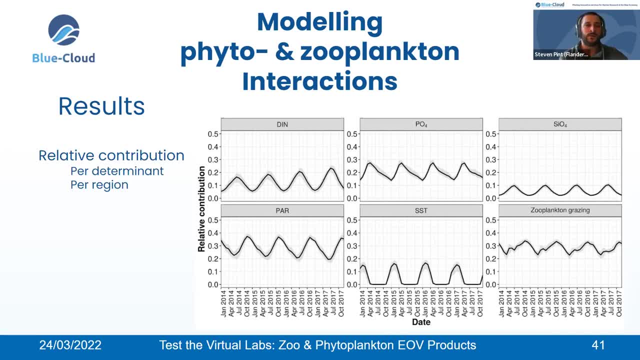 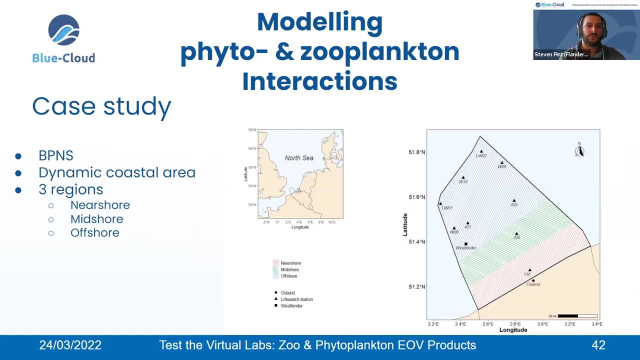 of all the factors together. over time It goes from zero to one, So one is if you combine them all. Maybe it's interesting if I show the results in a case study that we did. So we tested our model for the Belgian part of the North Sea. 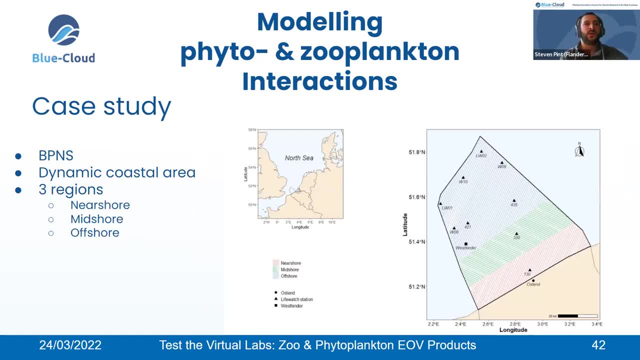 which is really dynamic and coastal area, and we divided it. it's in three regions: the near, mid and offshore region. In the offshore region, we pulled data from all the measuring stations together so we had sufficient amount of data to create these daily input data that we feed to our model. 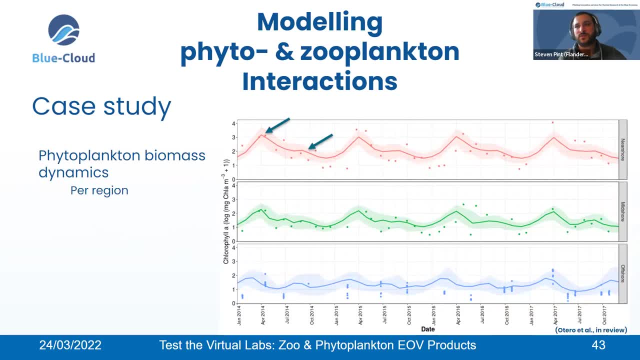 Then we have the phytoplankton biomass dynamics and we found that in the top graph, the midshore, there was the highest phytoplankton biomass located, followed by midshore and offshore region. The difference between the graphs doesn't seem much. 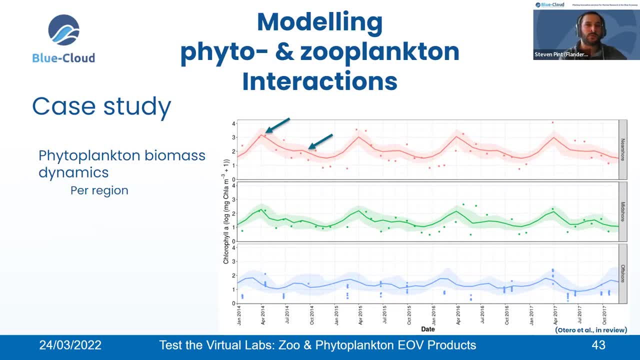 but remember we're working with a log scale, So actually we're talking about the difference of a tenfold, so it's quite a big difference. The two arrows indicate to the peaks in biomass, So we have one during spring bloom here at the Belgian coast. 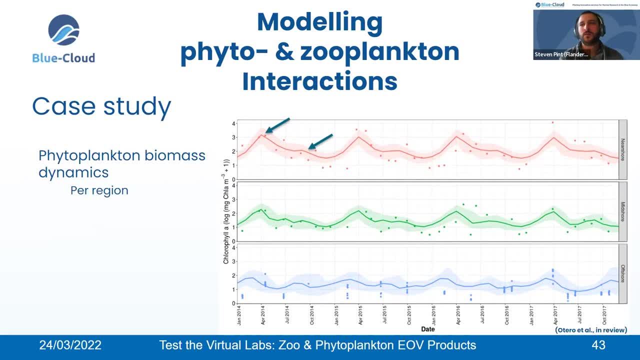 and one in autumn. It's a smaller peak, but it was remarkable that we found this, because before that there was a period where there was only one peak that was elongated in the Belgian part of the North Sea. so this could indicate that the Belgian part of the North Sea 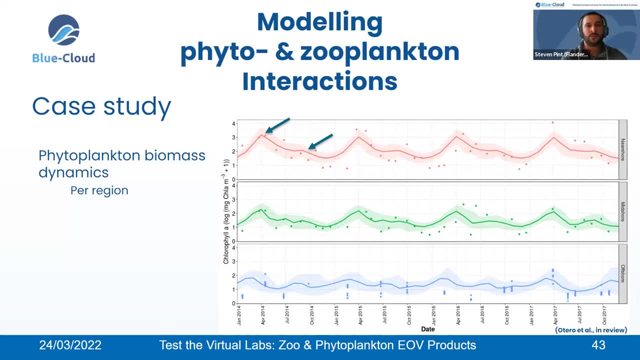 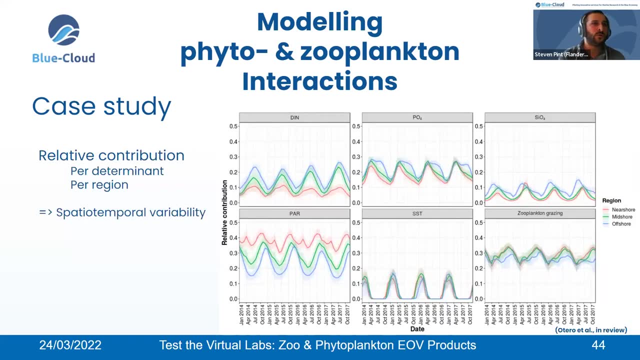 switched back to peak annual cycle So it was interesting for us to find Further. we have the relative contribution. We combine them here also for all the regions together. So in red we have the new shore, green, midshore and blue. 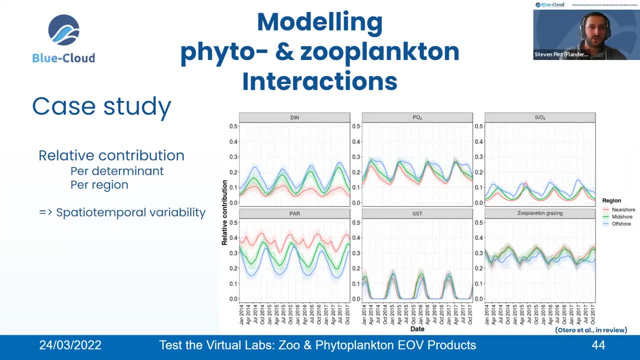 So the offshore region And, as you can see, there is quite a seasonal cycle, So there is a temporal variability. for the nutrients in the top layer, We see that they are most important and contributing the most during springtime and after springtime, after the spring bloom. 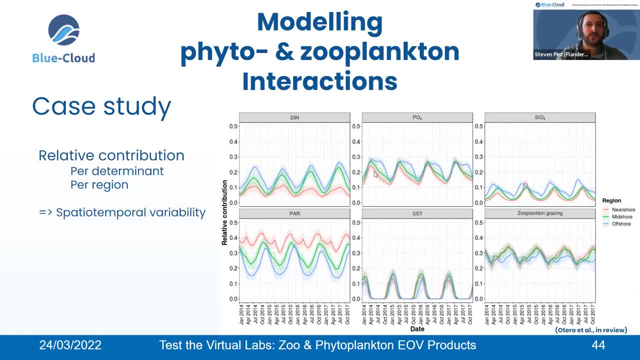 There is a difference. The phosphorus is a little bit earlier playing an important role than the other two nutrients, the nitrogen and silica. Solar irradiance and sea surface temperature play a more important role during the autumn and wintertime, And zooplankton grazing is more in the summer and autumn after. 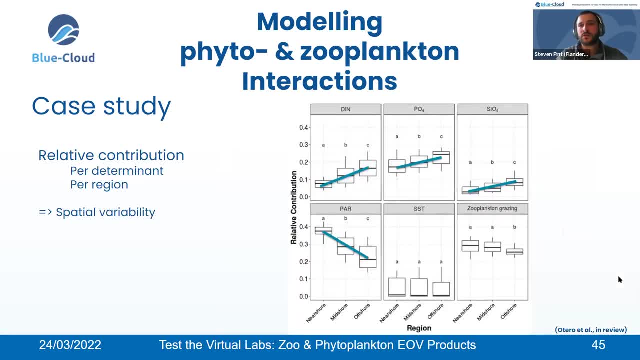 But there is also quite some spatial variation and it's also interesting to see that we have found a clear difference and a clear near offshore gradient for the nutrients being more limited in autumn and wintertime, So we can see that there is a change in the amount of nitrogen. 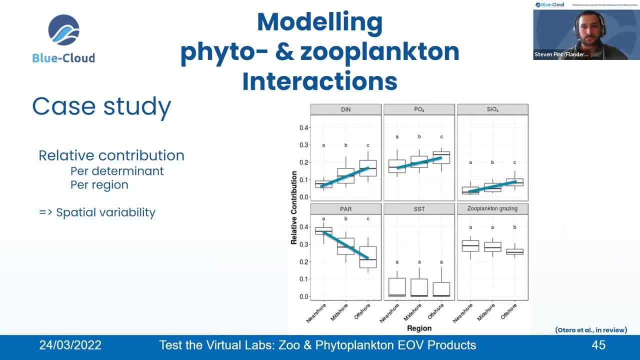 in the offshore region. This is demonstrated here in the top row. That can be due to the fact that we have riverine input from the river Scheldt and it gets depleted towards the offshore region, meaning that there is less nutrients available for phytoplankton. 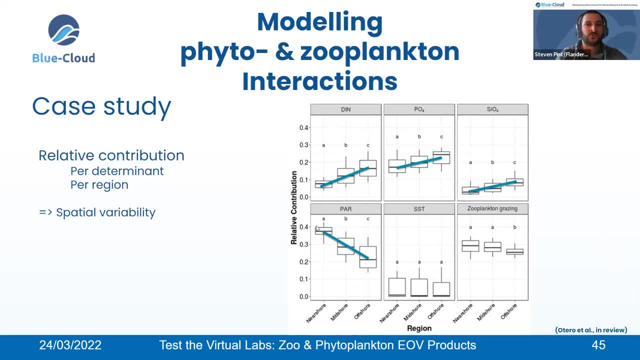 in the offshore region, We found the opposite to be true, for the solar irradiance being more limiting or having a higher contribution to the change in phytoplankton. In fact, the phytoplankton biomass in the near shore region that can be due to the high turbidity, blocking sunlight that's needed. 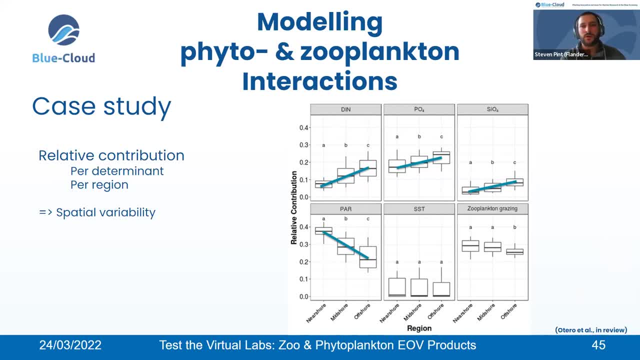 for the photosynthesis. For sea surface temperature, we didn't really find a difference between the regions, and the zooplankton grazing was a little bit lower or the pressure was lower in the offshore region. So that was our case study, that we did. 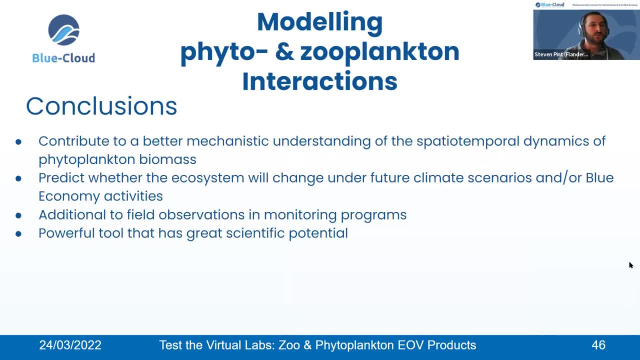 We were very happy with the results And so, to conclude, we guess the model contributes to better understanding of spatial temporal dynamics of phytoplankton biomass, and also its determinants can be used to predict whether or not an ecosystem will change under future climate scenarios. 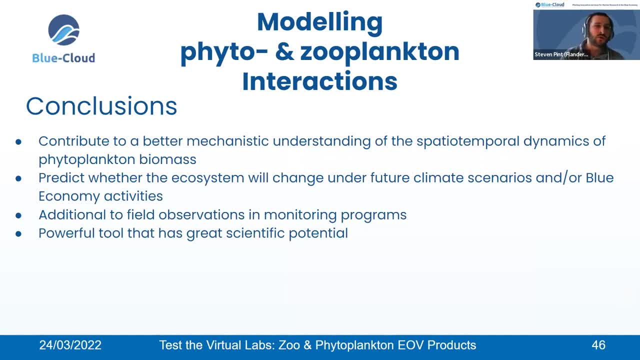 and or with blue economic activities. The model can be used additionally to field observations in monitoring programs to fill in data gaps And, of course, in general. the blue cloud with its VLABs is a powerful tool that has great scientific potentials. Thank you. 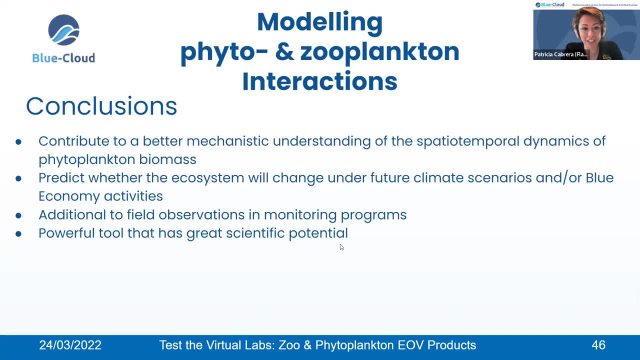 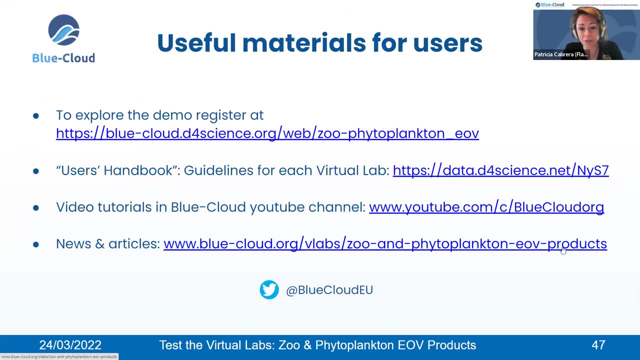 In your screen, Steven. I will just have a little wrap up slide before we jump into the Q&A that will be moderated by Sarah and that I see already some questions there. But just a few words and just to put all this scientific research into the blue cloud context. 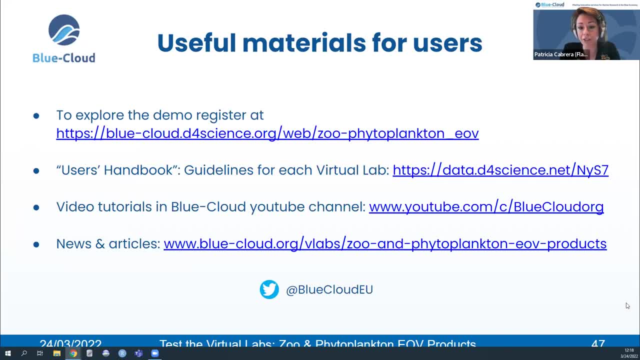 So you can see that there has been very diverse products developed within this demonstrator. We have products that are using machine learning techniques and neural networks. We are covering zooplankton, phytoplankton species in the open ocean and also in the coastal ecosystem. 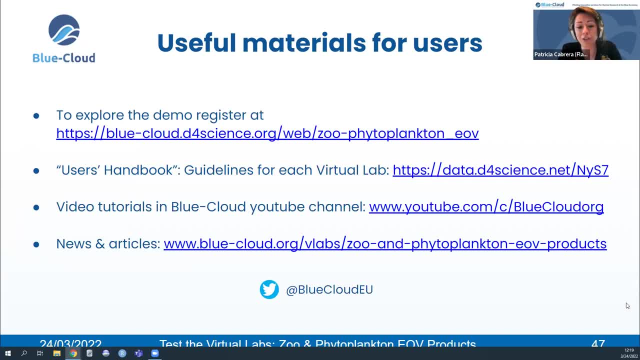 So, thank you, Thank you. So what is important is that some of these methodologies may need some specific knowledge, such as, for instance, you may think that you need to know Julia programming to use the zooplankton EOV product, or that you may need to know a lot. 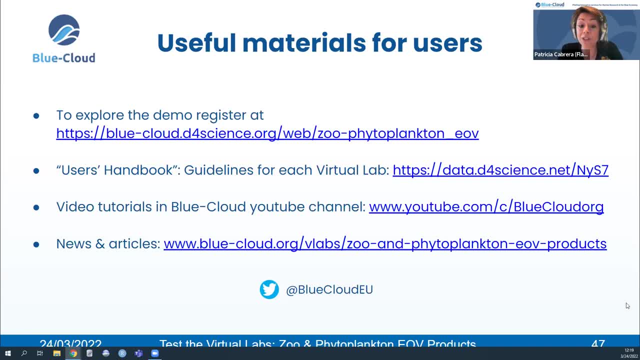 about the ecosystem model that Steven just presented, But actually the reason is that everything is presented in a way that users- and we are targeting a wide variety of users- can actually test these and build further on these and run the scripts with not a lot of skills needed. 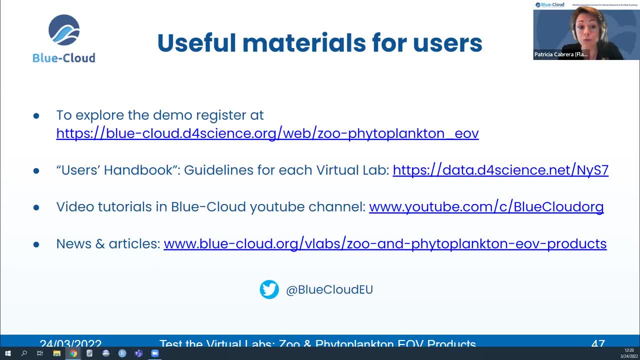 So, therefore, we really invite anyone to go and use it, to explore and hear about it. Thank you. Here I give you some of the resources that you can use. So first of all, that is the link that I think it has been shared already. 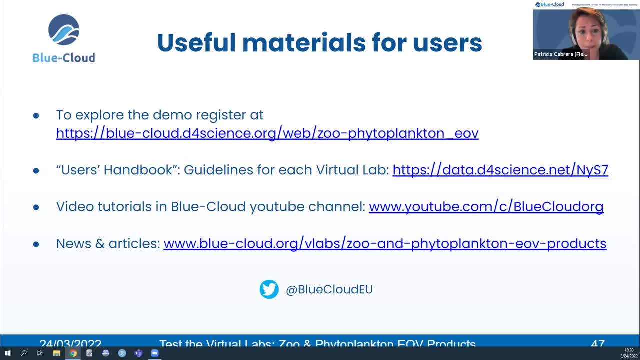 in the chat to access to the demonstrator, to the VLAB. Then we have another link that takes you to the handbook, the user's handbook, which contains all the very specific information about our demo, but all the demos As well. there is the YouTube channel for Blue Cloud, where. 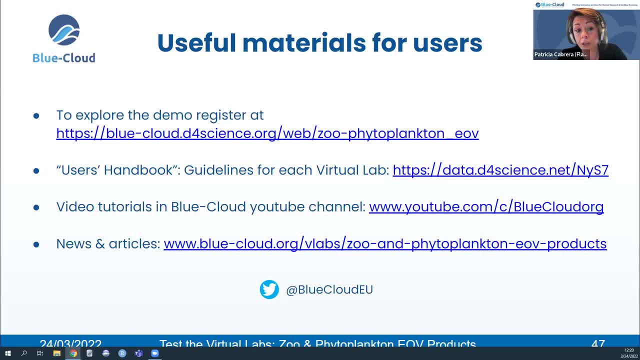 there is plenty of tutorials, with even live demos on how to find all this documentation that we have put a lot of efforts on really explain well for users And as well. you can keep an eye on Twitter, as we keep having a lot of communications about what is going on in the project. 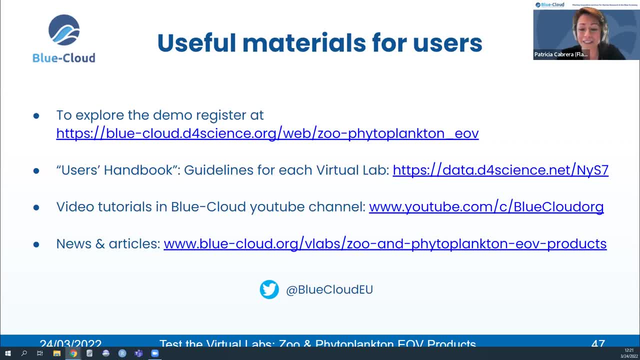 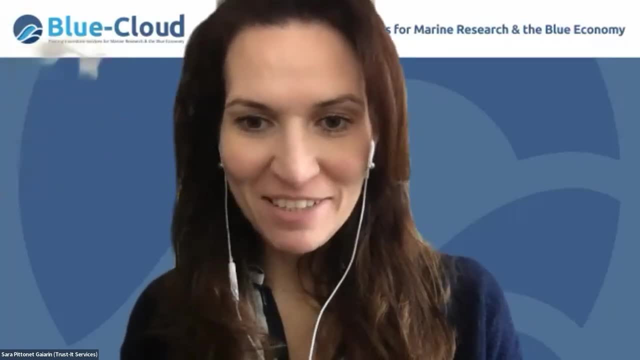 So, yeah, that's all for the materials and resources, And I think it's now the time to jump into the Q&A. So, yeah, thank you Sara, Thank you very much Patricia, And thank you all for presenting today. Yes, the question and answer chat is pretty active, I must say. 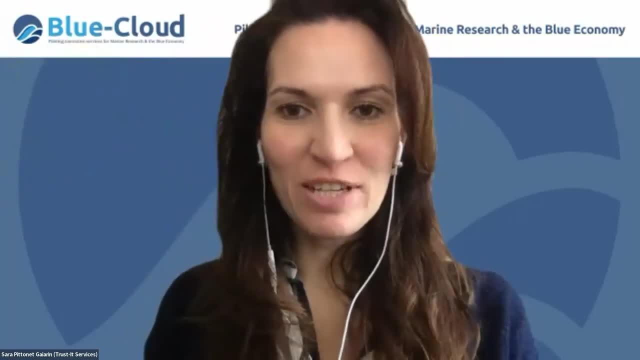 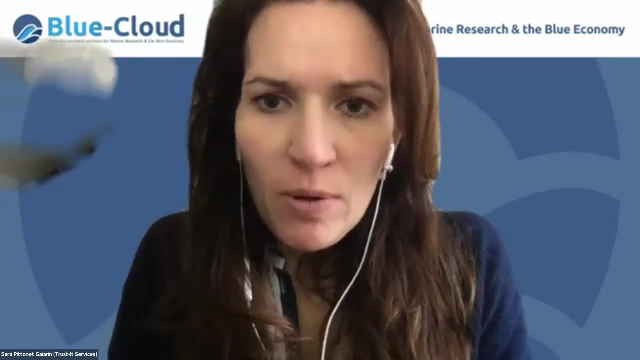 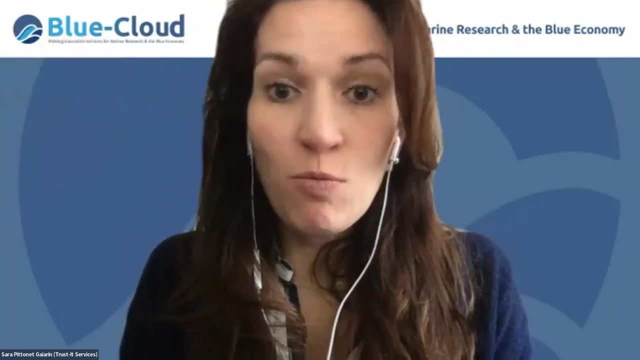 So I think this is a good sign of the interest. Maybe I'll pick up those that are still unresponded. So there is one question for both, or I presume I mean for all speakers. The images that are produced are wonderful. 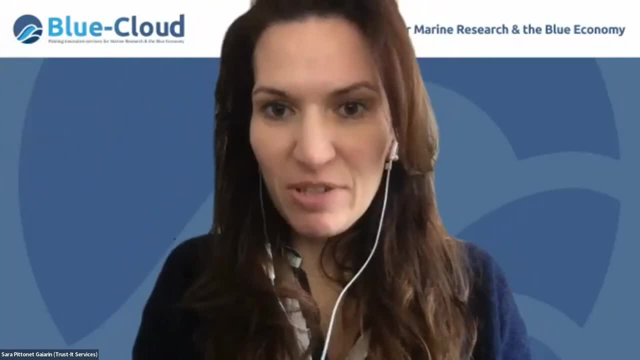 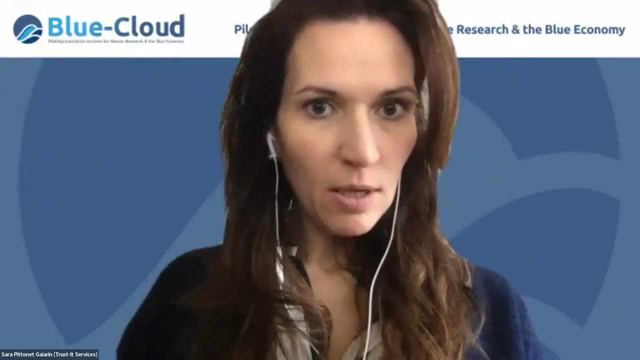 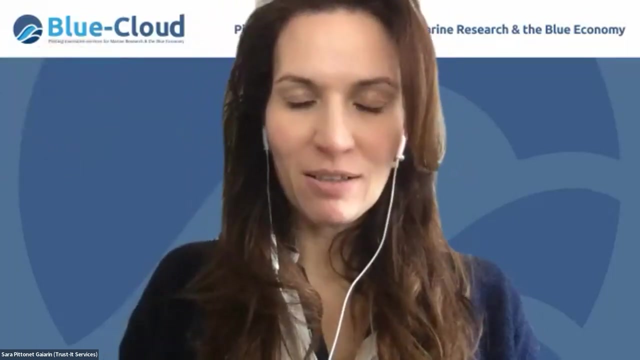 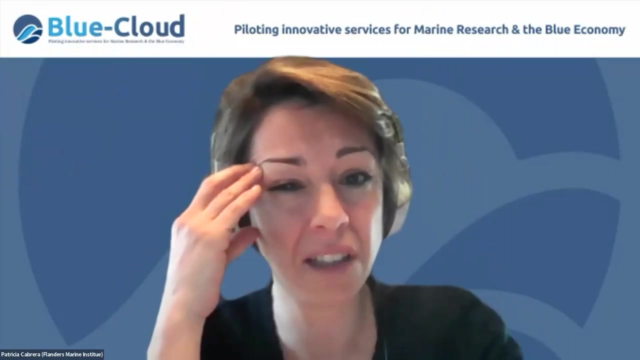 However, it is also important to get some actual statistical results. Is it possible to do some statistics too? I think the question was raised when Charles, I believe when Charles was presenting, but I think any of you can reply. I think, at least, Stephen, isn't it in your script that at the very 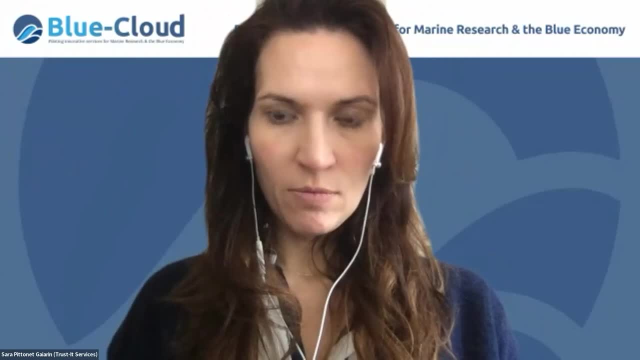 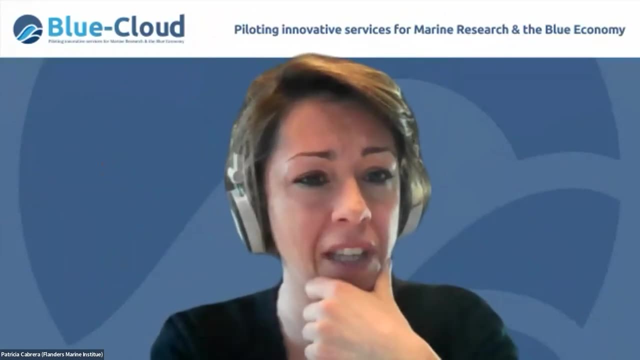 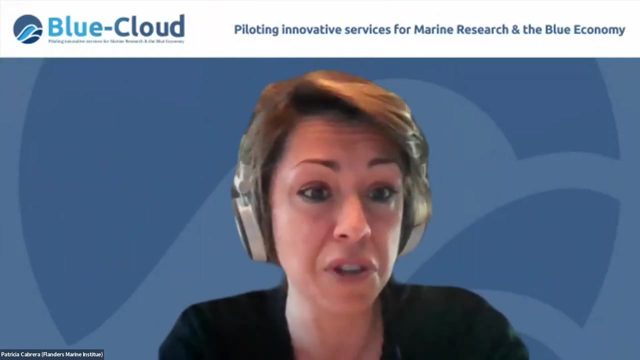 beginning. there is a part that it's really focusing on some visualizations to really understand the patterns on the data. And for sure as well for Charles I think there is with the CPR data. there is something done before, So maybe at least. yes, Stephen, you would like to add anything? 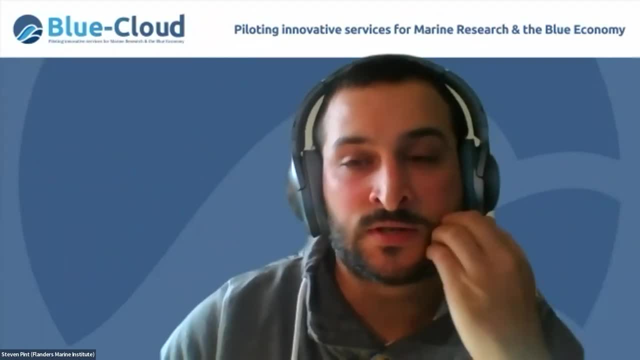 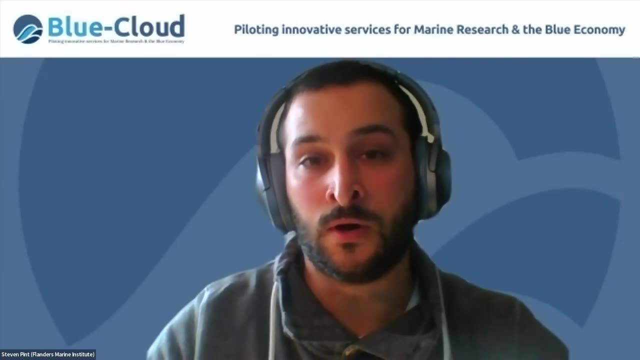 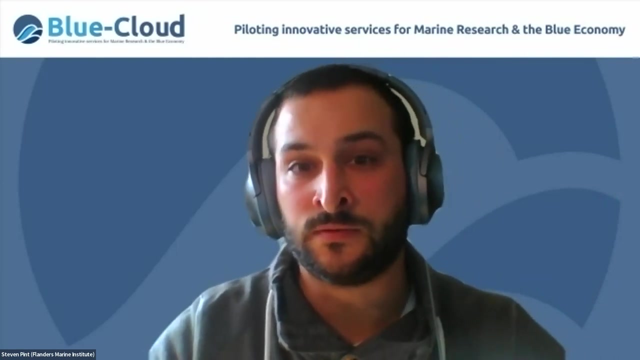 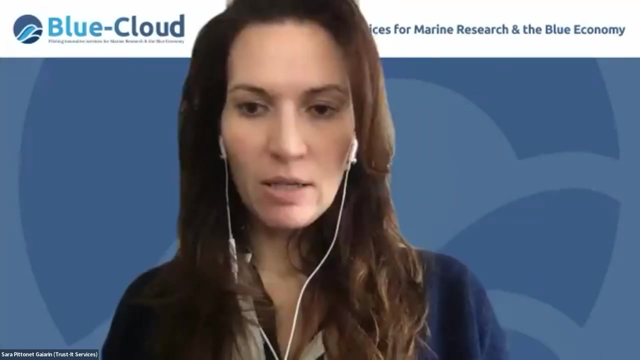 For me. for my part, there is really the potential to use statistical tools and tests on our results. I already used them in the box plots, So to see or illustrate a significant difference between the regions. So, yeah, Okay, great. 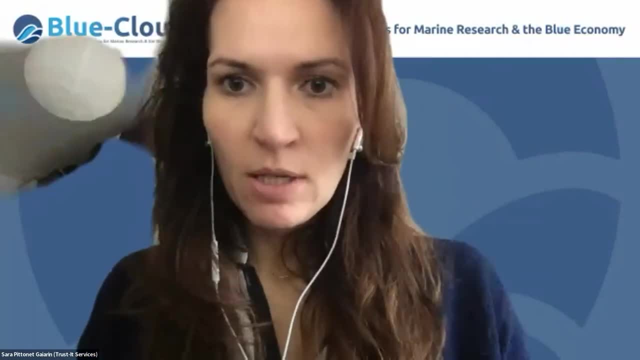 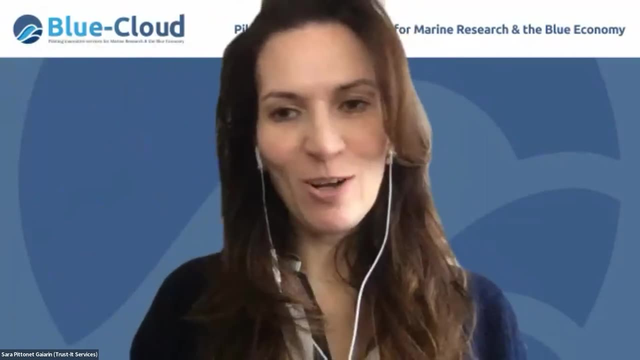 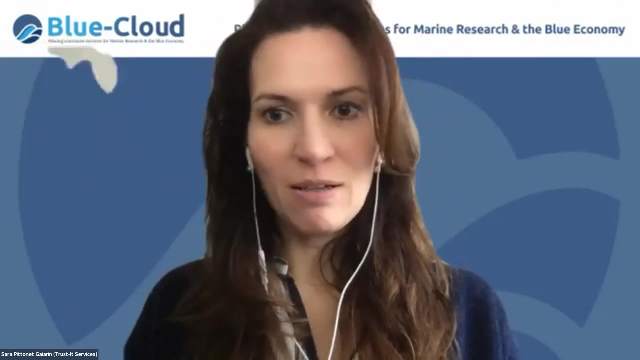 And then we have another one. Oh yes, I mean, it's not a question. I mean I think it's the last of a thread of exchanges between Veronique and colleagues at Blue Cloud, And thanks. So, Veronique, I understand you're part of the team who is working with Jericho. 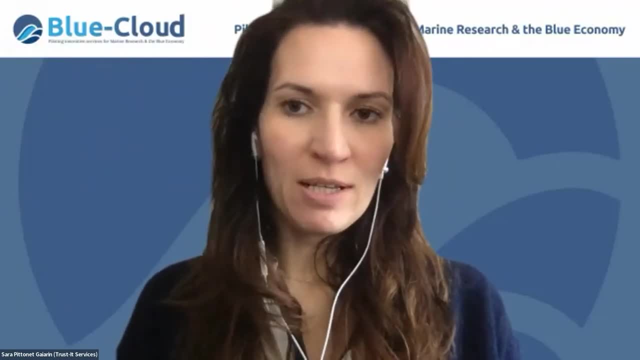 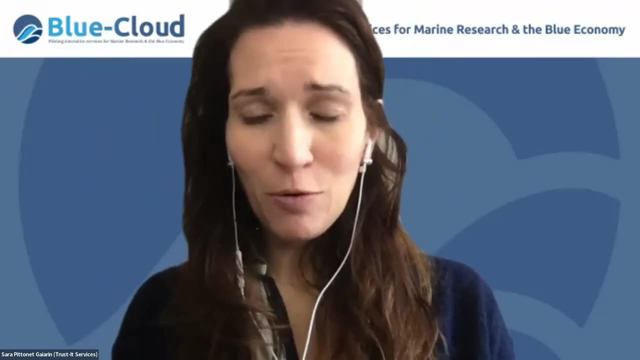 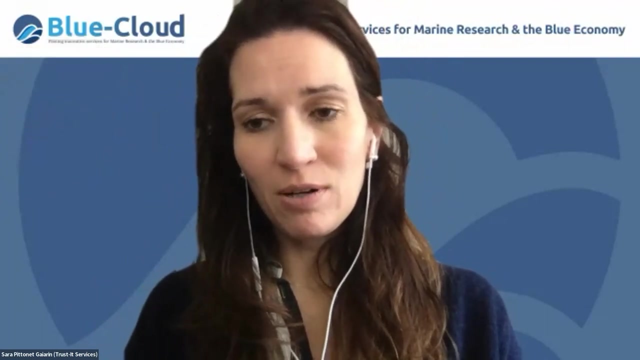 Yeah, on via- I mean cDataNet, and through them via Blue Cloud. So the only thing I can say is that we have started a very interesting collaboration with Jericho as well. In one of the cases where custom materials have been produced, we have 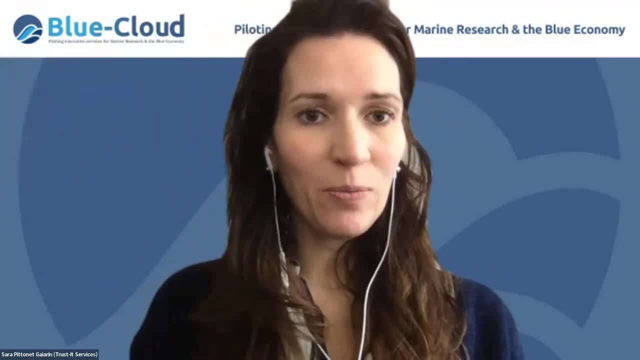 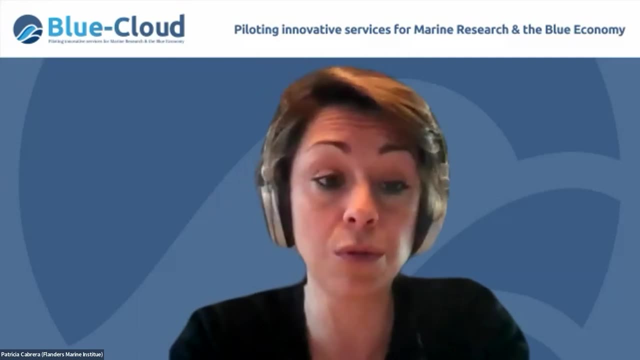 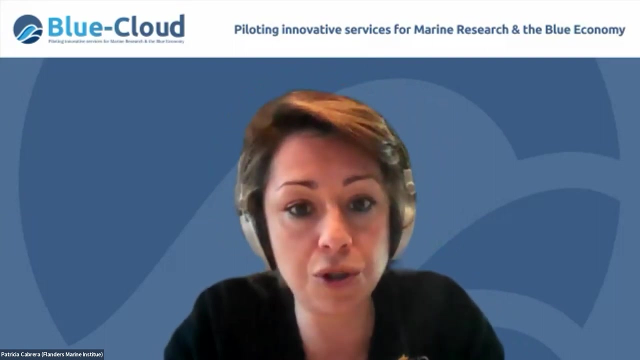 a virtual lab being implemented. So yes, Patricia, If I can add here, I think for us It was really interesting to produce global, global products, because in this way the idea was that we want to show how we can do harmonization. 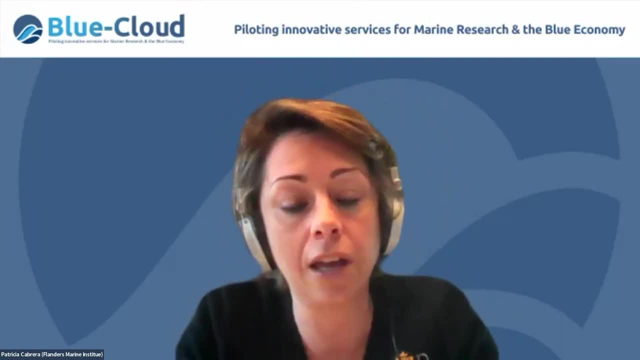 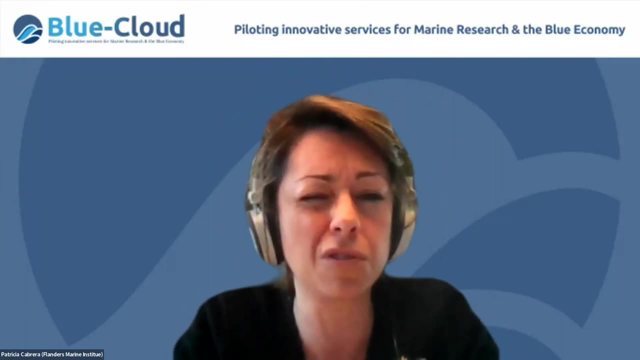 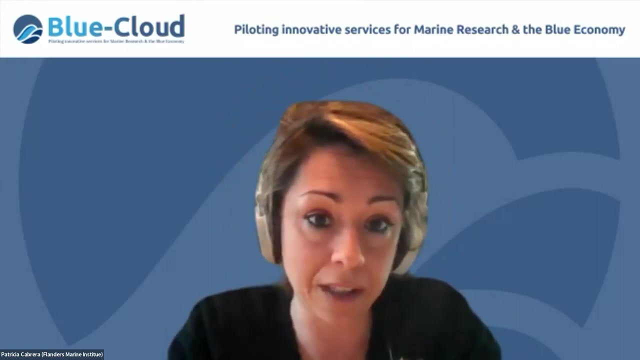 of different data types and, as well, to look at really global regions. So it is really like, as you see, the other products, not the phytoplankton one- it is focusing more on a smaller scale, but always with the idea that we want to really take extend this to global when it is possible. 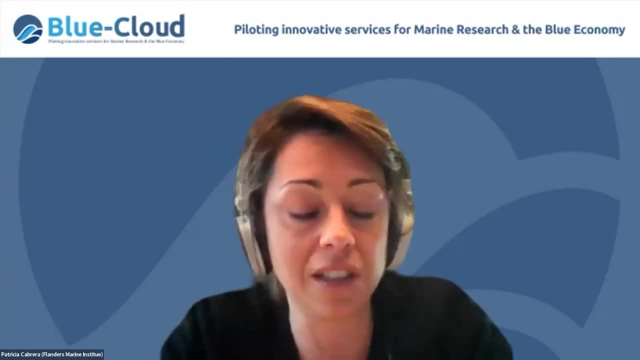 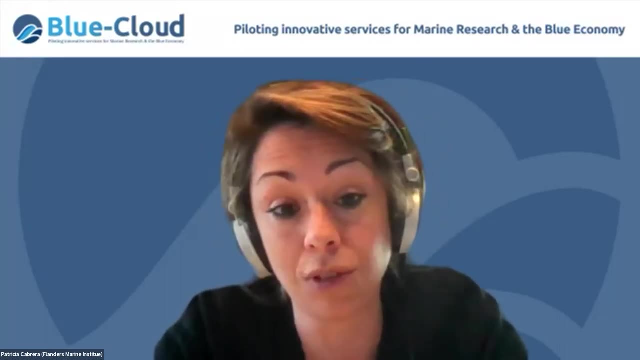 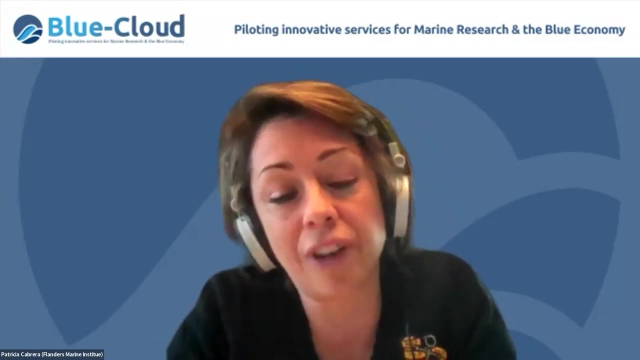 just to look at, Yeah, what are the capabilities that we can do? So, indeed, is something that we need to look into how to really translate these to the, to the societal challenges and the European directives, And that is why we want to provide these in a user-friendly way. 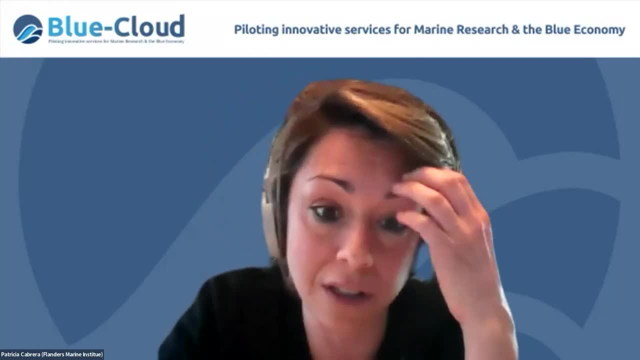 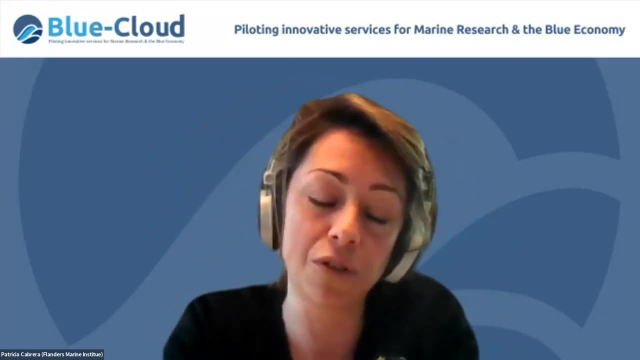 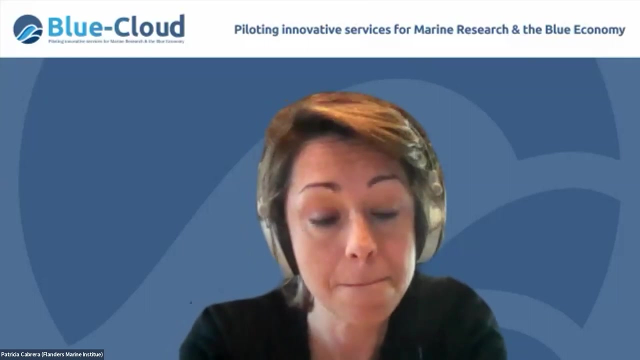 So actually it can be really used and translated to a very different non-scientific public. So yeah, but I understand your point of looking at also regionally, which indeed is done in Jericho. Thanks, Patricia, Yes indeed. 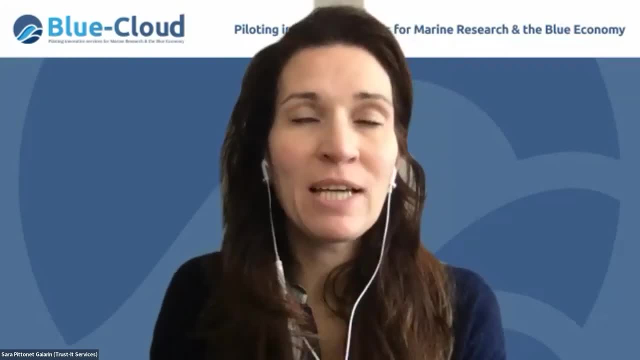 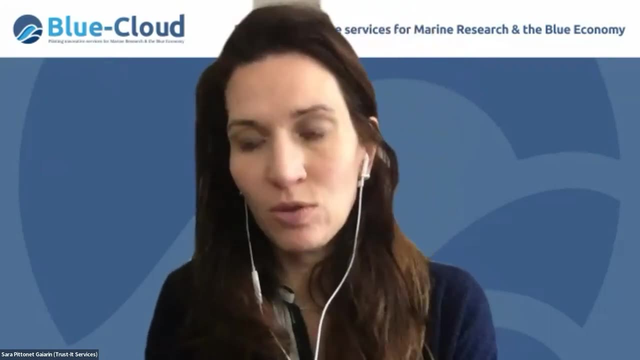 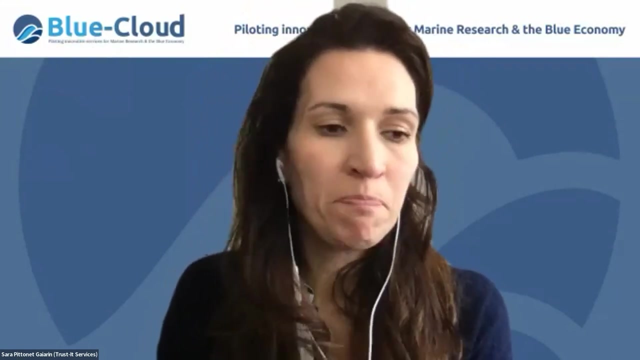 There are many opportunities still to exploit, and with that I mean- I reiterate what Patricia invited you to do- to follow the materials: sign up to The virtual lab. in case you haven't yet, There are some even social media functionality that allow you to get in. 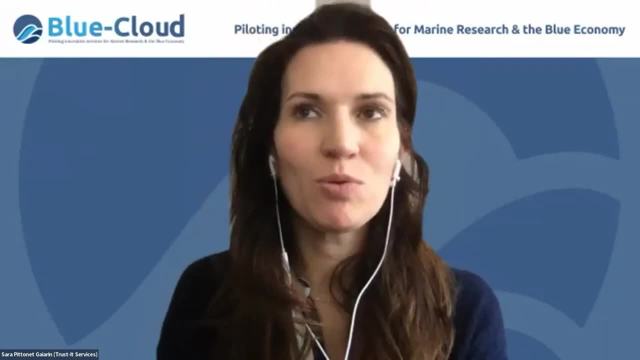 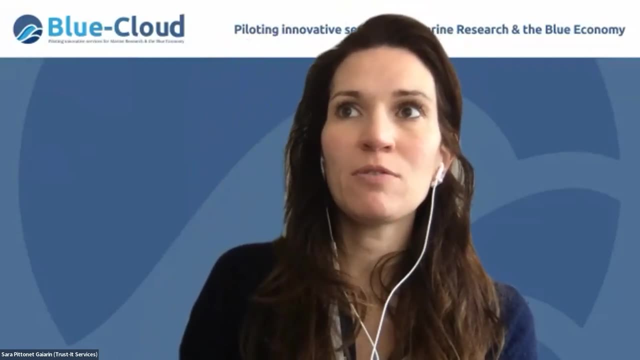 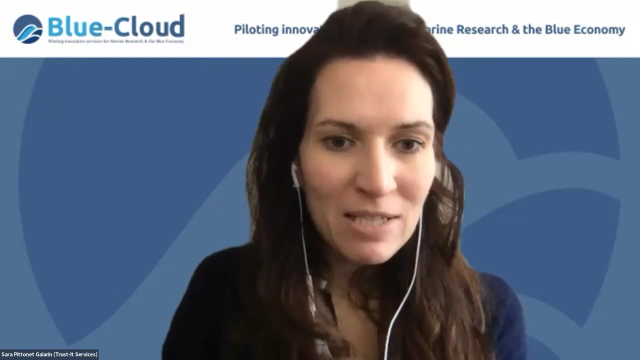 touch with the owners of the virtual labs, or I mean right blue cloud, and we pointed to the appropriate persons. in case you're new and you simply want to understand if we can fit your research case And with that, unless I see, Patricia, you? Yeah, I see. 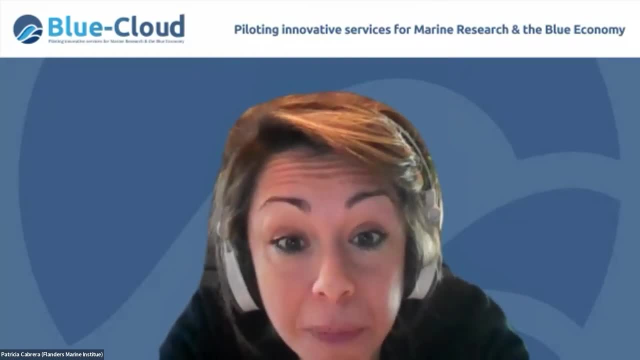 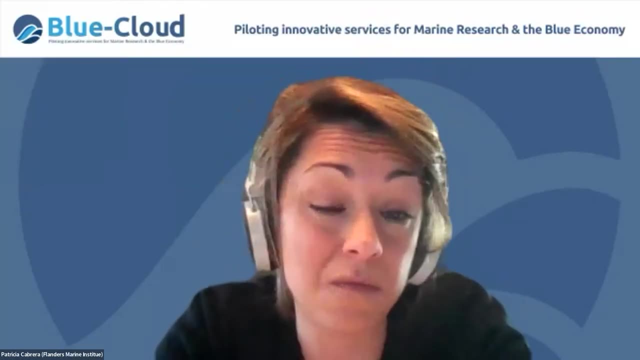 There is a question for love, Laura. that has been answered, but maybe I can add, because yeah, the question was: if for the, I guess she was meaning for the diva and deep product, the zooplankton product, which aims to use heterogeneous data. 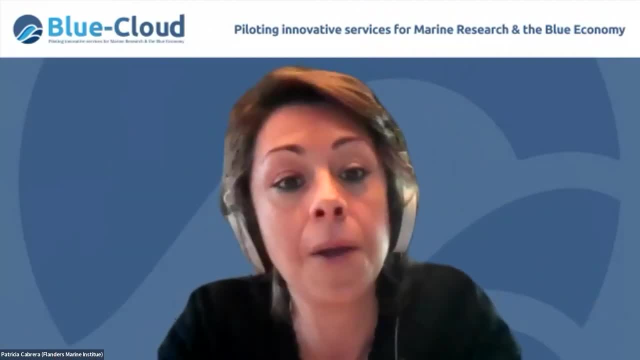 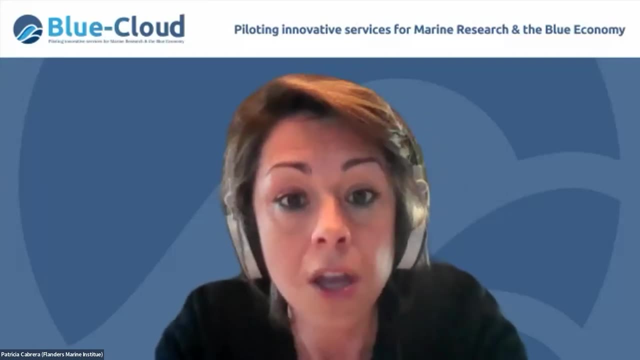 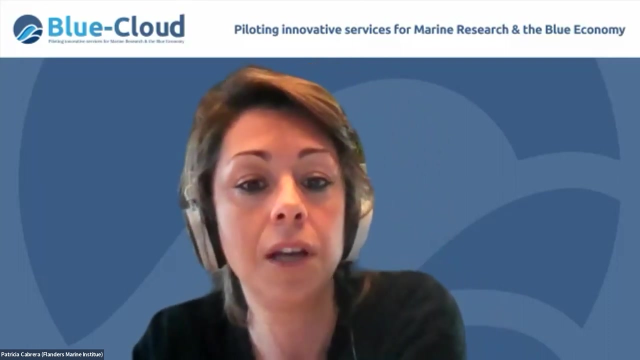 to have a better understanding of this heterogeneous data. So she asked if we have used the data from the Black Sea region, which is not very generous. So actually, the idea is that We have produced it. We are showcasing how to apply this model or any of these other different 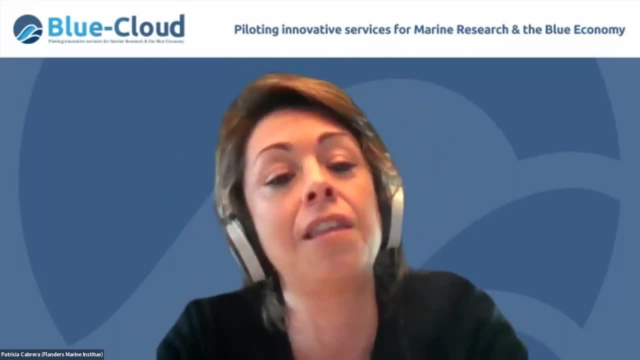 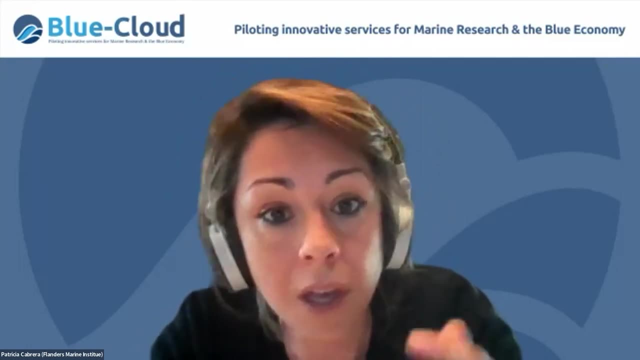 methods with some specific data, But the idea is that now everyone can go there and use it. So, for instance, if you think this model is really applicable with plankton data from the Black Sea, this is something that you can always take, everything. 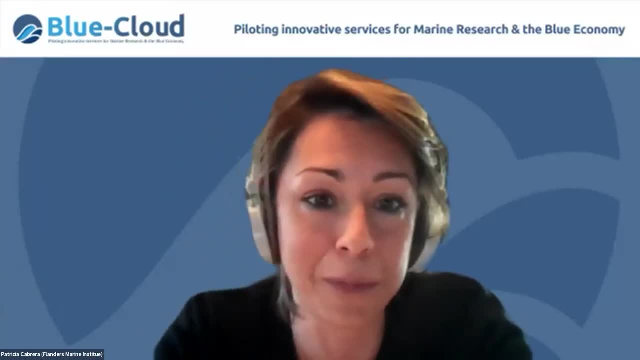 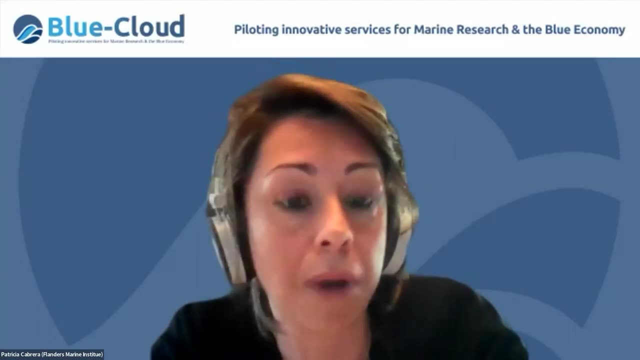 We made sure that everything is as fair as possible- Fair principles, I mean- so you're able to really reproduce this Method and have your product for blacks- Black Sea plankton, for instance. So that's just my addition, that now our idea is not to keep working on. 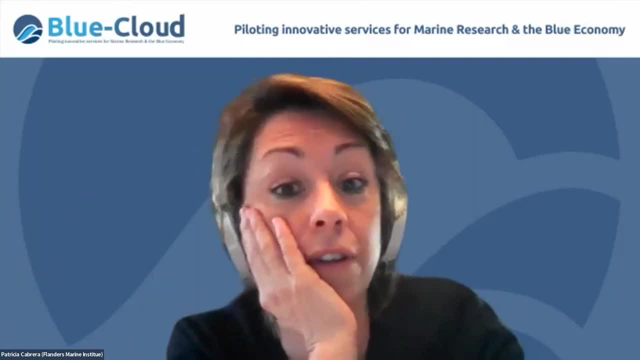 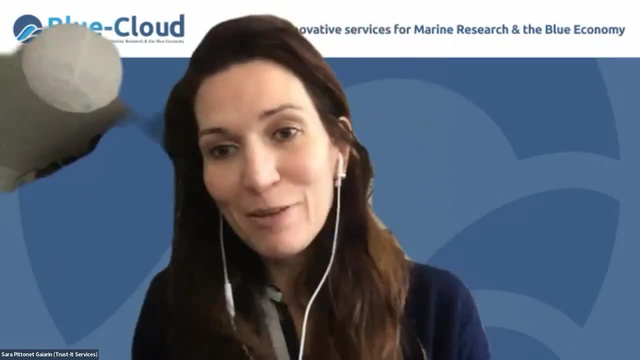 this, but actually users to work on it with their ideas and data. Yes, I mean just to be clear. we had the hackathon last month, but we don't need an hackathon to have users. It's just so really, we were entering now. 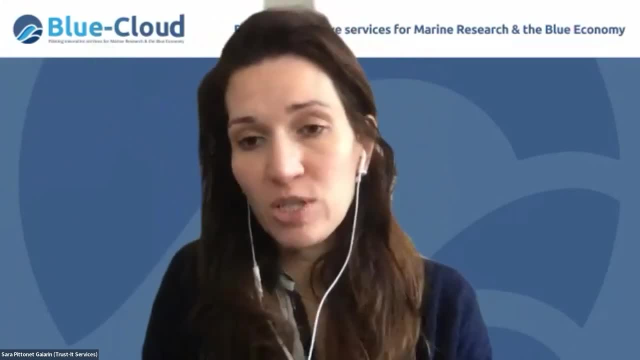 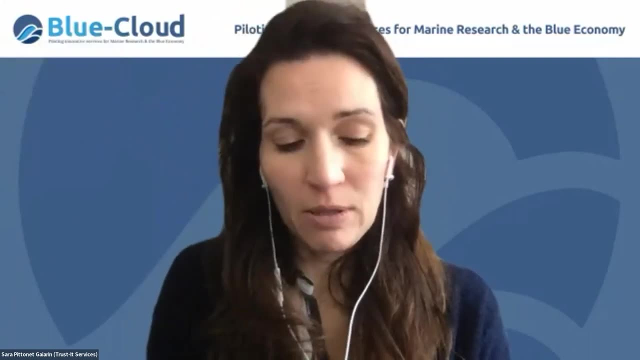 Let's say the concluding phase, I would say, of the project, which is the one dedicated to User testing. So we have effort to support you and to customize, as I mean a little bit or as far as the tools allow, I mean the software and the products to your, to specific needs, or at least 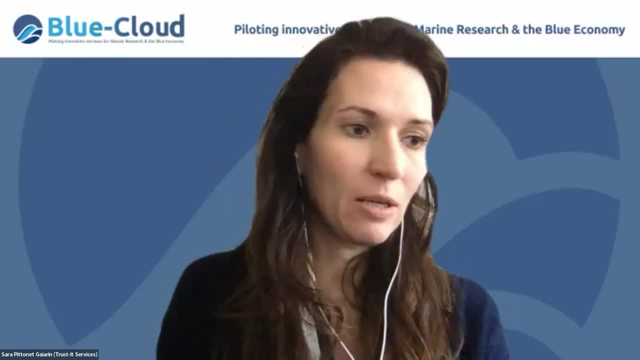 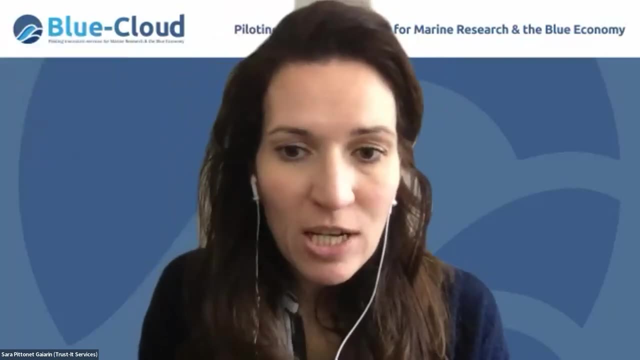 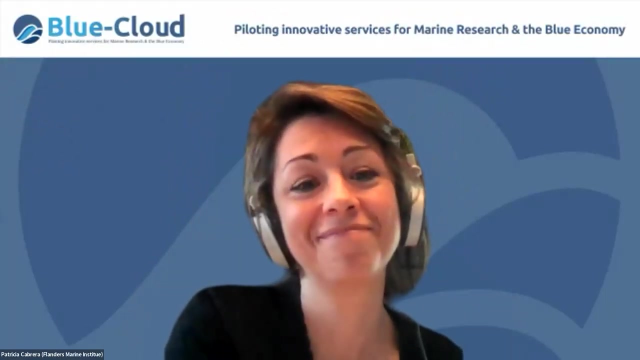 I mean, and this age, what is the bandwidth to really help you adapt these solutions? And since we have few minutes, I suggest if you can turn on. we have a very light survey and it's a One question actually that we would like you to help us with, and this relates 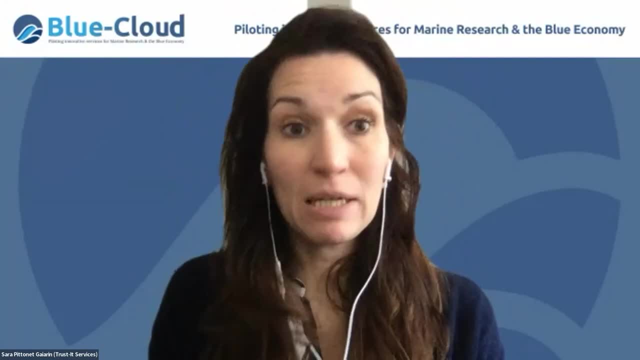 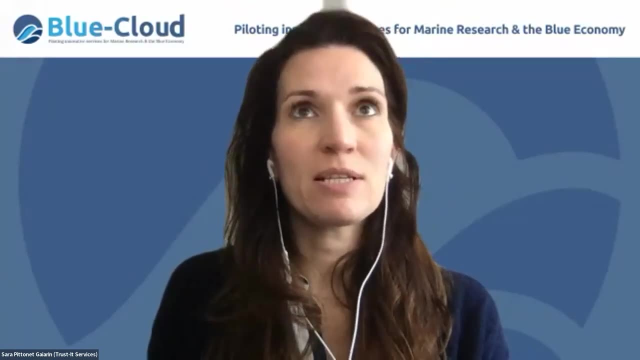 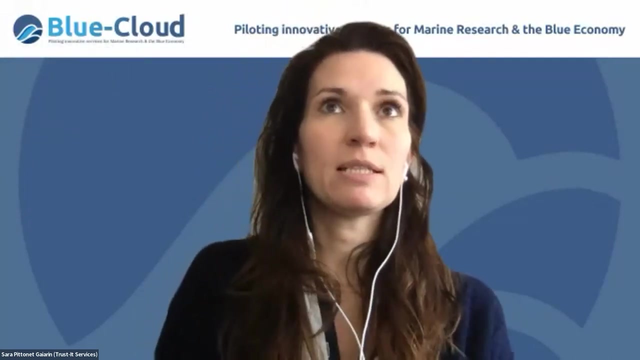 to say, the sustainability of this model. So we need your help to understand for how long would you like the services, in particularly the notebooks, to be available in this virtual environments? So you should see the tab open on your screen. Just feel free to take the option that you prefer. 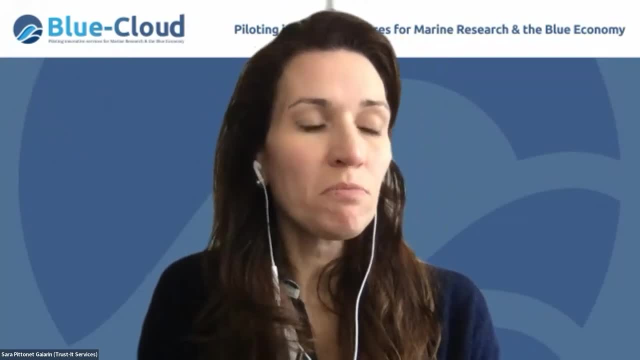 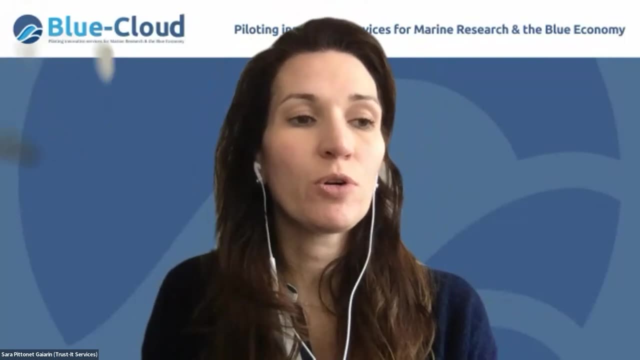 We are doing So, as I mentioned, because we we have still a few- I mean few- months ahead, but we are working to understand what type of support we should give to newcomers, And so even understanding time frames and how long ideally you would like this to be. 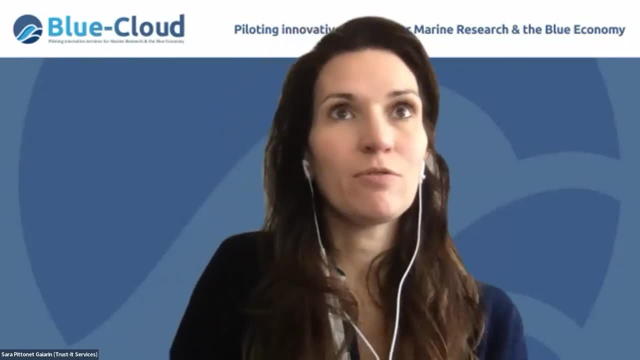 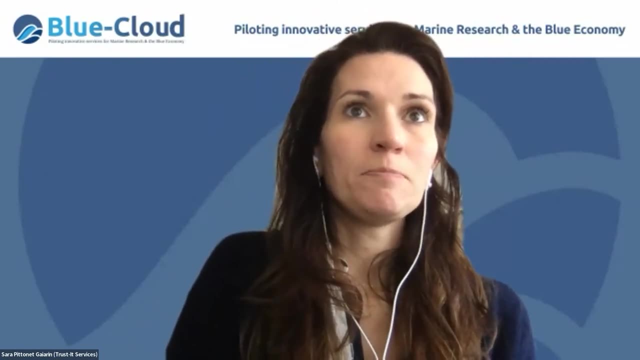 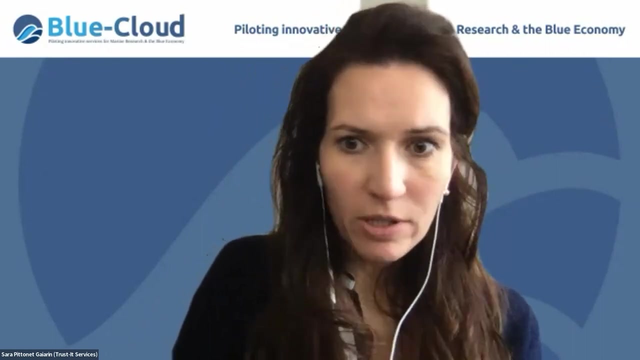 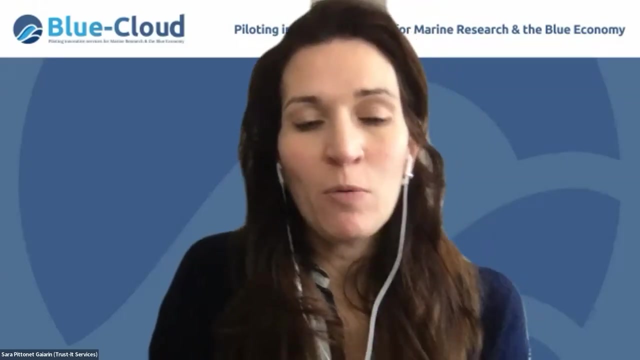 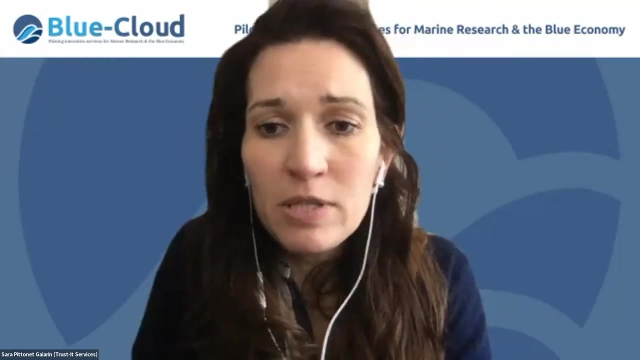 Running. It's fundamental for understanding Sustainability aspects of the project. I hope I think for there. are you receiving answers right? Yes, 60% of the people have replied as of the moment. Great, And maybe while we wait another few to fill in the survey, unless any of the 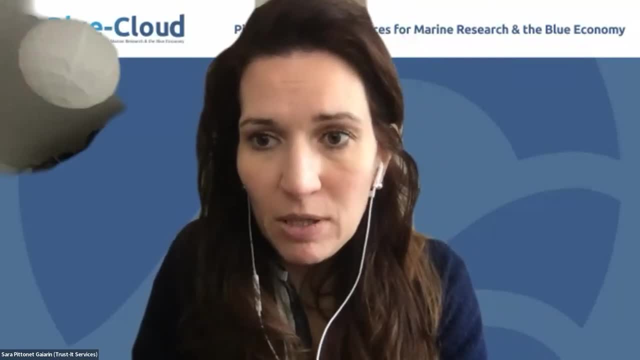 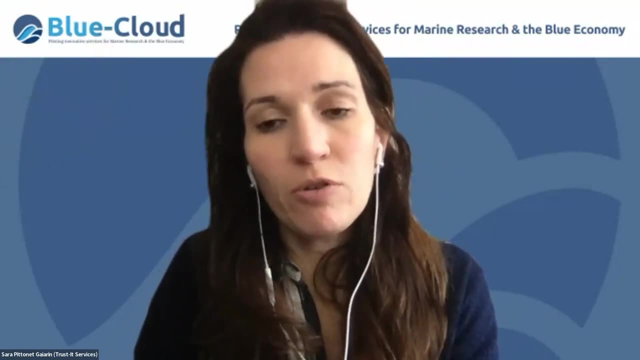 speakers wants to pick up one of the questions received. it might be of particular interest And, by the way, I can say that you are going to retain these and use them for a frequently asked section that we can have on the website and on the 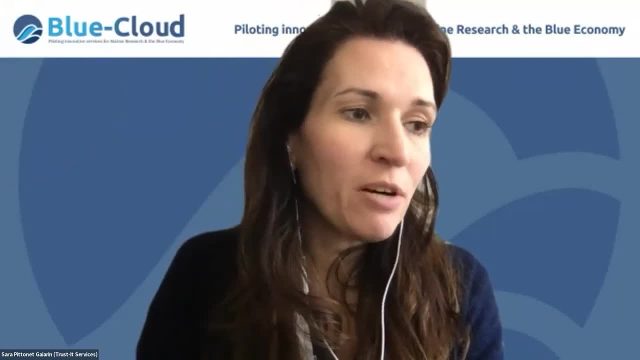 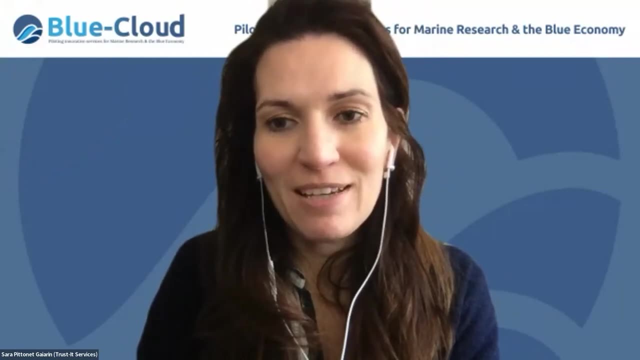 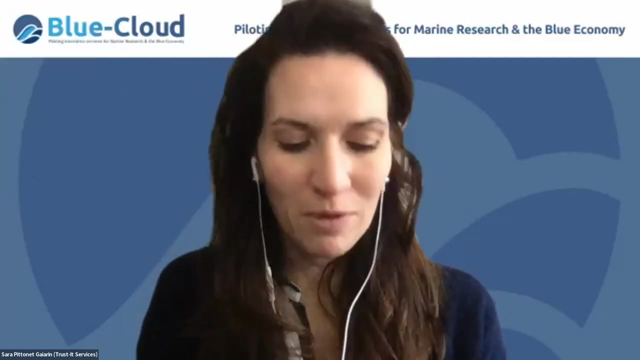 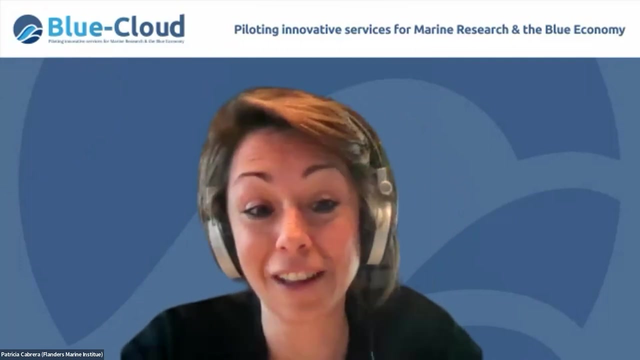 virtual lab page. Patricia, can you share any insights from the hackathon that might be of interest for participants today, Some case and questions that you got that can help Our listeners today? Yes, actually we had quite a lot of participants that joined the challenge. 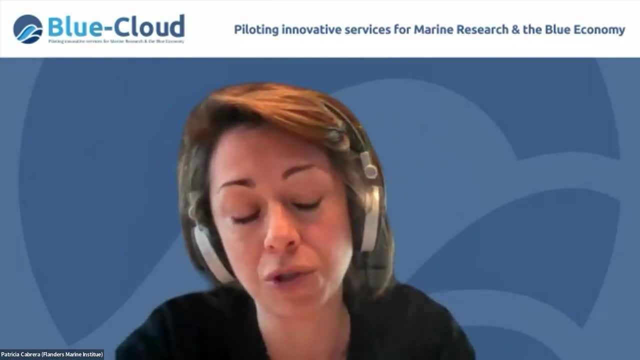 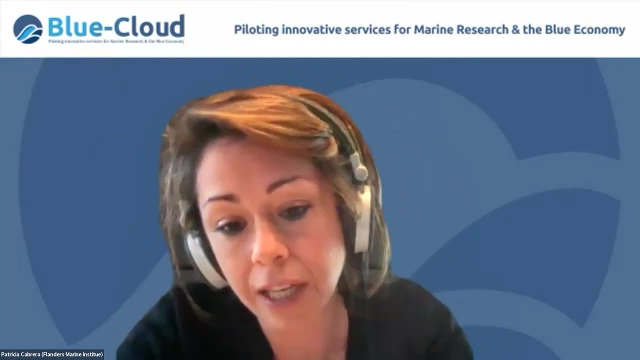 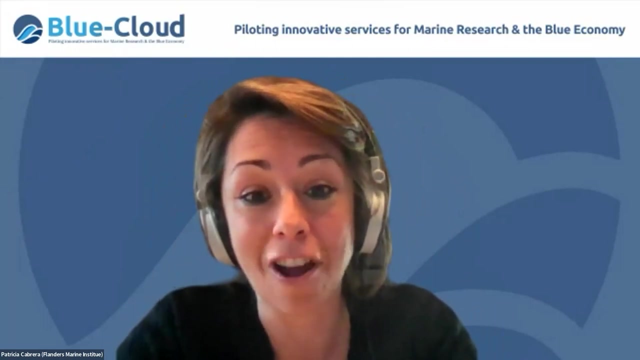 that we were proposing in the theme of our demonstrator and demonstrator to which also deals with plankton, but genomics, and there was a specifically a group that had tried to reproduce the Jupiter notebooks from Charles, from an Alex, and actually it was really interesting to see because 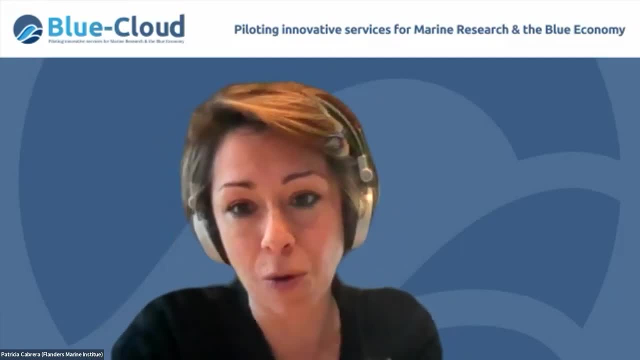 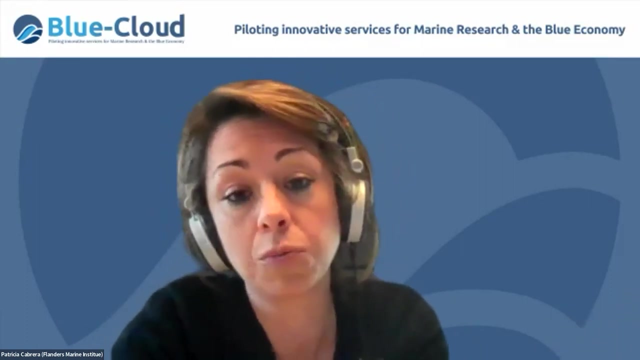 it was a team of it. There was really a wide, diverse profiles joining in the hackathon. So there was a marine scientist, but as well the main components of the group where it that not necessarily knew how, Julia, or how to use Jupiter notebook. 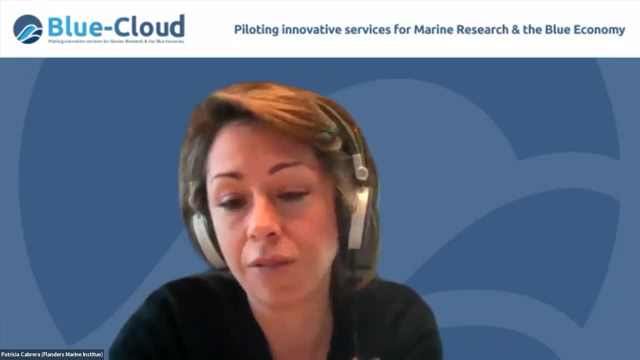 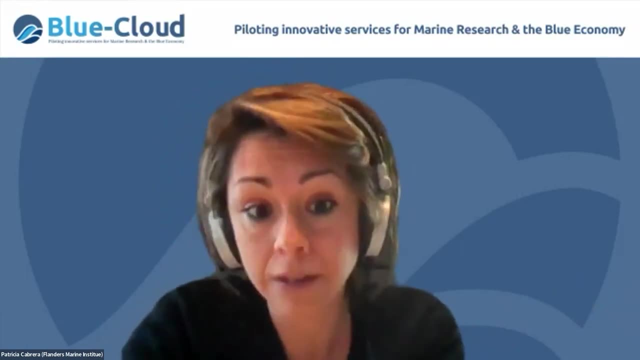 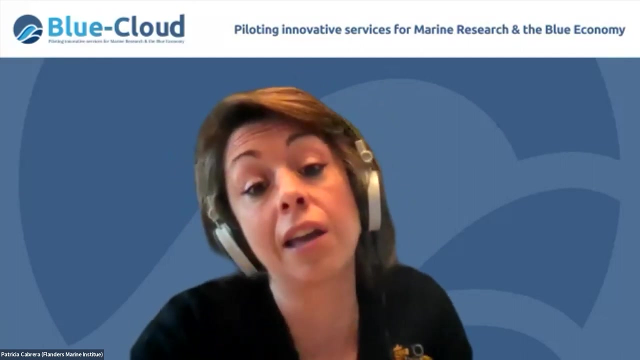 So it was really interesting to see how, in actually even less than three days that lasted today- The hackathon- they were able to really understand run the Jupiter notebooks with other data, not the data. So do changing a little bit of the code and get really interesting results.